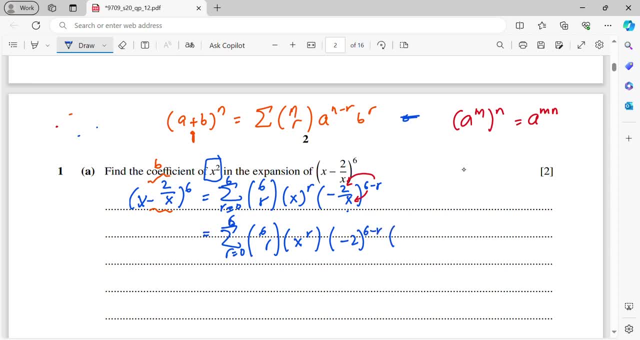 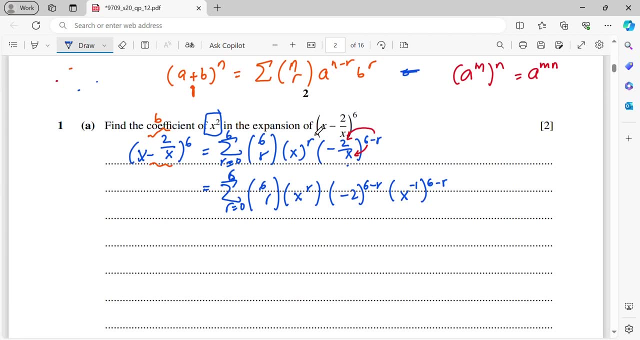 minus 2 to the power 6 minus r, and then this x, I will move up, it will be x power negative 1 to the power 6 minus r. so then from here I will group my x together, because we have another formula, which is a degree m times a degree n. as long as this is same base, you will get a degree. 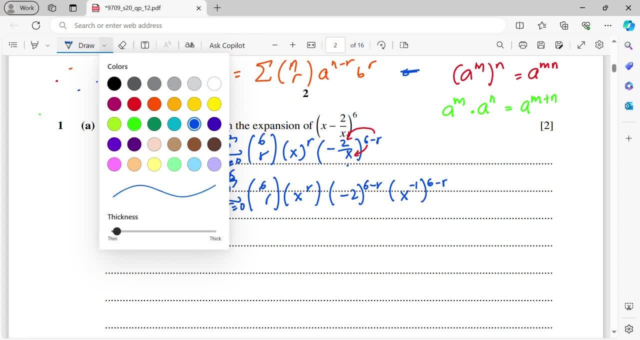 m plus n. okay, that means, now I will just add one more term, or I will just continue with one more step, that is 6cr. then these two x will be combined together. that means it will be x to the power, r plus, and then here you just times in, so I will get minus 6 plus r, together with minus 2 to the. 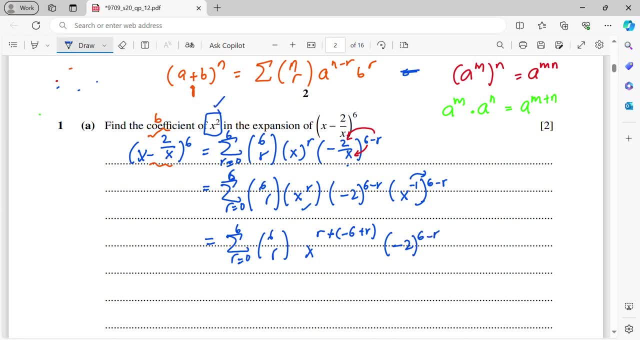 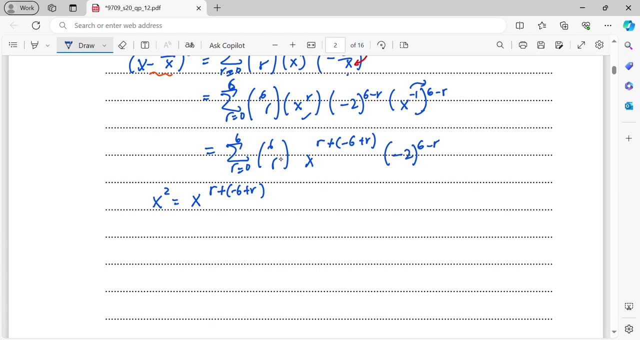 power 6 minus r. okay, so now I will compare with the x squared. so now x squared equals to x, to the power 6 r plus minus 6 plus r. then now, since the x, with I mean both terms with the same base. now I will just compare the index, that will be 2 equals to r plus the times- I mean new times in. 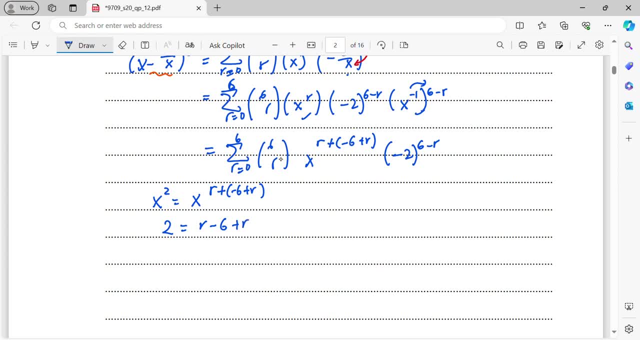 the plus to the brackets, it will be r minus 6 plus r. then I will get 2r equals to 2 plus 6, that is 8. hence my r is 4. okay, so that means the coefficient for x squared have assist when r. 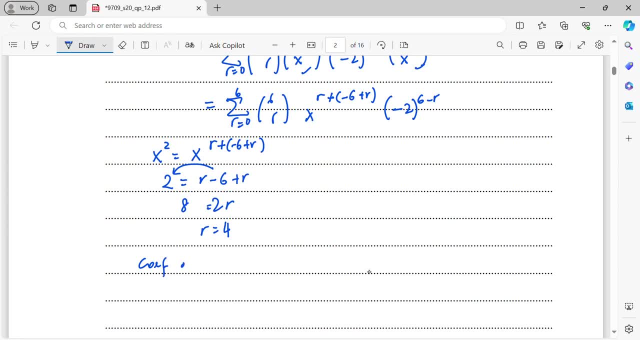 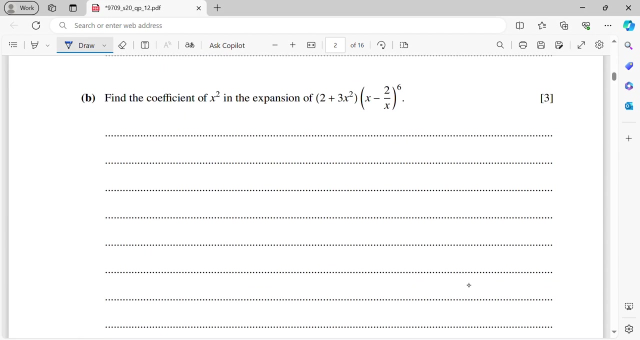 equals to 4. so now I will just write down coefficient for x squared. so just substitute into these two terms: that will be the coefficient for x squared with the calculator are. this is going to be 60, okay, so done for this question. now, plus B, find the coefficient for I squared. 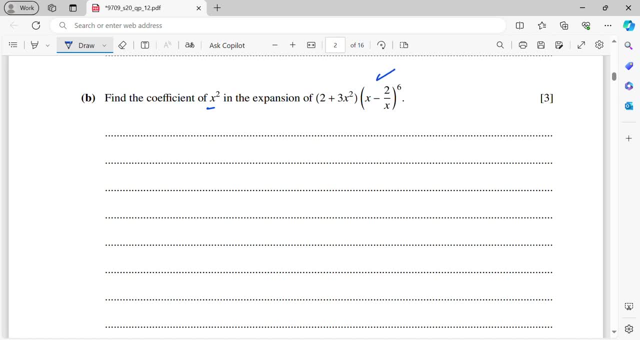 in this expansion. just now we have found the term of X minus 2x to the power 6 right: X minus 2 over X to the power 6. so now I will just add one more. so rewrite the question first, and then here I will change it into: 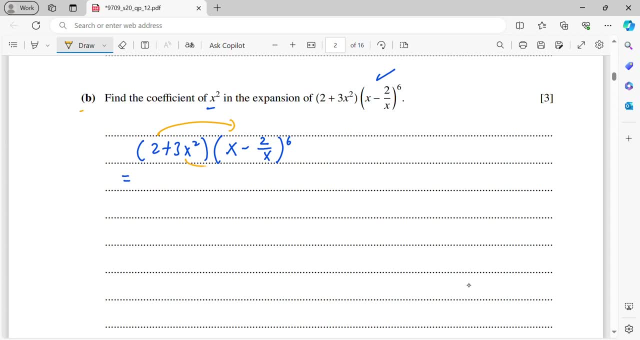 just do expansion, so 2 times the bracket and plus 3x squared times the bracket. so it will be two of the expansion, or two of the terms plus 3x squared of the other term. okay, so for the first one, basically we have found it right, which is here: 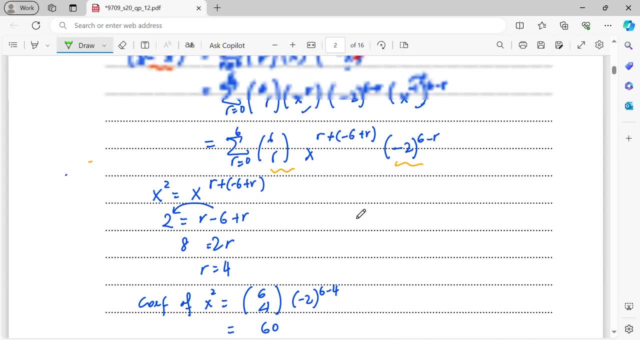 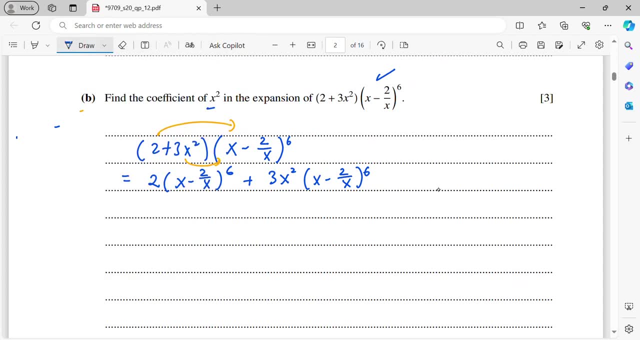 so it means that I just know times two. okay, so I know that the coefficient for x squared is 60.. so which means right here I will just rewrite this- is two times x minus 2x, 2 over x to the power 6.. 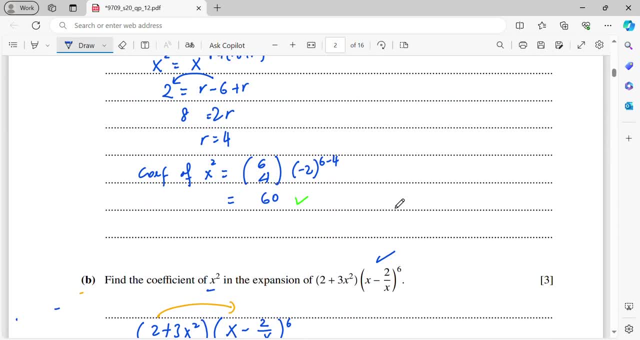 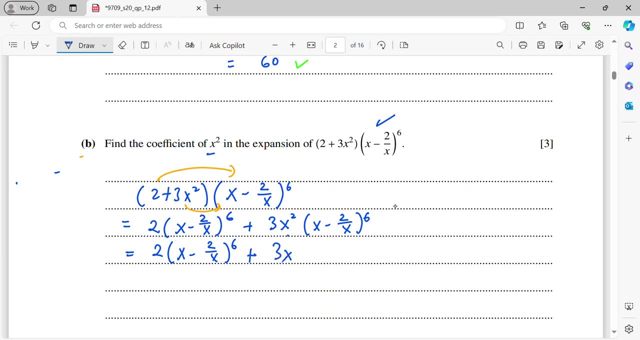 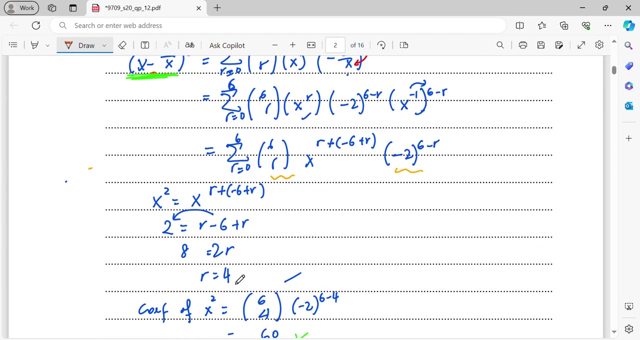 and for the second term, just now we know that our r equals to four. okay, and then now, because of the x squared here, which means I will say my r is basically two, so here the r will be two, because I have another squared outside, so that will be x degree. uh, I mean to get the x degree two right just now. r equals to two, r equals: 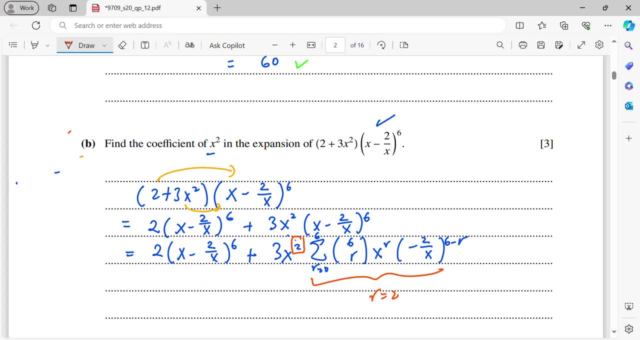 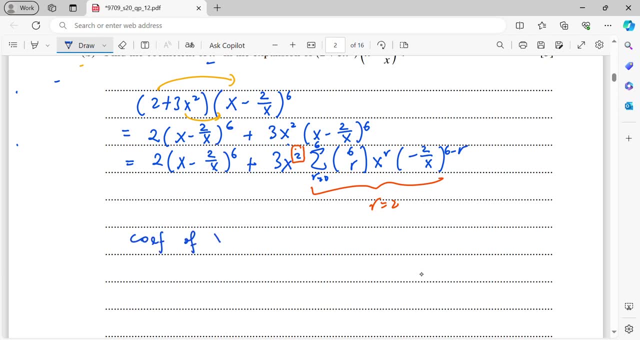 to four. so now I just need r equals to two, because I already have degree two here. that means now my coefficient of x squared, this one. you get it from previous step right, this coefficient of x, what is 60? so you just need to multiply by 2 and plus 3 remains all right. so when r equals 2, 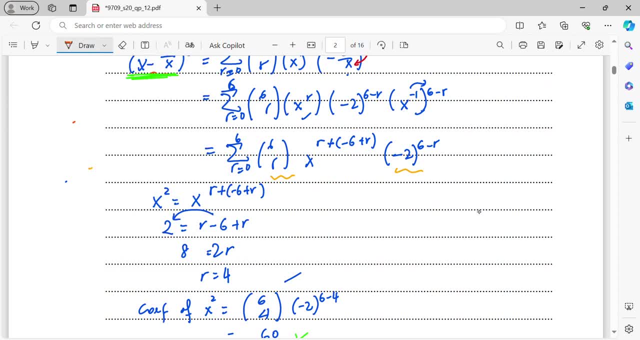 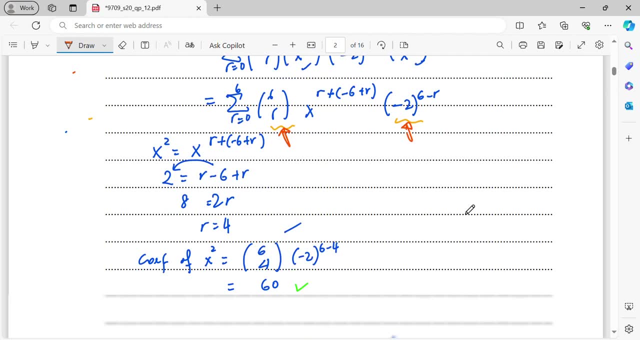 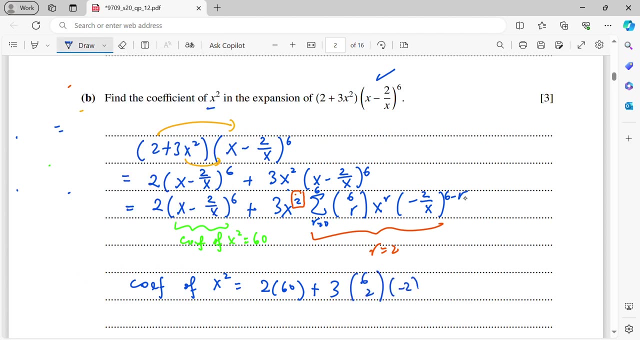 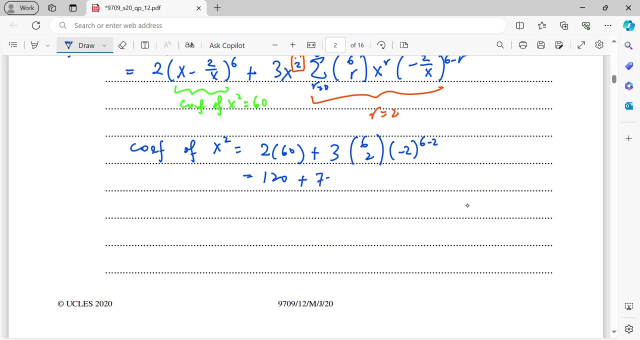 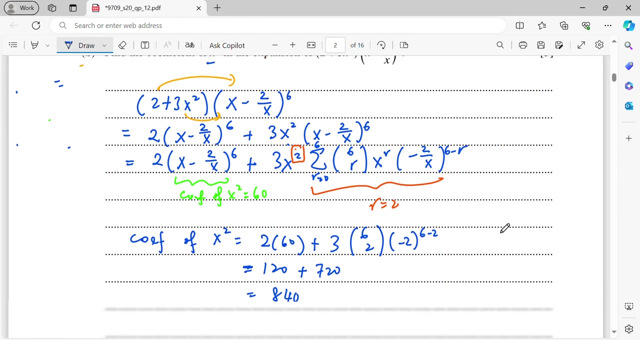 just substitute that into these two terms. just replace. so i will write 62 minus 2 degree, 6 minus 2. so from here you will be getting 120 plus 720, so at last you will be getting 840. so this is how we use the previous part answer to solve this question. 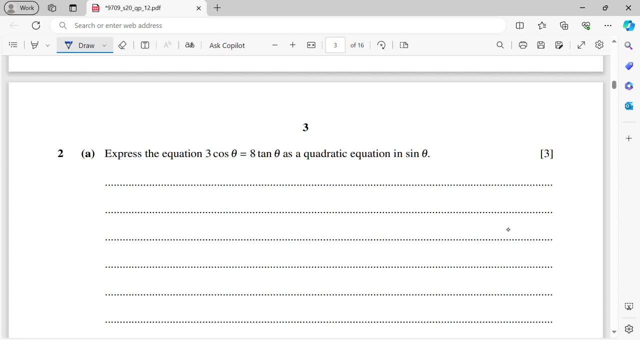 okay, now for question number 2a. express the equation as a quadratic equation in sign data. here we have cos, we have 10 tangent. so now, first of all, i will change the tangent data into sine data over cos data. okay, then, for this cos data. i will move it to the other side. 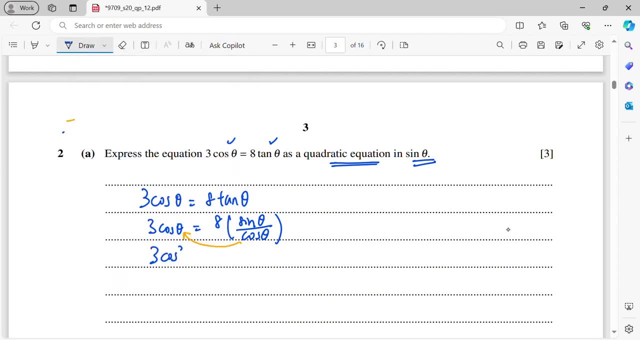 then you will get 3. cos squared data equals to 8 sine squared data. and now to get the answer in sine data means that i need to change my cos squared data into sine squared data. we have a formula over here: sine squared a equals to a plus, cos squared a equals to one. this is the identity, so now we need to keep the sine squared. 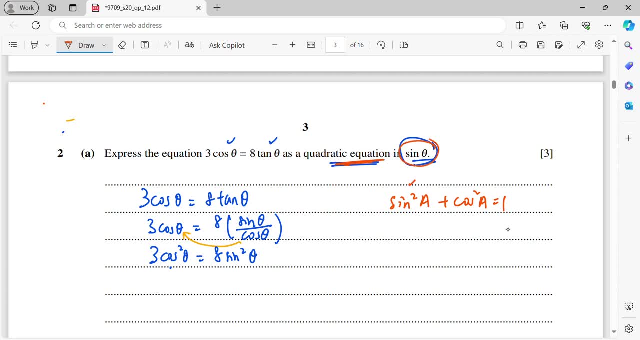 because i need to get the quadratic equation in terms of sine squared or in terms of sine data, which means i need to get the cos squared a as a subject. we need to eliminate it. so this sine squared will be moved to the other side. it will be 1 minus sine. 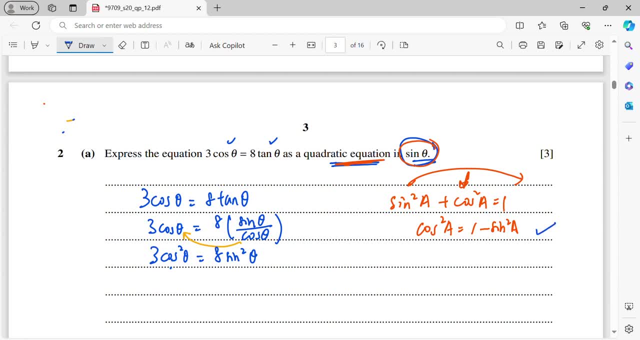 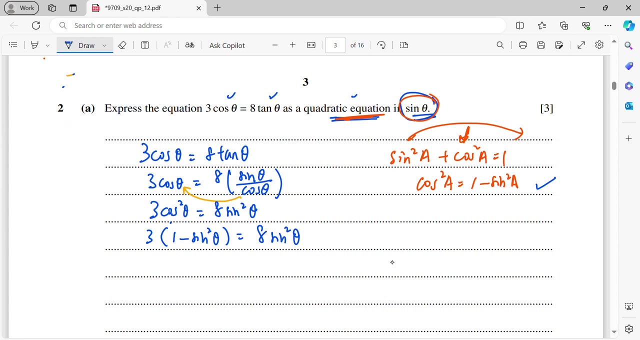 squared a. so now, using this expression, I will get 3 times 1 minus sine squared theta equals to 8 sine squared theta. okay, then from here to get the quadratic equation. so just do expansion. okay, now I made a mistake. this numerator right. when you times in it will be just 8 sine theta. there's no squared, so I shouldn't. 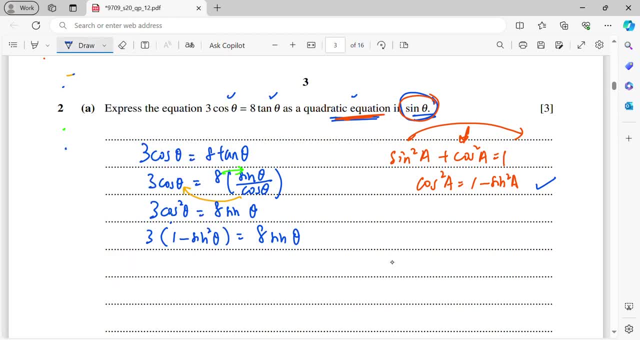 write squared here. so now you just need to write, I mean the, you just need to do expansion. for the left hand side, that will be 3 minus 3 sine squared theta equals to 8 sine theta. okay, and then to get the quadratic equation, I will just 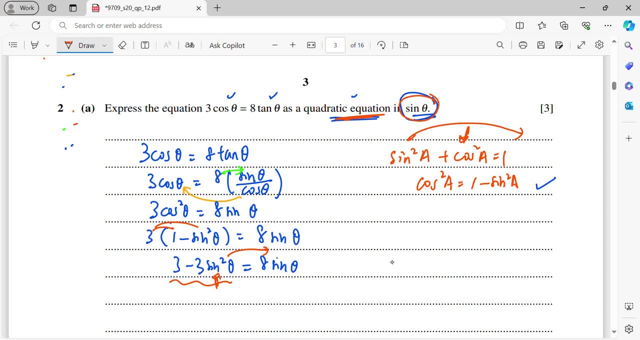 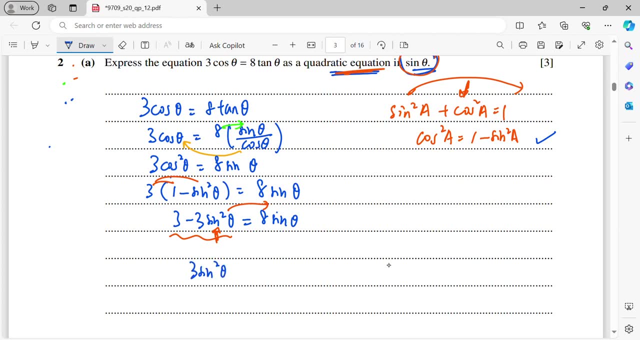 move all the terms to the other side to make it to make the coefficient for sine squared theta as positive value. so therefore you will be getting 3 sine squared theta plus 8 sine theta the 3. you move to the other side because minus 3 equals to 0. so this is the quadratic equation in terms of. 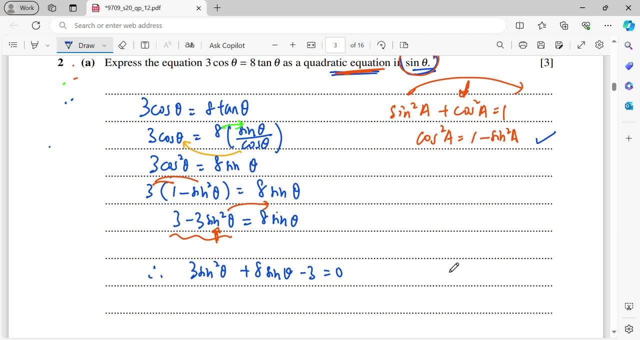 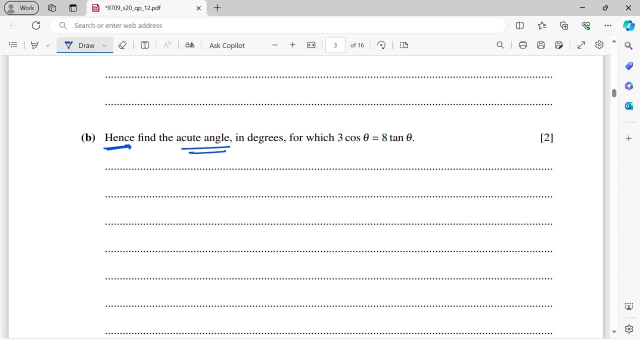 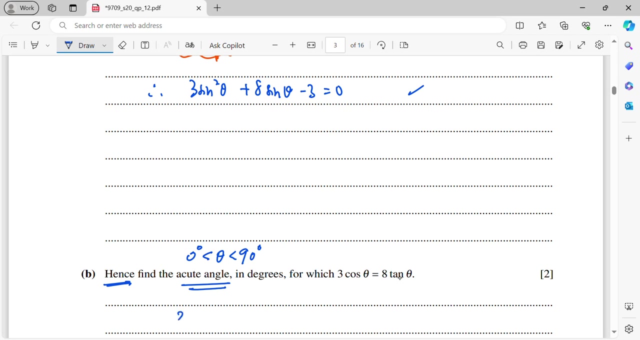 sine theta. okay, now B hence. hence means use the previous answer. find the acute angle. acute angle means the angle in 0 and 90 degrees. okay, for which 3 cos theta equals to 0. it's tangent data. just copy back this quadratic equation so I will get 3 sine. 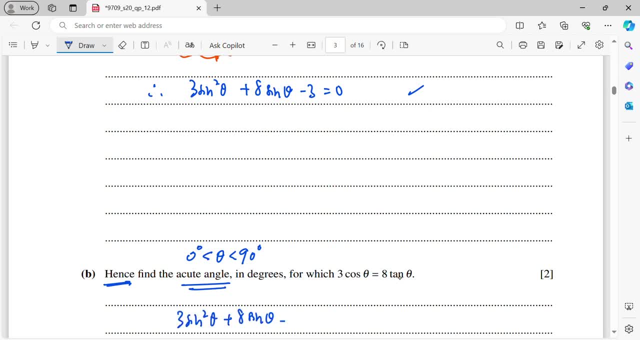 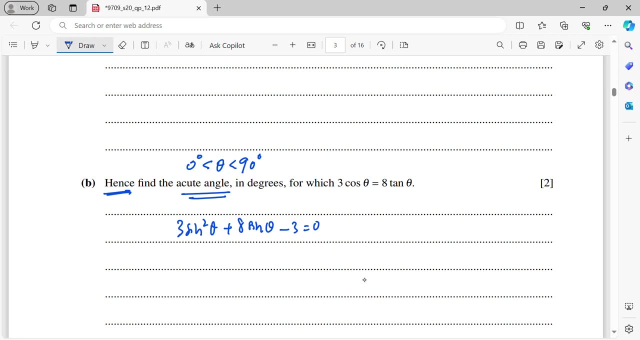 squared theta plus 8. sine theta minus 3 equals to 0. now, when you need to solve this, I can just factorize this into 2 linear factors. that will be sine theta minus 3 times sine theta minus 1. multiplied with sine theta plus 3 equals. 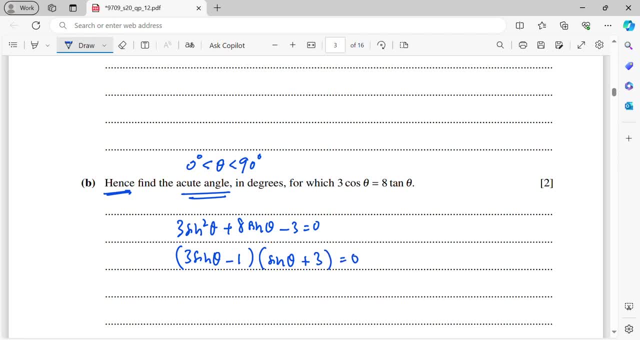 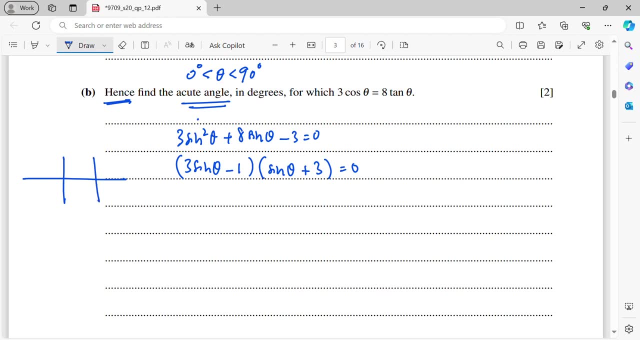 to 0. so this factorization can be done using these two factors in order to get the done using calculator or just a manual factorization. okay, if manual factorization is like this: to get three sine squared data- it will be three sine data, times sine data, and then to get the three. here it. 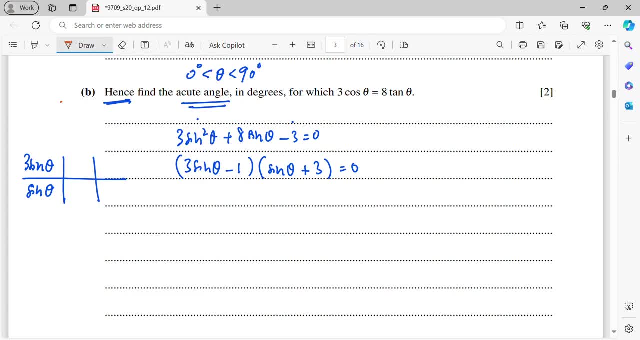 can be three times one, but then where to put my three? it can be the top or the bottom. let's look at here: plus times. minus is a minus. therefore, in order to get plus eight sine data later on, i should put my three over here. this is my plus three, because when you multiply it will be nine. 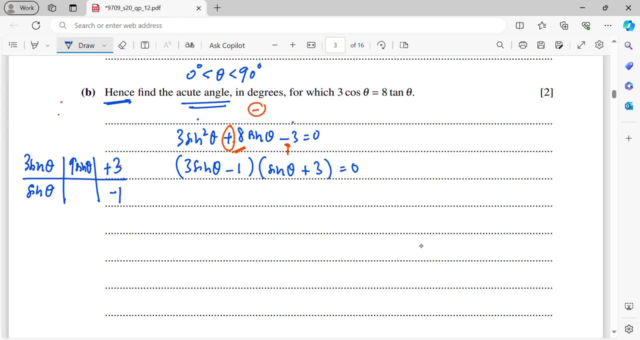 sine data. okay, then this is minus one to get plus and minus. so minus one times sine data, that will be minus sine data. then at last, right, this is going to be three sine squared data. when you multiply first column and multiply third column it will be minus three, but the second column you. 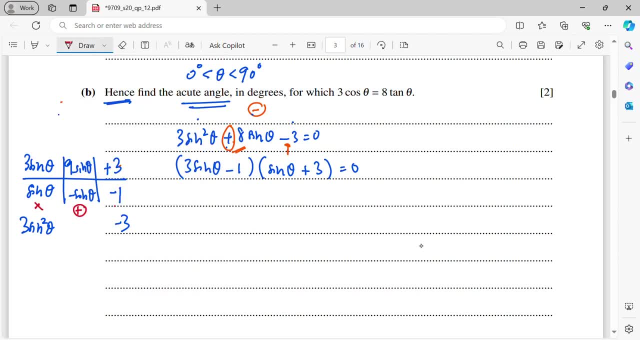 got the plus. okay, you got a plus this one times. so when you plus, that will be nine sine data minus one side data, that is plus eight sine data. so this is how i get the factorization, but final answer for the factors will be cross multiplication. okay, this is how i get these two factors. if you do it manually, then 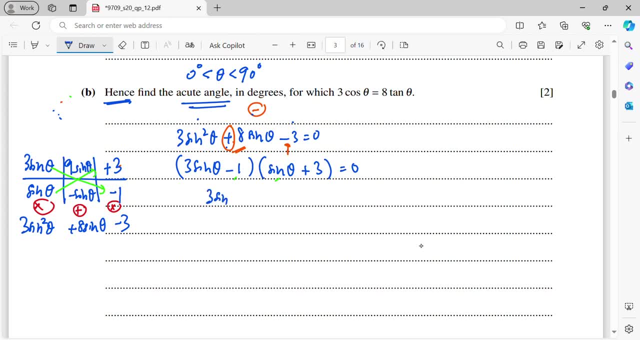 now, multiplication of two terms equals to zero means one of them must be zero. i will let either the first and the second be equal to zero, and the second be equal to zero and the third be equal to zero. the first term equals to this equals to zero, or the second term equals to zero. but then when you 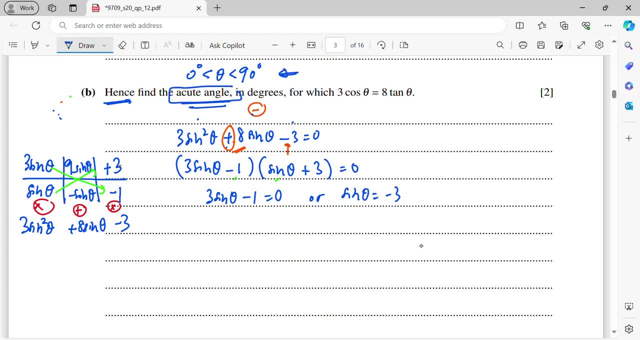 look at here. a cubed angle means your angle is between zero and 90 degrees. but we know that for any data sine theta minimum is minus one. it cannot be minus three. so that means undefined for the second form. okay, there's no solution for this second form, so now i just need to solve 3 sin theta minus one, equal to: 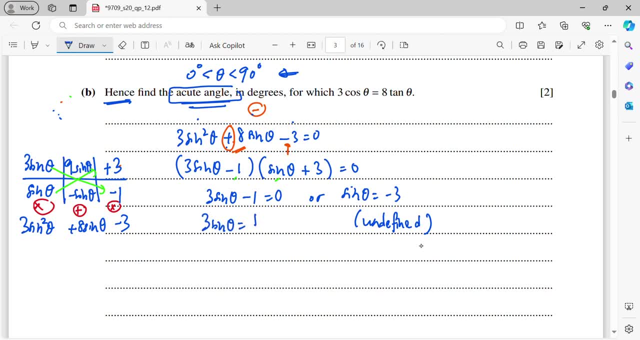 zero, which means my three sine data equals one. so sine data is one over three. so then it is in the first quadrant because of a cube's angle. so when you take inverse sine of one over three, make sure your calculator is in degrees mode or the default mode. it will be 19.5 degrees. so this is your. 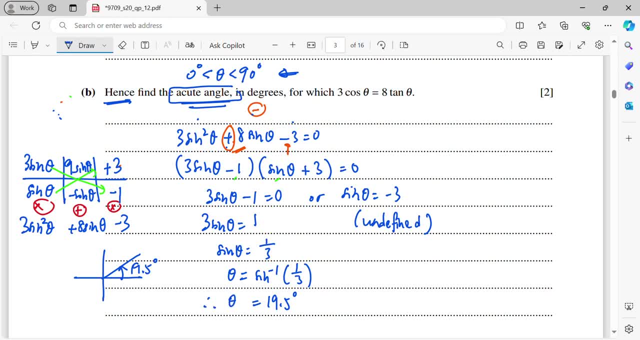 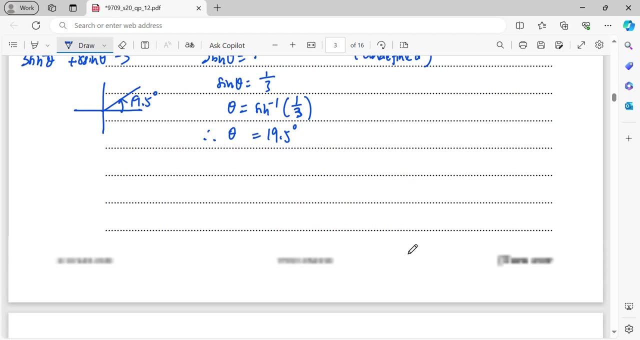 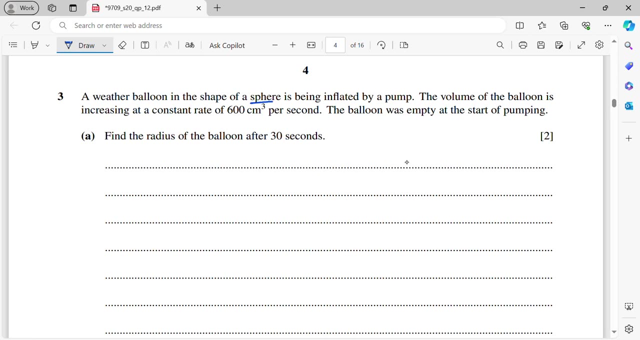 solution: okay, now next question, number three. a weather balloon is a weather balloon in the shape of sphere is being inflated by a pump. the volume of the balloon is increasing at a constant rate of 600 centimeter cube per second. so volume is v. whenever you see the rate, that is d over dt. therefore, we'll combine this whole information that is dv over. 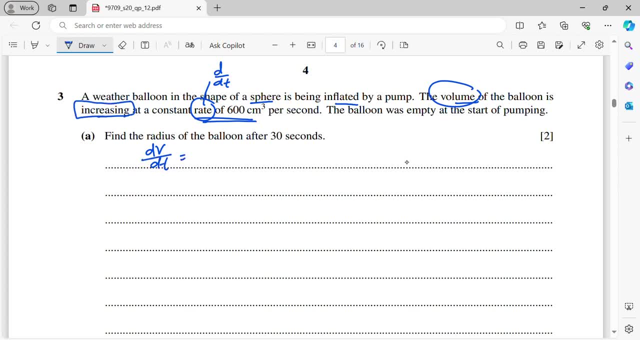 dt, and this word is very important. the increasing means this 600 is a positive value. okay, if this is decreasing, then you have to times a minus, so i will write 600 now. the balloon was empty at the start of the pumping. means that t equals to zero, right, the volume is zero. 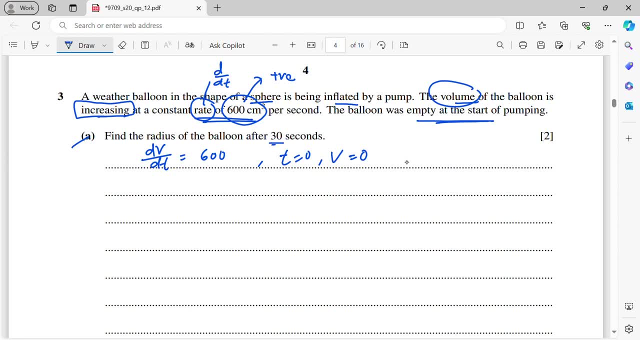 now a. find the radius of the balloon after 30 seconds. so what is the r? okay, what is the r when t equals to 30.. okay, so from here? all right, we know that volume of sphere is 4 over 3 pi r cube. all right, so for this question, 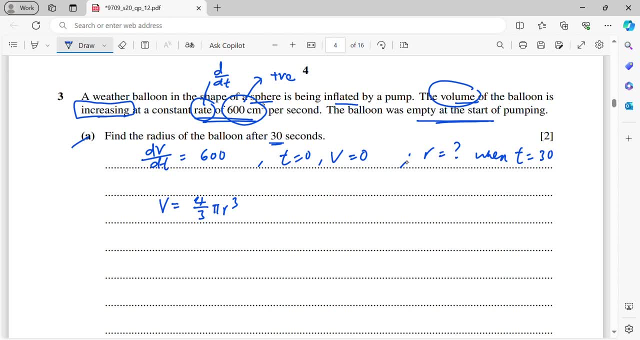 from here. okay, i need to find out what is the volume after 30 seconds, right? so look at here: per second is 600. this is centimeter cube per second. so i will say: one second is 600 centimeter cube. this is the volume. so when 30 seconds, 30 seconds, okay, t equals to 30. so now my volume: it will be 600. 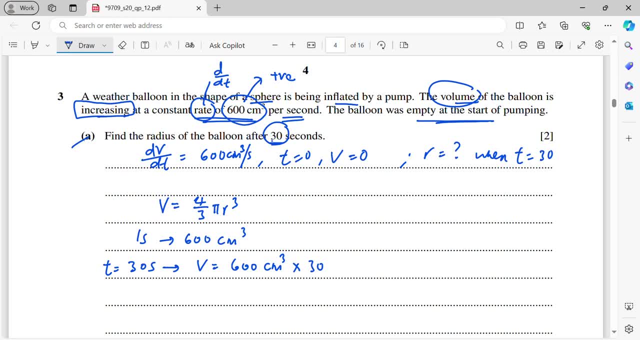 centimeter cube times 30, right, which means you will be getting 18 000 centimeter cube. so this is my volume when t equals to 30.. right, so now the question asks for radius. so i have found the v. okay, the r is unknown. therefore i can just substitute into this formula: right v, down, v is found. 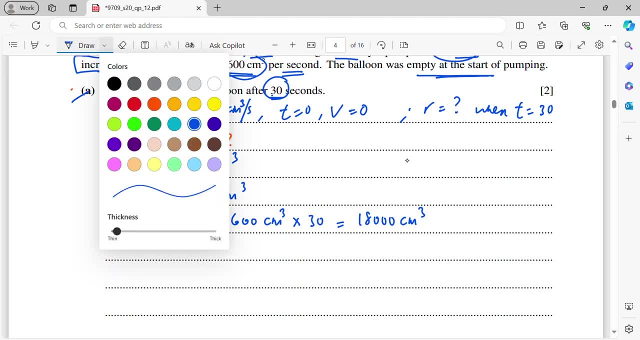 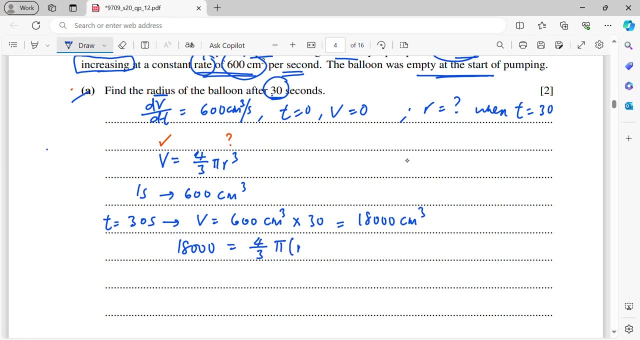 r is unknown, so i will just write my 18 000 equals to 4 over 3 pi r cube. so to get the r, this 4 over 3 pi will be moved to the other side. okay, so now it becomes r cube equals to 18 000 times. this is 4 pi over 3 on the left side, on. 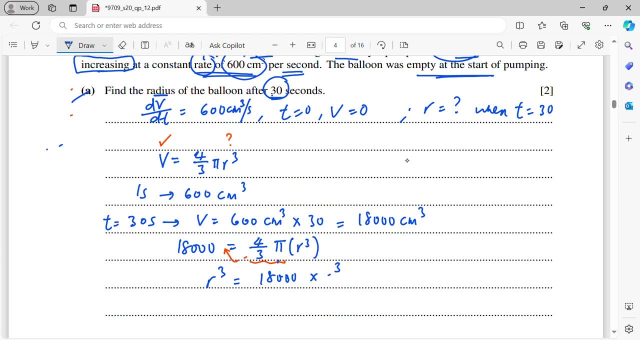 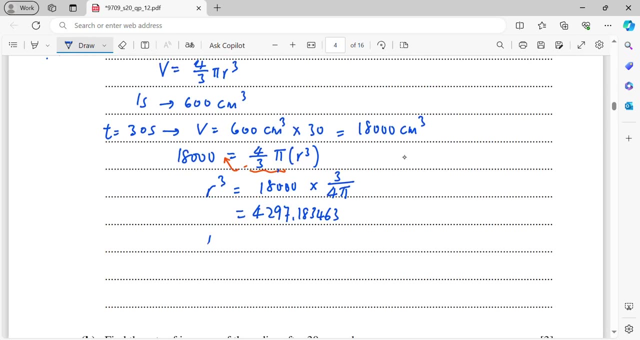 the right side 4 power 3. so when you move it to the other side it becomes 3 over 4 pi, because it's divided. so then from here i will be getting four, nine, seven point one, eight, three, four, six, three. i give more decimal places now. my r will be the cube root of this value. so cube root. 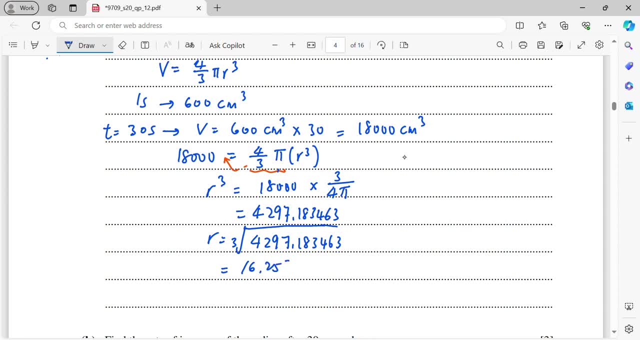 then you will be getting 16.2578, and now my r round up to three significant figures. that's really great �'s okay. so the next l is their plus and minus will be. the next one is 4 and the 검은 permitted. let's me now write the value: Saint 1. the offset of 16 seeds can carry up to 36. suddenом is equal to 16 points, 0 and 0.. gap from 7 ways format and double order forth and cross over 0 goes outdan. so from e1 to false, from e2 and drink it up and lost your number in the empty music. 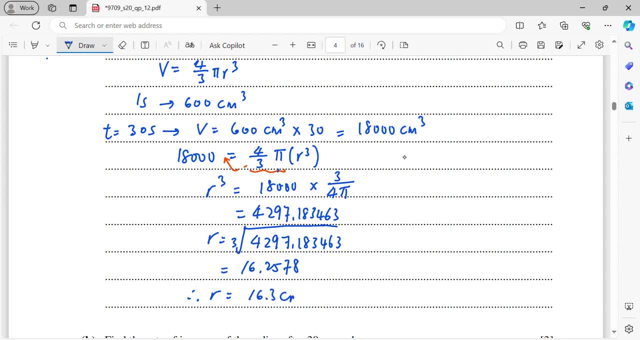 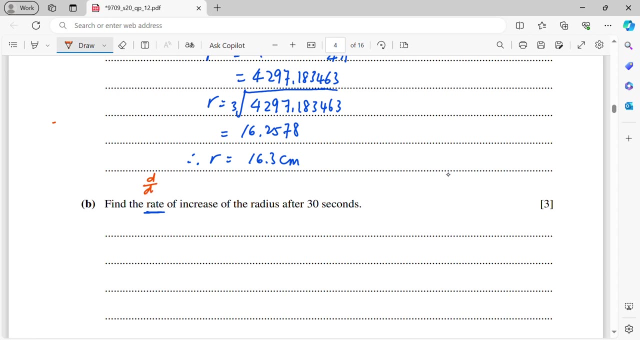 up to three significant figures, that is, 16.3 centimeters. so this is the solution of this question. now we find the rate rate is d over dt of increase. that means it's a positive of the r. so what is dr dt? make sure it is a positive value because of increase after 30 seconds. 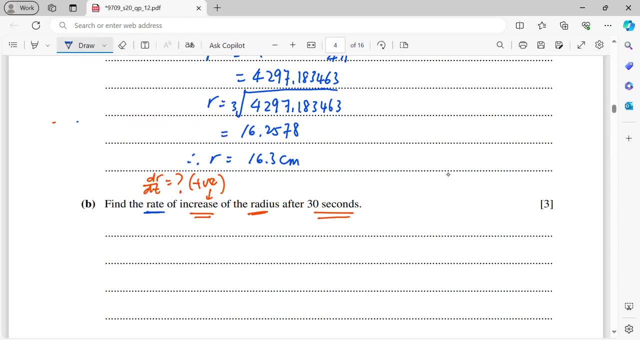 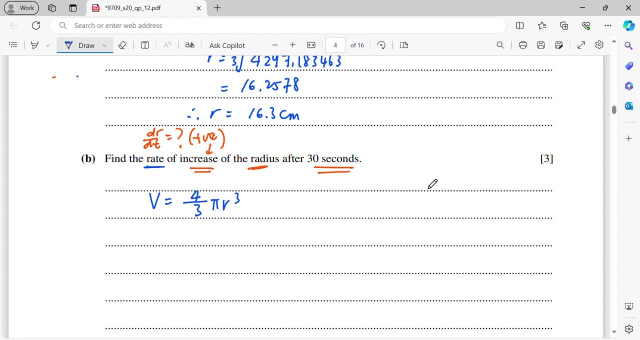 right. t equals to 30.. so now you need to find dr, dt. so means that we need to use the course, the chain rule. okay, we need to use chain rule. so from here your dv, dr, to differentiate right, let's say differentiate constant times, x, degree n. so you take out the 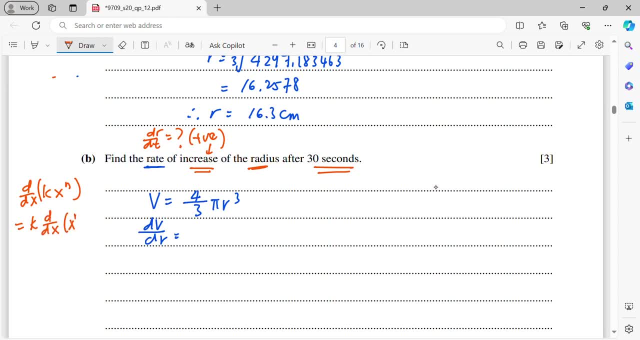 constant, or you factorize the constants and differentiate x degree n. so when you differentiate x degree and you basically basically move down, the n remain the x and degree need to needs to be minus 1. after that you differentiate, the x is 1. okay, this is the formula, which means you get 4 over 3 pi. that is a constant. 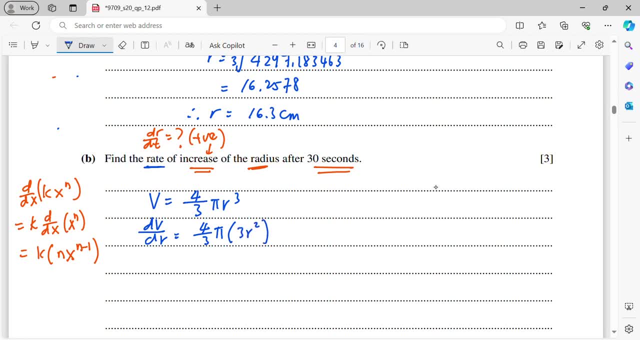 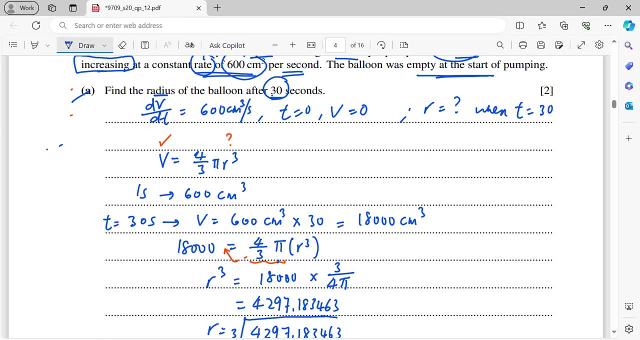 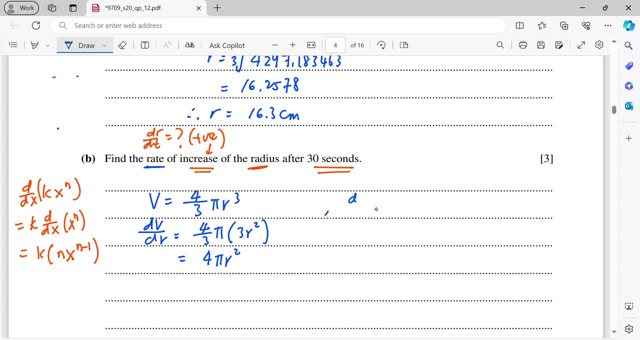 differentiate r cube is 3 r squared, then at last this will be 4 pi r squared. okay, and now, just now you were given dv dt is 600. so here i will write down: dv dt is 600 positive. and now you need to find what is your dr dt. 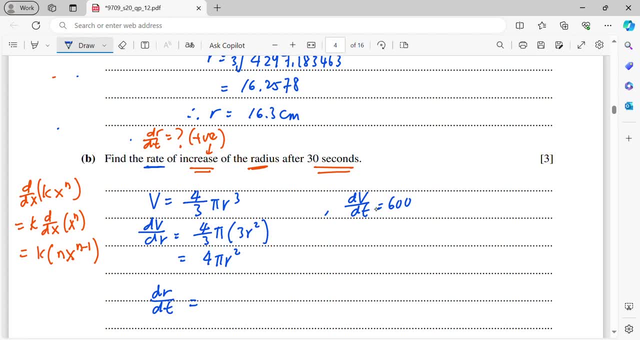 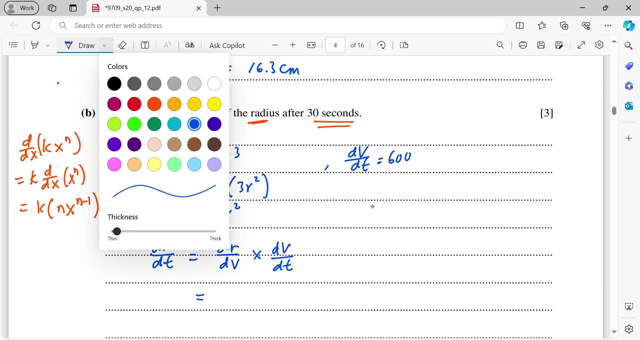 so i will write dr over dt. i need the r in the numerator, so i must write dv dr here first. so it will be dr over dv times dv over dt. which means now, for your information, dr over dv equals to 1 over dv over dr. that means now i will take 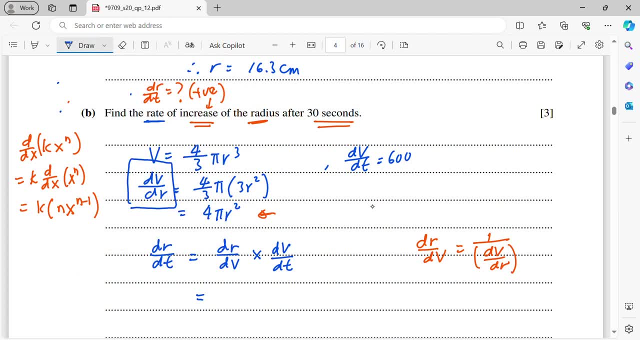 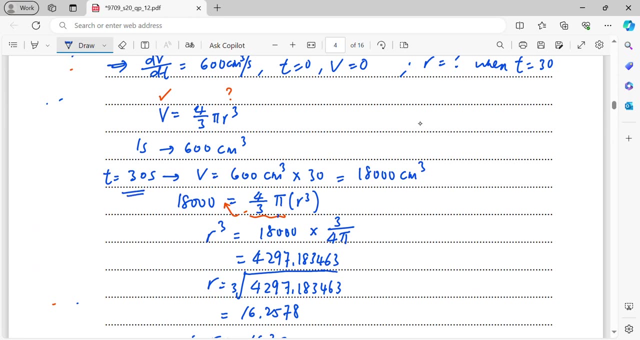 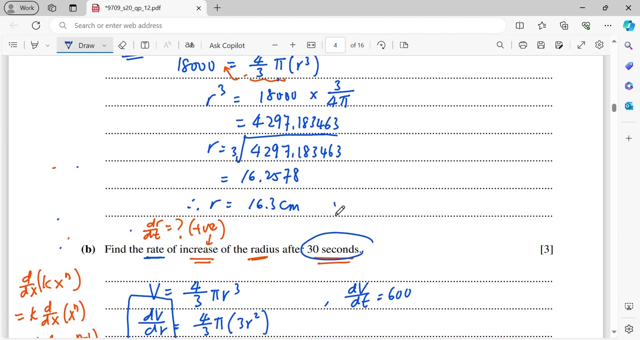 1 over this value. so that is going to be 1 over 4 pi r squared multiplied with 600. okay, and now we know that after 30 seconds, right here here, you are r. so after 30 seconds, your r is found 16.3. so now here, i will just replace the value by 16.3. 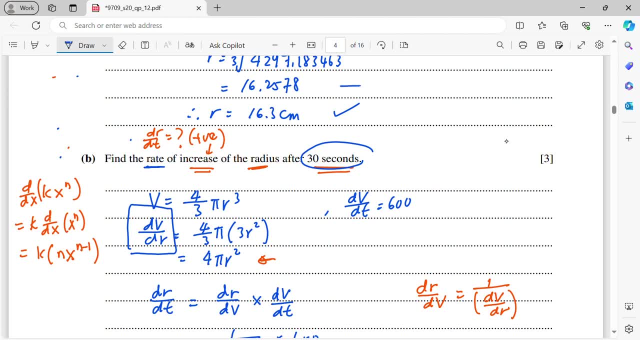 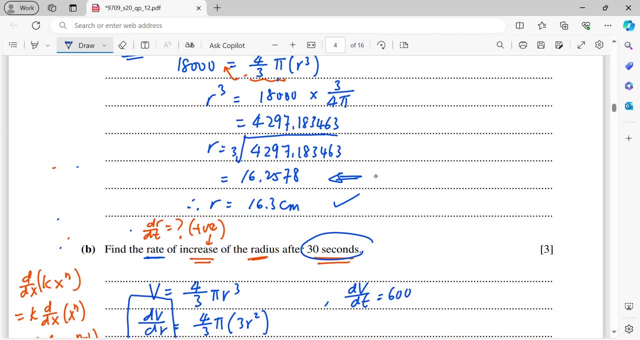 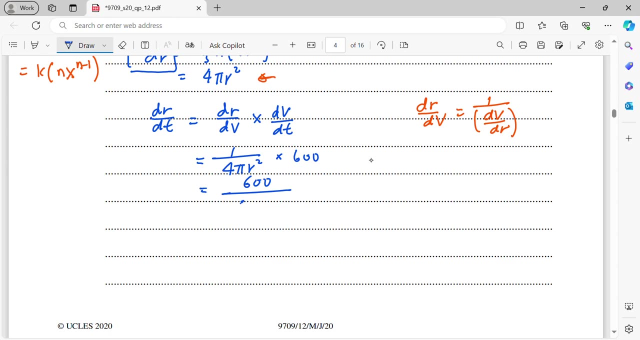 but then for the actual, for the accurate calculation, i will refer to the previous value, which is more decimal places or more significant figures. so i will be using 16.2578 for the calculation. so here is going to be 600 over 4 pi times 16 point 2578. 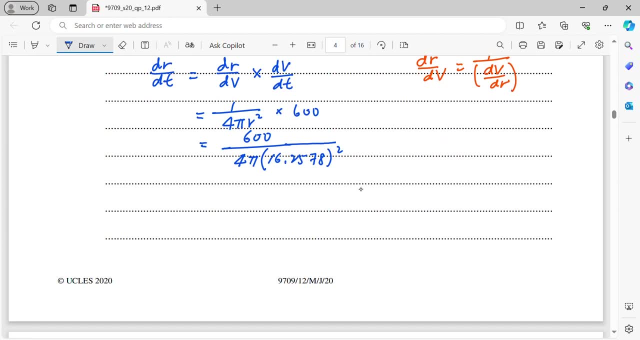 times 16.2578, then split, so then from here you will be getting 0.1806. and now, if i round up to three significant figures, look at the fourth significant figures, it is more than five. therefore you round up so i will get 0 point one. eight one there are is centimeter, and that's also uh r double. 36.38 ct, so it's equal to three, and then in terms of 3 r, now, if you were to such that ms 0.5, then saving it to c, there is cenahma, which is prepare the money, money, money희. 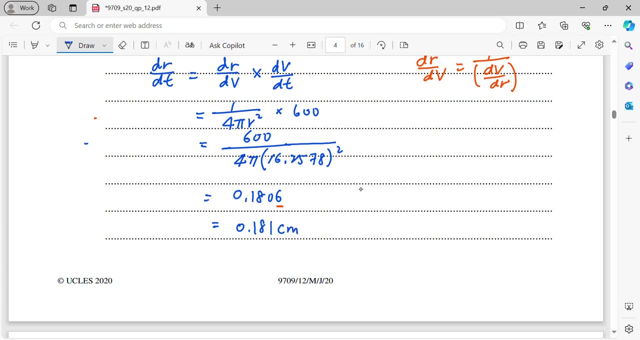 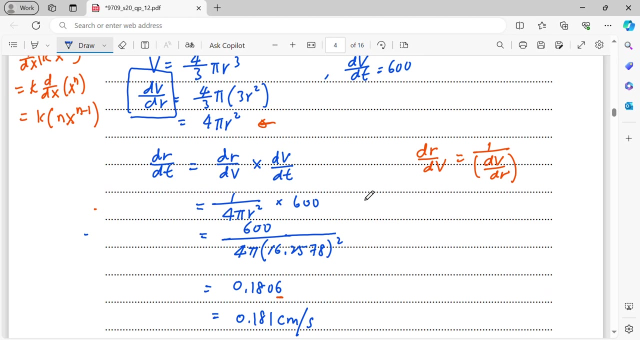 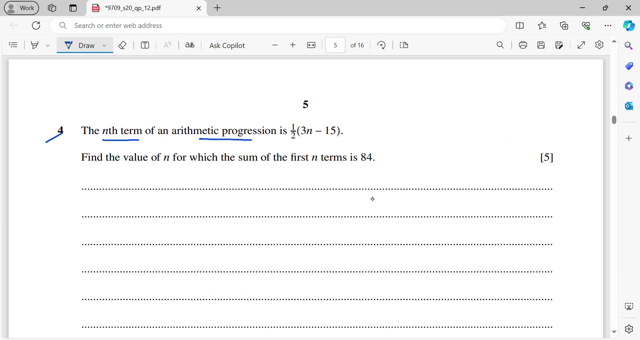 the r is centimeter, and then time is second, so it becomes dr. dt is 0.181 centimeter per second, so that is the rate of increase of radius. okay, next question number four. the nth term of an arithmetic progression is this expression. so i will write down first ap arithmetic progression: tn is half of 3n minus 15. 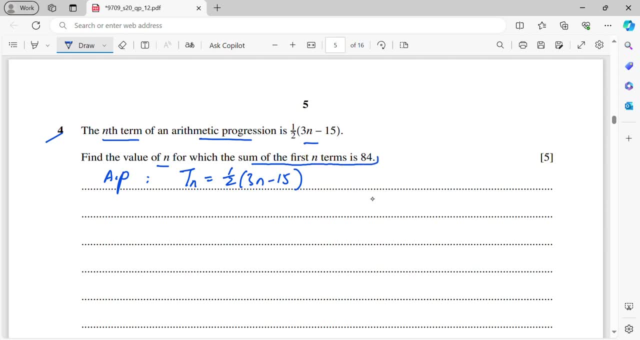 find the n, for which the sum of the first n terms is ad4. okay, so for arithmetic progression, sum of the first n terms is basically as: n equals to n over 2, 2a plus n minus 1, d. that means now i need to find out what is my first term, a, and the common difference d. 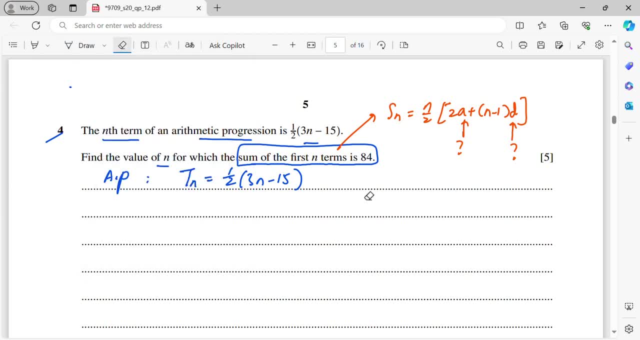 so first term is same as t1. all right, so a equals to t1. i just need to replace my n by one. that is half of three times one minus fifteen. then this is going to be half of three minus fifteen. i get negative twelve, and that is negative six. now, before you get the d, this d is basically: 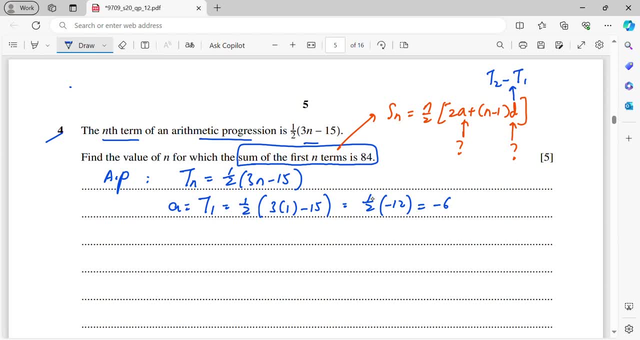 second term minus first term. so i need to find out what is my second term. so t2 is half of 3 times 2 minus 15. that is half of 6 minus 15. that is minus 9. then I will get minus 9 over 2. 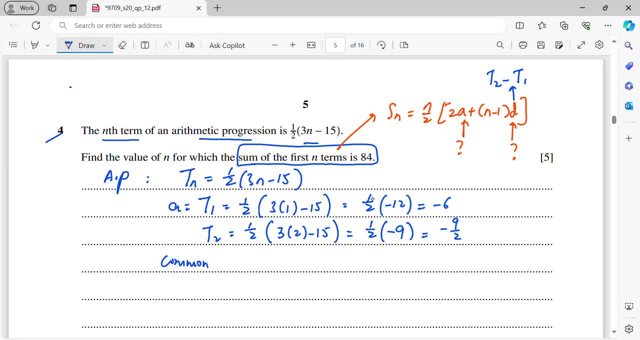 now my common difference d equals to t2 minus t1, that is, minus 9 over 2 minus minus 6, and this is going to be 3 over 2. all right, so now Sn equals to n over 2 times 2a plus n minus 1d. this is the. 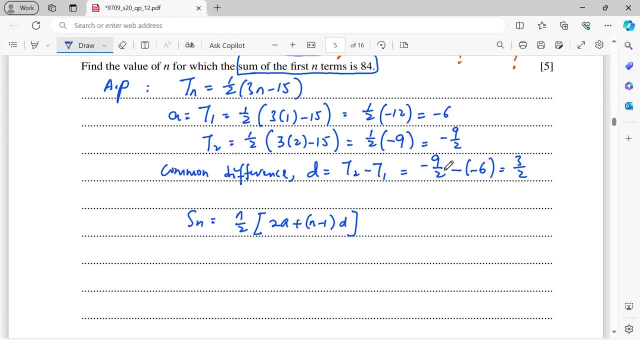 definition for the sum of first n terms for arithmetic progression. and now it's given that it is ad4, so I will replace the Sn by ad4 and then keep the n and replace the a and the d. so I'll get 2 times minus 6 plus n, minus 1 times 3 over 2. okay, so from here, since I have the denominator of 2, 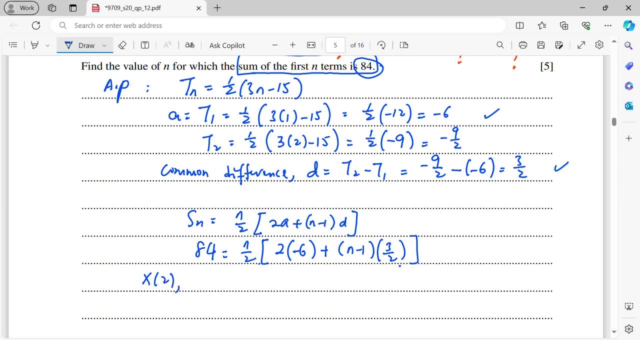 here means that I times the whole equation by 2 first. so left hand side: 84 times 2, you will be getting 3, 168, okay, 168. then now these two will be cancelled off because you times 2. then now here just expand and do expansion, so I will be getting n bracket minus 12, then the 3 times. 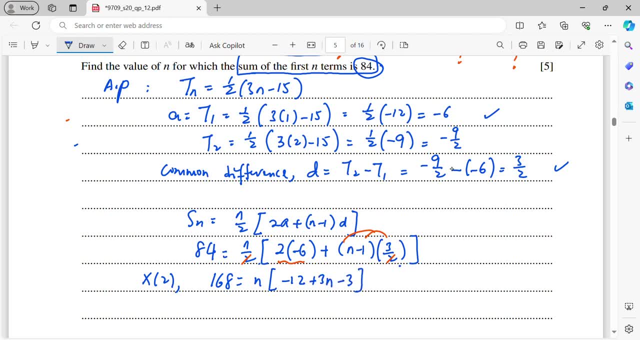 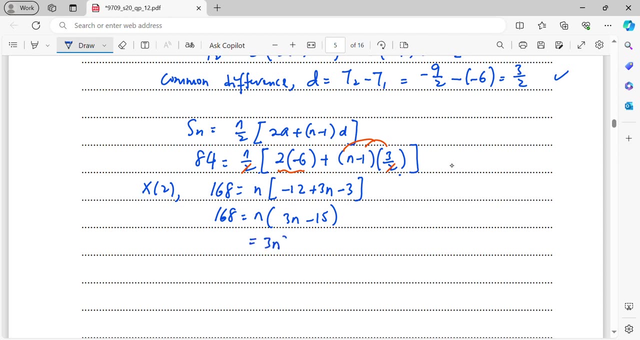 n is 3n 3 times minus 1, I get negative 3. so then from here 168 equals to n times 3n minus 15. okay, then you can just multiply, so here I will get 3n square minus 15n. 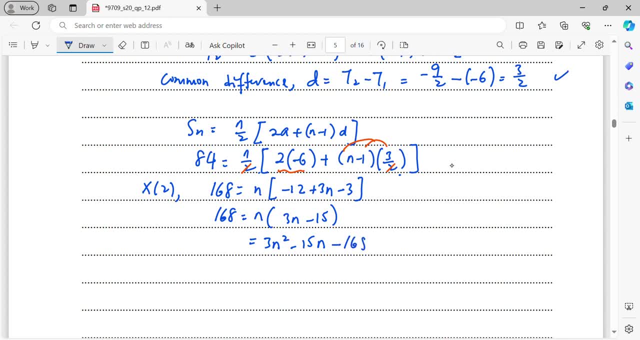 the 16, 168 move to the other side. negative 168 equals to 0,. so this whole equation can be divided by 3, I will get 0 equals to n square minus 5n. okay, wait, all right, I overlook this. 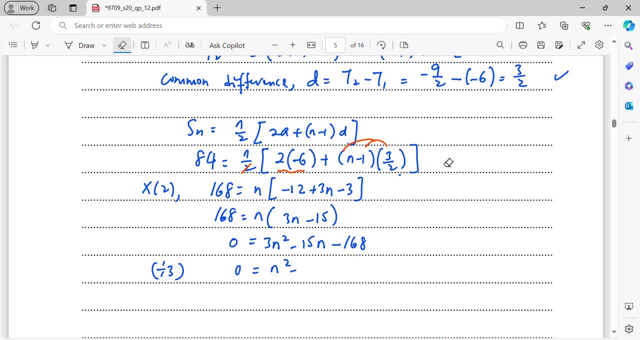 okay, wait, here I times by 2, right, so this was supposed to be wait. there's a mistake over here, because I times by 2,. basically this: when you times by 2, the 2 and half cancel off, okay, but then you still have another half outside. that means: 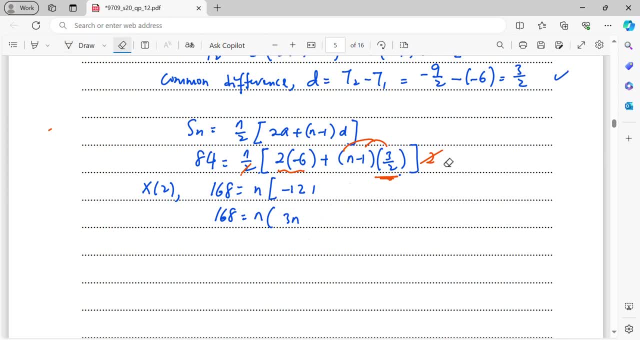 basically I need to times by 4, okay, so never mind, I leave it in this form first. then here I will be, getting plus 3 over 2n, minus 3 over 2, okay, there are times another 2,. 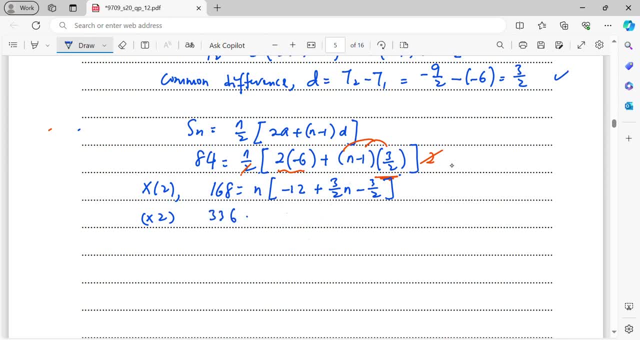 so here becomes 3, 3, 6, then 2n. after that here will be okay, probably I just times 4 directly. okay, that's it, that will be better. okay, my working becomes this: this 2,. I move out, so it will be 1 over n over 4,. 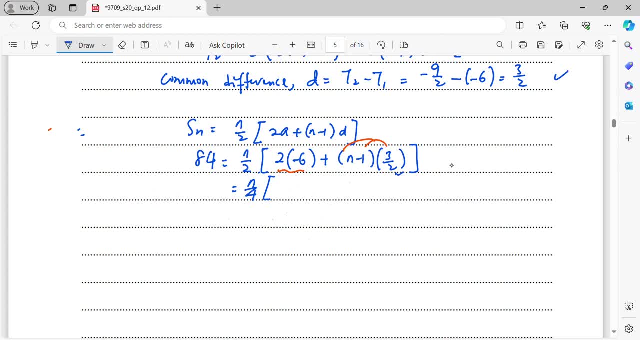 so when you factorize another half from the brackets means that first term here got to times another 2, so 6 times 2, then times another 2 will be negative 24,. okay, so since I have factorized this over 2, that means just left 3 times n minus 1,. 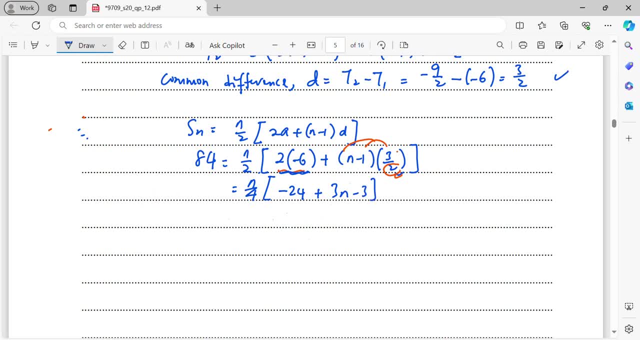 then I will get 3n minus 3,- this one is better. then it will be n over 4,, so 3n minus 27,. then now I times the whole equation by 4, so 84 times 4, you will get 3,, 3,, 6, okay, so. 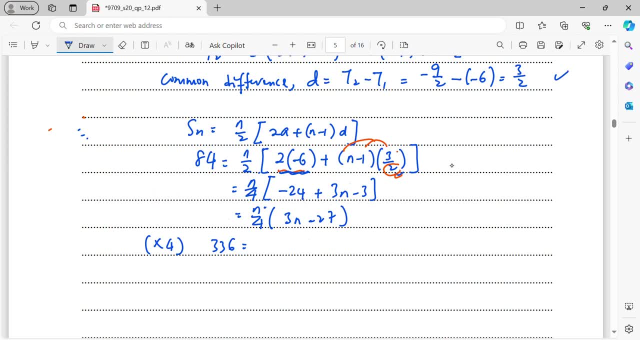 for the right side. when you times 4, the over 4 is cancel off. left the n, so I will multiply in. it will be 3n square minus 27n. okay, and now, since your 3n square is positive, 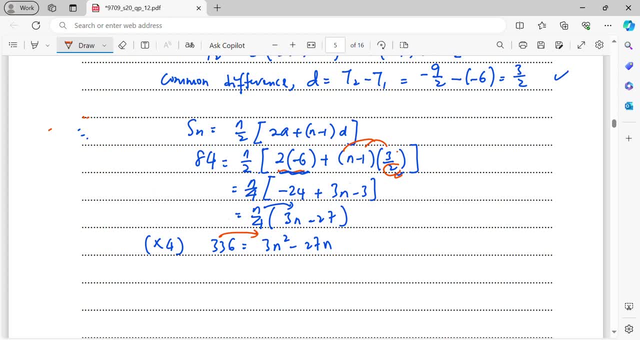 on the right side means that I will move this 3, 3, 6 to the right side to get the quadratic equation. that means you will be getting 3n square minus 27n minus 3, 3, 6 equals to 0,. 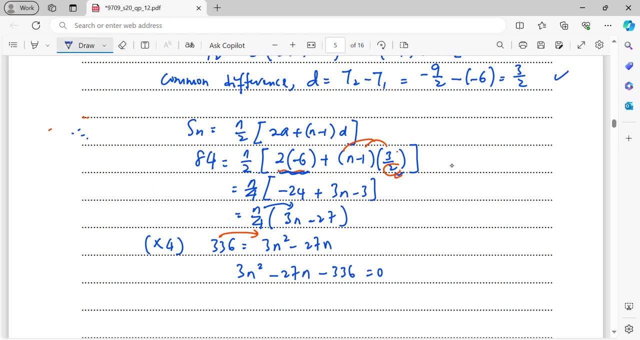 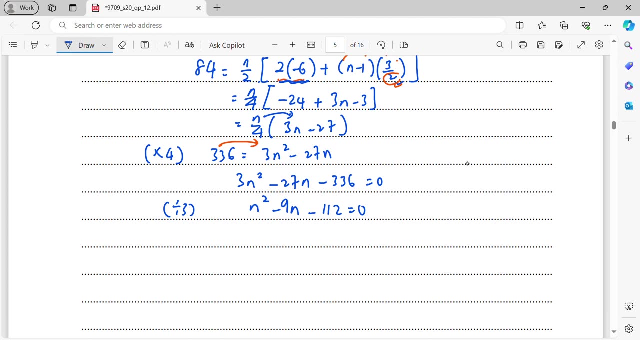 and now here I will divide the whole equation by 3, then you will get n square minus 9n minus 1, 1, 2 equals to 0, okay, and again factorize the quadratic equation, then you will be getting n minus 16, after that, n plus 7 equals to 0,. 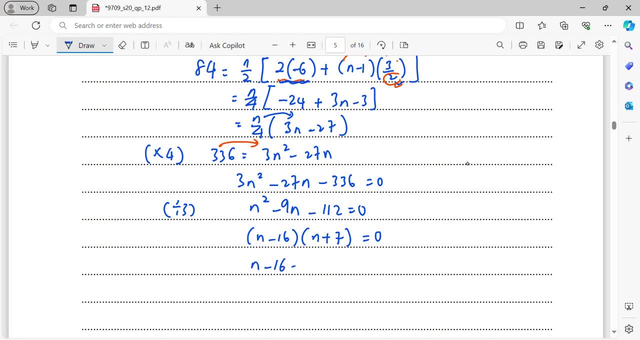 so one of them must be 0, so n minus 16 equals to 0, or n plus 7 equals to 0, so when you consider the first one equals to 0, your n is going to be 16 and the second one is. 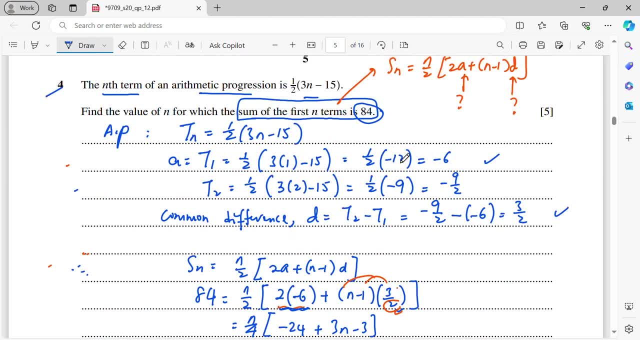 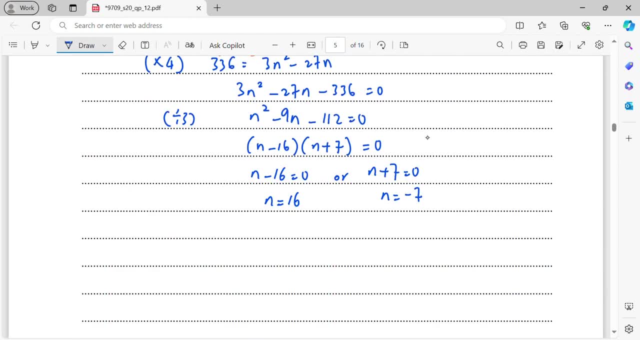 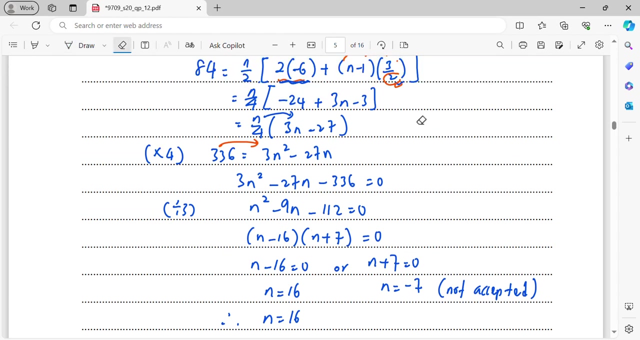 going to be negative 7,. now, when you look at the question, the n is the n terms, so which means cannot be negative, right? so that means this is not accepted because your n is the number of terms. therefore, the answer is 16, so that's the solution of this. 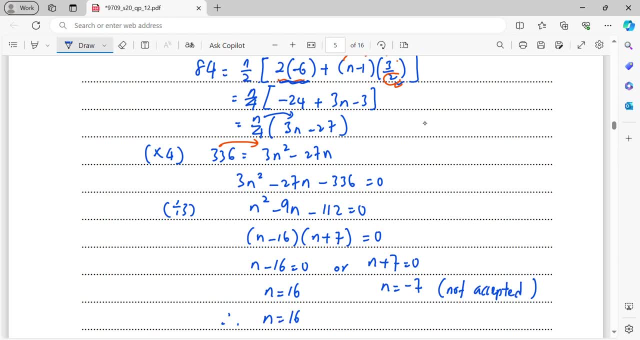 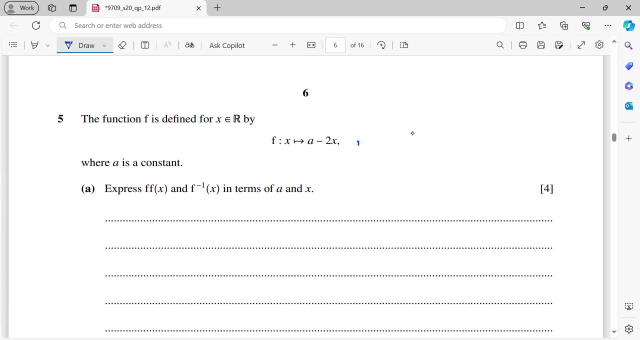 question okay. next question, number five: given this fx where a is constant, express, f fx and f inverse. okay, so this f fx is basically the composite function. so now i will write f fx. okay, firstly, i will write down my fx first. my fx is basically a minus 2x. so here is f of a minus 2x. 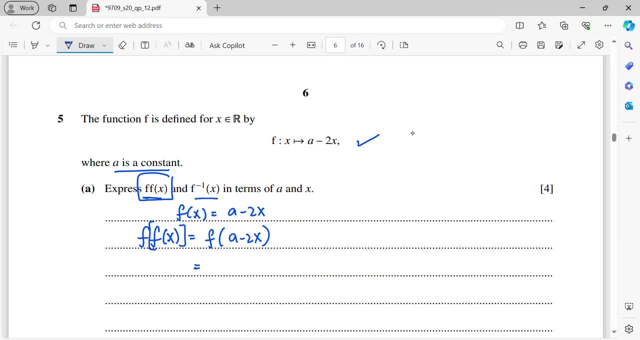 okay. so now what to do here is you just need to change this x to a minus 2x, so change all the x here, which means i will be getting a minus 2 of my new x. so then here, when you do expansion- right, do expansion over here- i will be getting a minus 2 times a minus 2a. 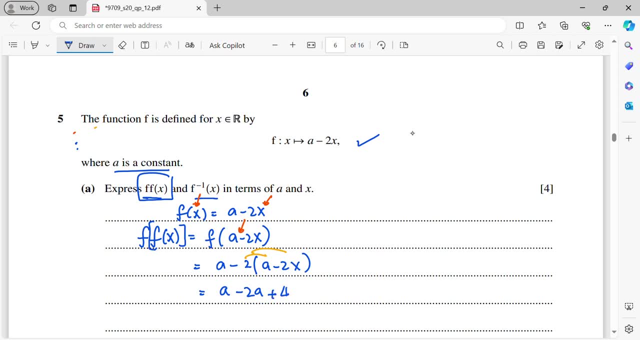 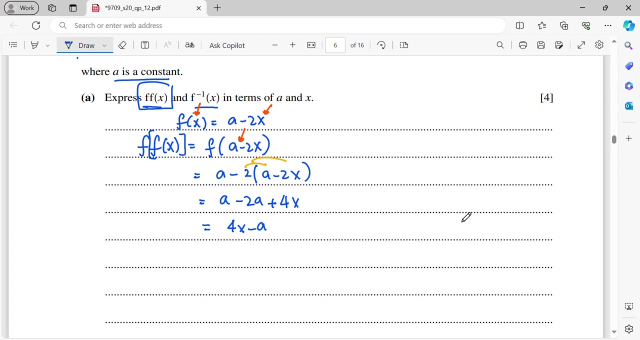 minus 2 times minus 2x it will be plus 4x. so at last I will be getting 4x minus a. that is my f fx. okay, now to get the f inverse. so to get the f inverse I need to get the x as a subject instead of the y. okay, so I let y equals to fx. that means my y is a minus 2x. 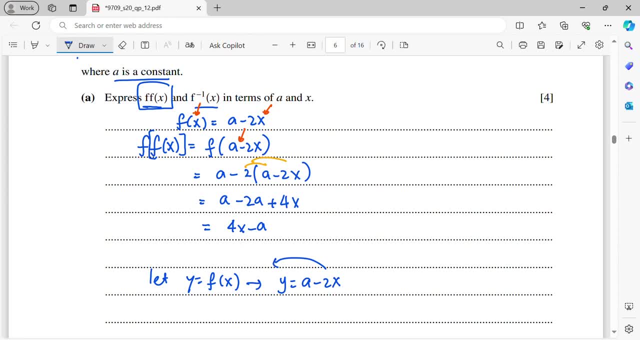 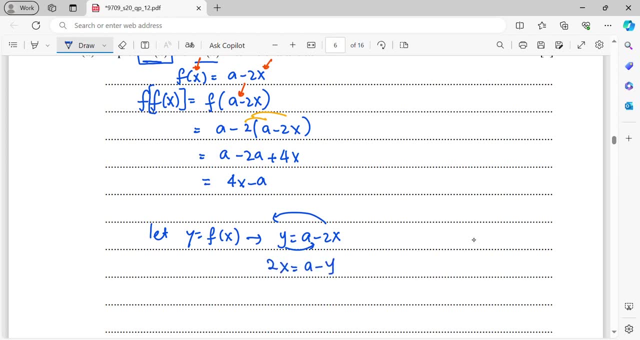 now get the ax as a subject. so means move the minus 2x to the other side and move the y to right side, so I will get 2x equals to a minus y. hence my x is a minus y divided by 2. therefore my f inverse is going to be a minus x divided by 2. so that's all for the solution of this question. 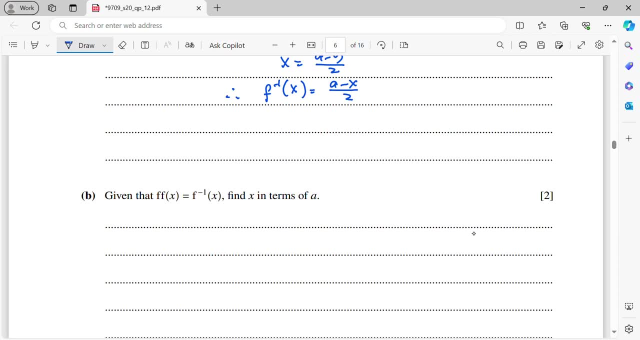 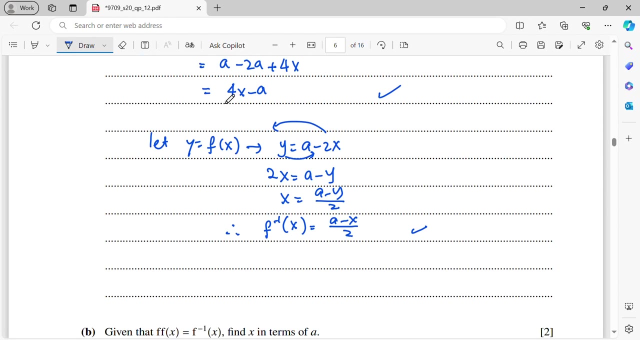 now b, given the composite function equals to the inverse function. find x in terms of a. so composite function equals to inverse function. just refer back to these two equations or to these two functions. so I will write 4x minus a on the left side. right side will be a minus a divided by 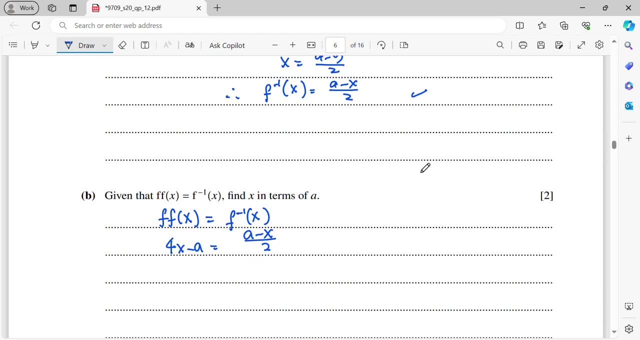 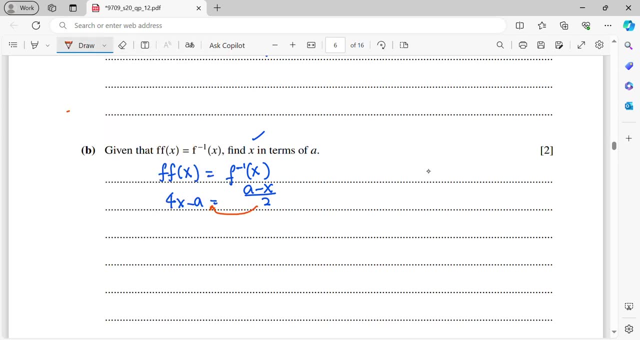 a minus x divided by 2. okay, and now we need to get the x as a subject. so just move this 2 to the other side means that becomes times. so I will get 2 times a minus a divided by 2 times 4x minus a equals to a minus x. and now you need to do expansion. it will be 8x minus 2a. 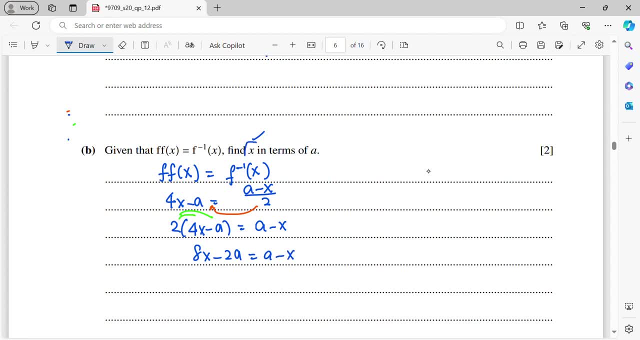 equals to a minus x. and now to get the x as a subject, this minus x on the right side will be moved to the left side and the minus 2a will be moved to the right side. that means now I will be getting 9x, because when you move the minus x to the other side, because plus, and then you will get. 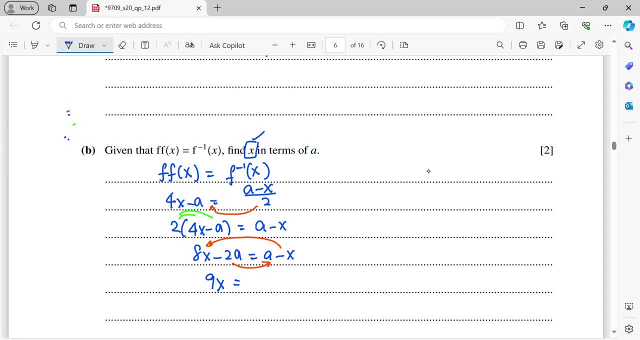 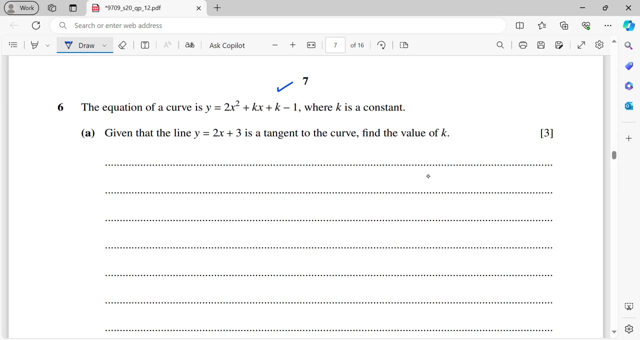 then when you move the minus a to the other side becomes plus 2a, so end up with 3a. so hence your x will be 3a over 9, that is, a over 3. so that's the solution of part b. okay, question number six: the equation of this curve of the curve is given where the k is. 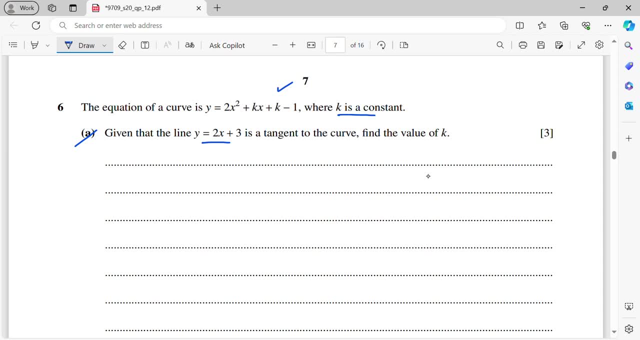 constant a. given that the line is a tangent to the curve, find the value of k. okay. basically, when the line is a tangent to the curve means that there's only one intersection point. or I will say that the discriminant is basically equal to zero. okay, because when discriminant equals to zero, that means there will be only one root, okay. so first, 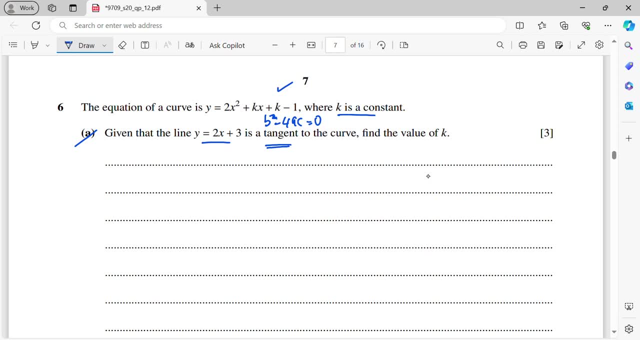 of all I have to find out the intersection point first. I mean the intersection between two graphs, curve and the line. so I will let the curve equation be the two equations here and then the straight line be the second equation. so now to find the intersection points. it basically first equals the second equation, so 2x square plus kx plus k minus 1. 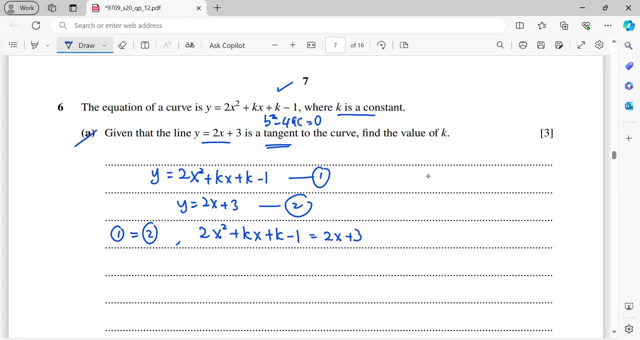 equals to 2x plus 3. and now get a quadratic equation by moving the right side to the left side. so then I will be getting 2x squared plus kx, minus 2x, then plus k, minus 1, then plus 3. move to the other side because minus 3. 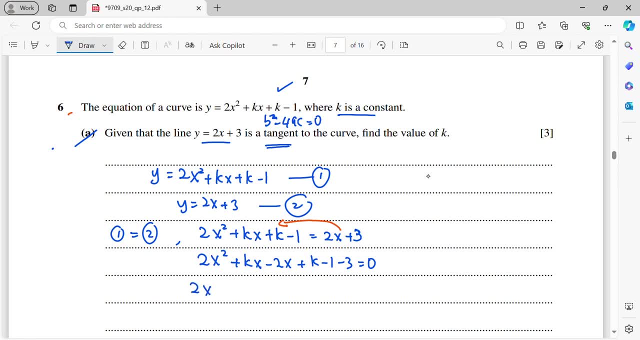 and equals to 0. then from here i will group the x squared and the x. so when group the x you will have k minus 2. okay, because those are the coefficients for x, and then for the last three terms here it will be my constant. so that means this is going to be k minus 4. 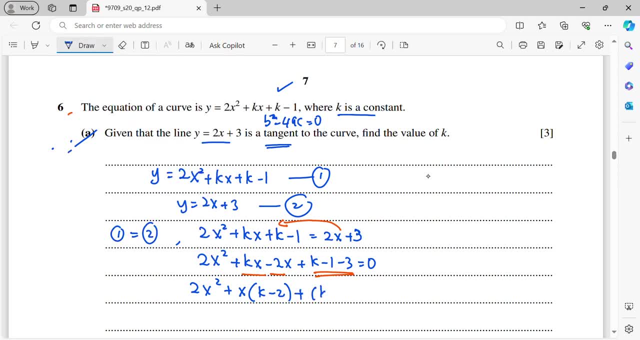 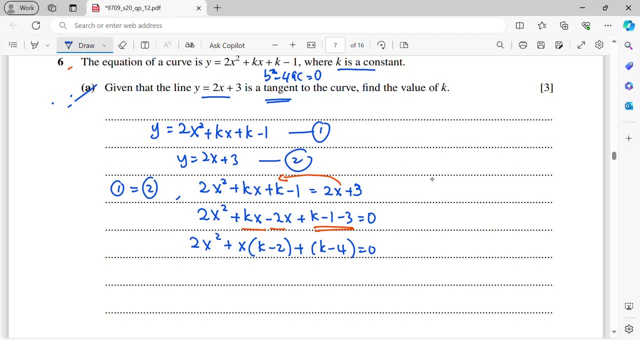 okay, so now write down the coefficient for the x squared, because the general quadratic formula is: ax squared plus bx plus c equals to 0. so i will write down all the coefficients: first my a is 2, my b is k minus 2, and then my c is k minus 4, and then the discriminant. 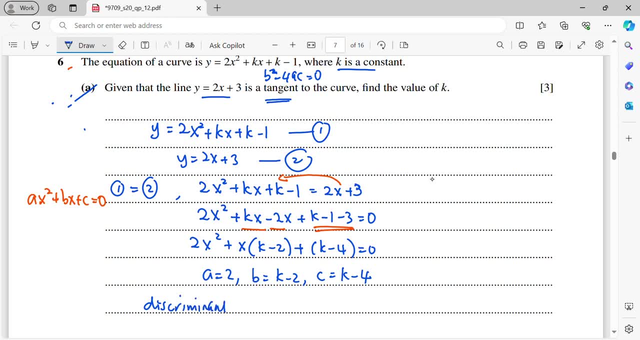 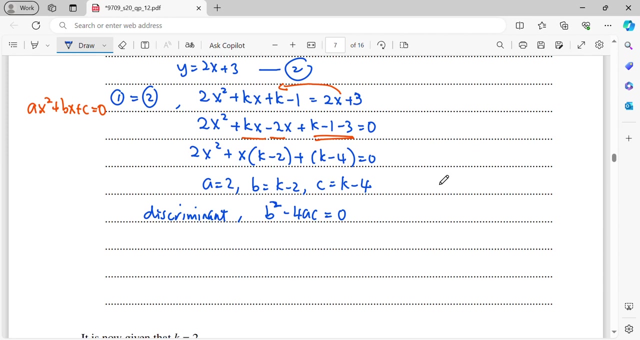 b, squared minus 4ac, equals to 0 because of tangent. remember, tangent means there's only one intersection point, or i would say that the line touches the curve at one point. therefore, discriminant equals to 0. so now just replace k minus 2 squared. 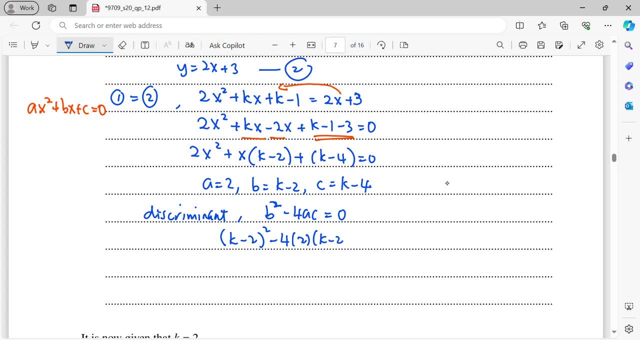 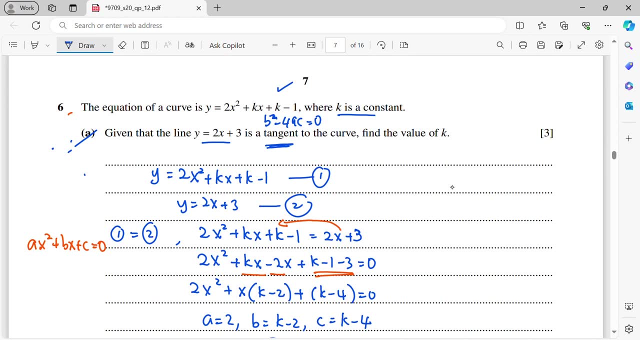 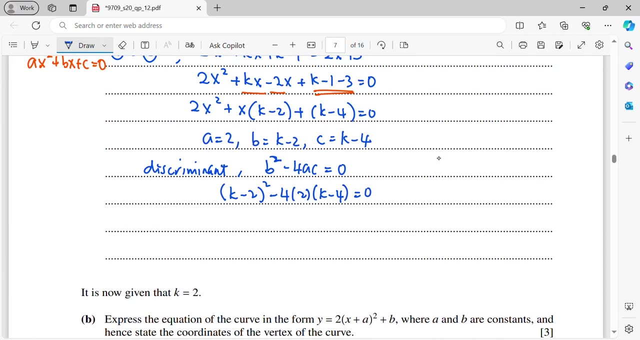 minus 4a is 2. c is k minus 2. sorry, c is k minus 4. that equals to 0. now the question asking for k value only 1k, therefore. now i need to expand this quadratic so a minus b squared you. using the quadratic formula, it will be a square minus 2ab plus b squared. use this: 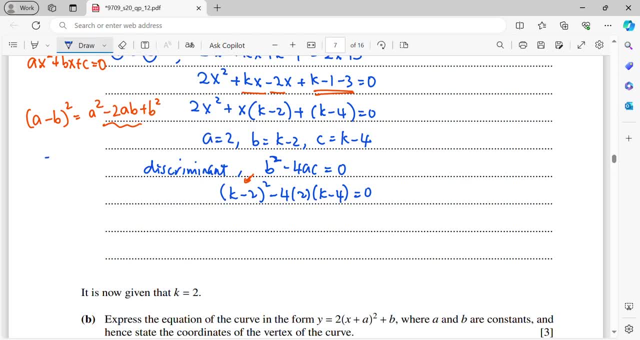 to expand square of k minus 2. that is going to be k square minus 4k plus 4. okay, and then now this is minus 8. so you multiply with k and multiply with minus 4, that will be minus 8k plus 32 equals to 0. and now just simplify it. so k squared minus 4k minus 8k minus 12k. 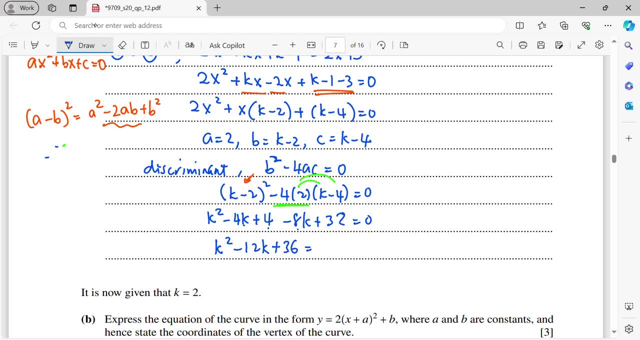 4 plus 32 is plus 36. that equals to 0.. okay, then, from here for the quadratic equation, factorize it and you will be getting k minus 6 squared equals to 0. hence your k is going to be 6. all right, that is the value of k, only 1k. 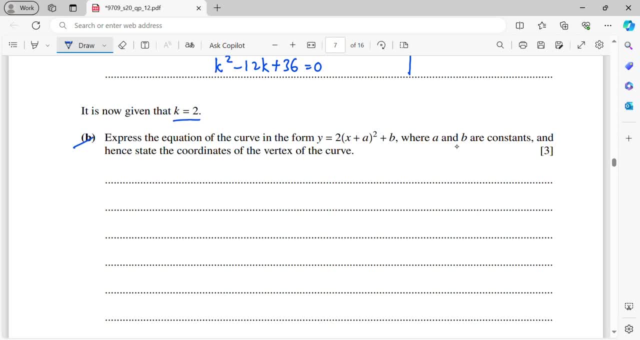 okay, now it is given that k equals 2. b express the equation of the curve in this form, where a and b are constants and hence. so this is the first part. second part is state the coordinates with the vertex. so the vertex here means the maximum or minimum point. so now replace the k by 2. 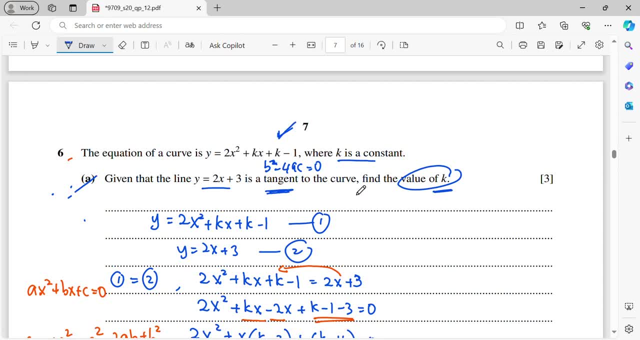 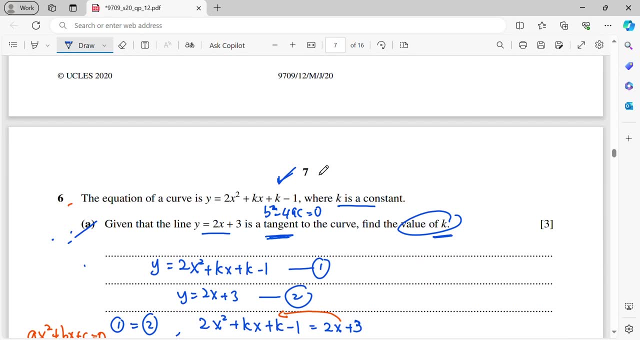 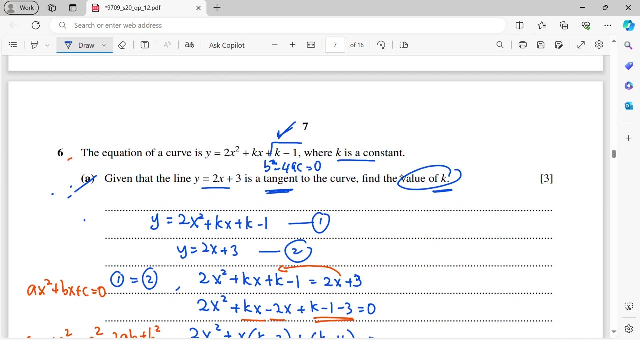 so all right, replace the k by 2 first, so 2x squared. then plus kx, that means plus 2x. after that, for the k minus 1 plus k minus 1, your k is 2, means that 2 minus 1 is 1. so here: 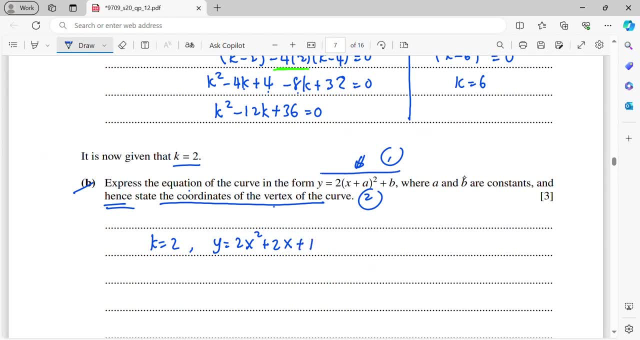 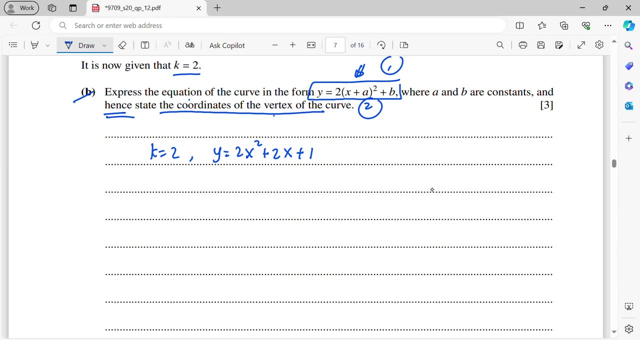 becomes plus 1.. okay, so to get the, to get this form, this is basically completed square form. so, according to the completing the square method, first step is to get the positive 1 for the coefficient for x squared, which means now i have to factorize 2 from all the terms. it will be x. 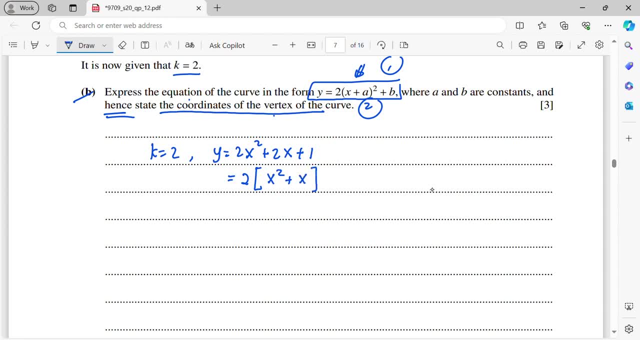 squared plus 1x, then you can just leave it outside for the plus 1, because we have the plus b at the back right. so now you rewrite these two terms inside the bracket and then we need to plus square of a term and minus square of the term, then plus 1. so these two brackets are the additional terms. 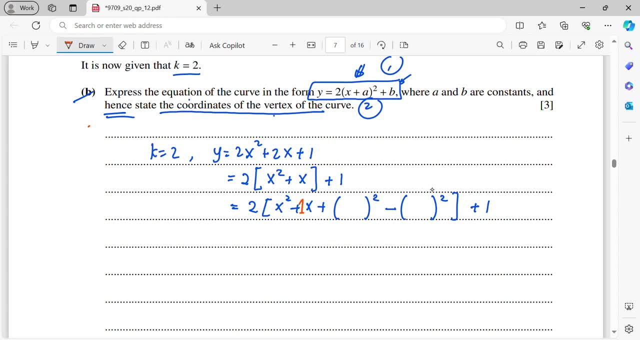 the term inside the brackets is basically the half of the coefficient of x. your coefficient of x is plus 1. therefore, it is plus 1 over 2. okay, this is how i get it. so then, from here you just refer to the first and third term. combine these two terms and take out the squared. 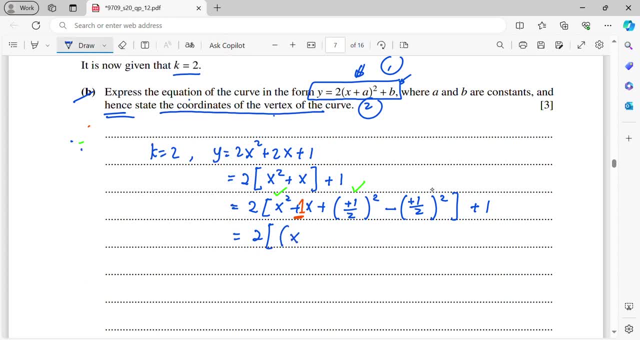 means that i will get x. the second term here will be inside the bracket. it is plus 1 over 2. that's why i copy: plus 1 over 2 and then minus. you expand this square of half is basically 1 over 4, then plus 1. then now look at here: you need to get b outside. therefore i will get 2. okay, this 2 you. 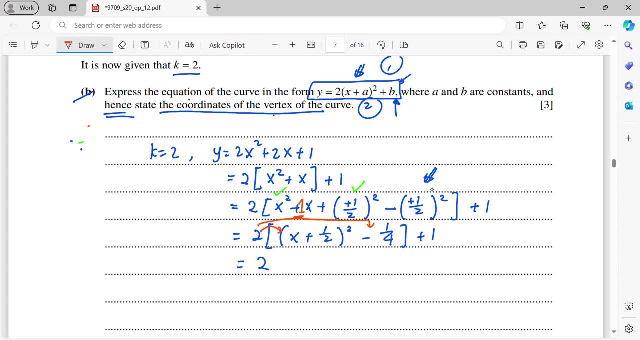 multiply to the bracket and to the negative: 1 over 4. therefore you are looking at the negative 1 over 4. therefore you are getting two of x plus half squared. so two times minus one over four is basically minus half, then followed by plus one, and now here i will get two brackets x plus half. 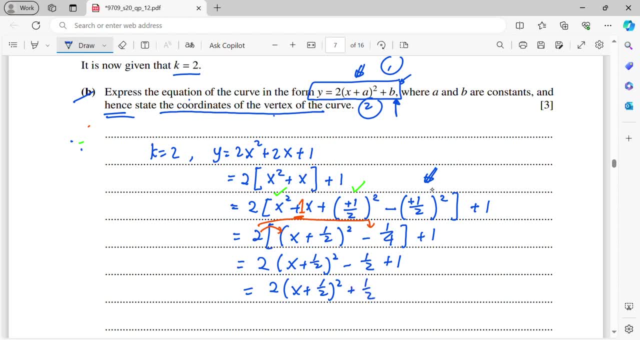 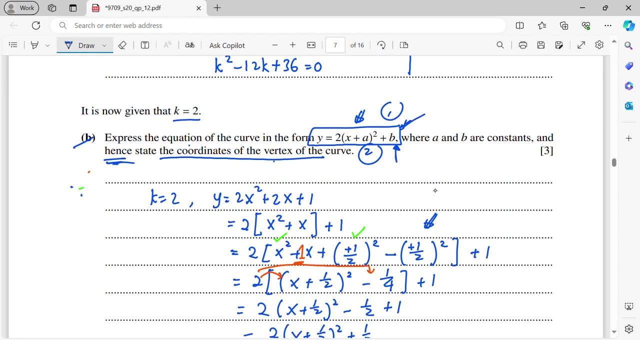 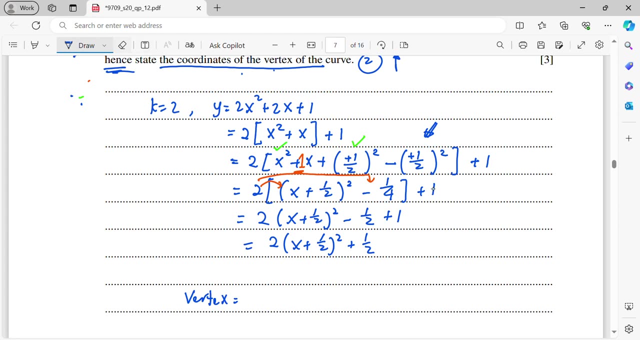 squared now, minus half plus one is plus half. therefore i have found the expression. okay, this is the expression now. hence state the vertex. so basically the vertex is the maximum or minimum point. so you just let this be zero, right? so probably i will write here: x plus half equals. 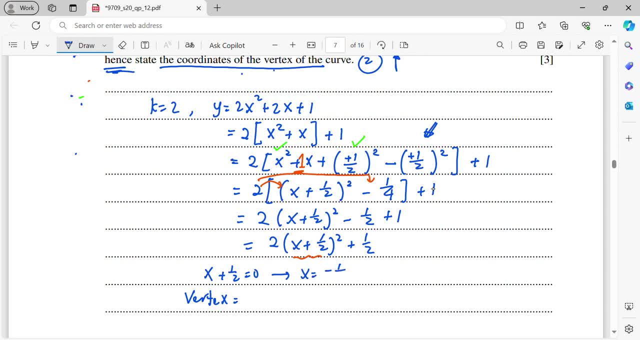 zero. that means your x is negative half. so that is my x coordinate of the vertex, negative half. and then my y coordinate of the vertex is going to be plus half. this is my y coordinates of the vertex plus half. so that is the expression coordinate of the vertex. so here I will just add on positive half. so that's all. 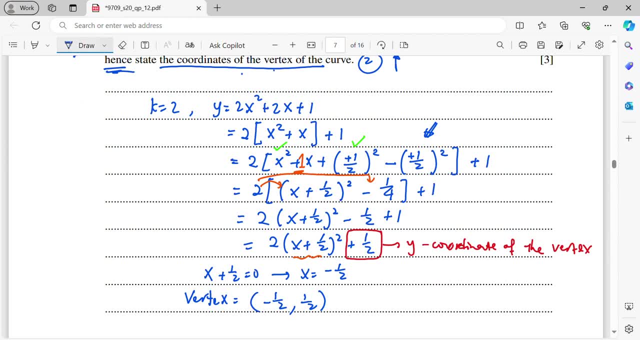 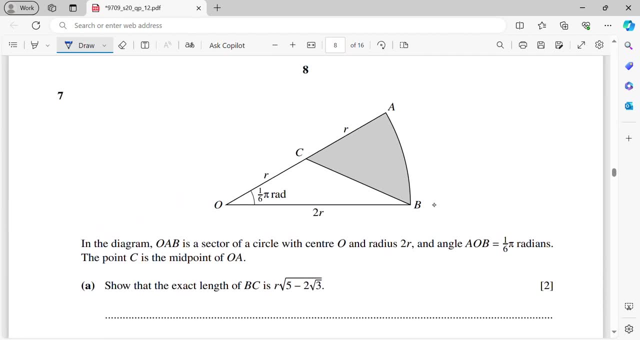 for the solution. okay, now question number seven. in the diagram OAB is a sector of circle. refresh the center O and radius to R. okay, so OAB, that means here is to R. now an angle AOB is 1 over 6 Pi. even the point C is a midpoint. 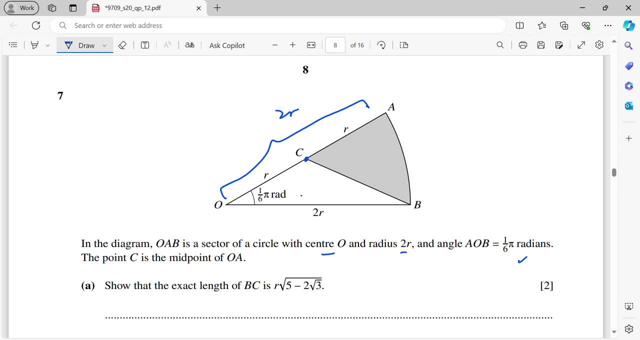 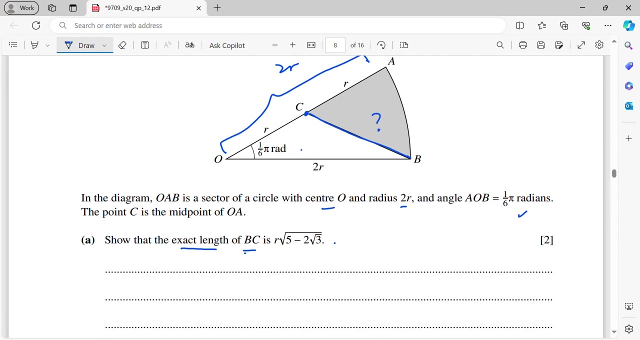 since this midpoint that means OC is R is R, show that the exact life of B C called food. so BC is district line. okay, it's given by this now from here. okay, I can just use the cosine rule right, because we have two sides and one angle, so you can. 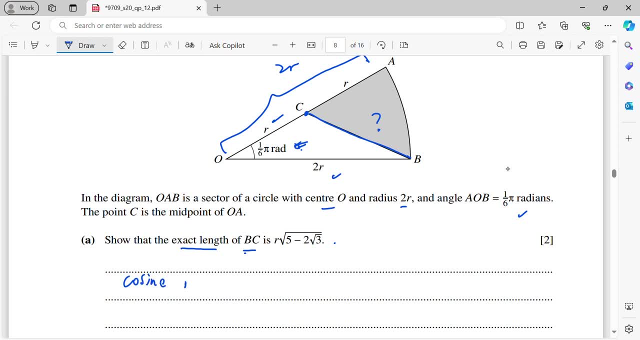 just use cosine rule. so cosine rule, cosine rule, is basically like this: here a, here BC, this is theta. so as long as the angle opposite to the- I mean the sides opposite to the angle- is B, so I will just write: B square equals to sum of the other two squares minus 2ac. cos theta. this is a cosine. 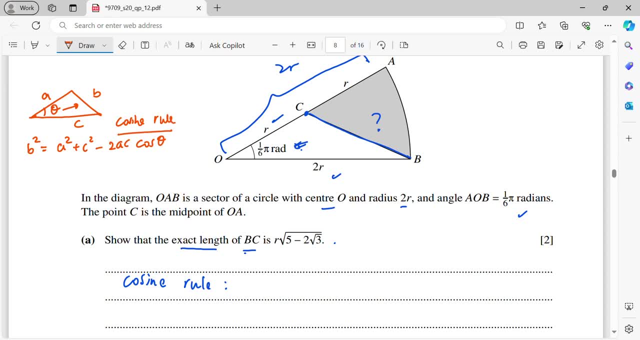 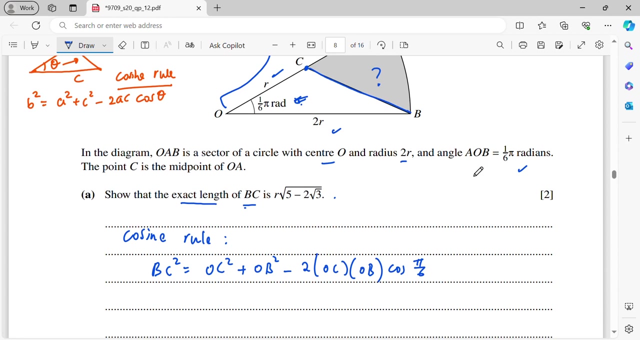 sine rule, right? so that means here I will just write: BC squared equals to OC squared plus OB squared minus 2 of OC, OB cos pi over 6, right? so now OC is R, so R squared OB is 2R. 2R square minus 2R times 2R. 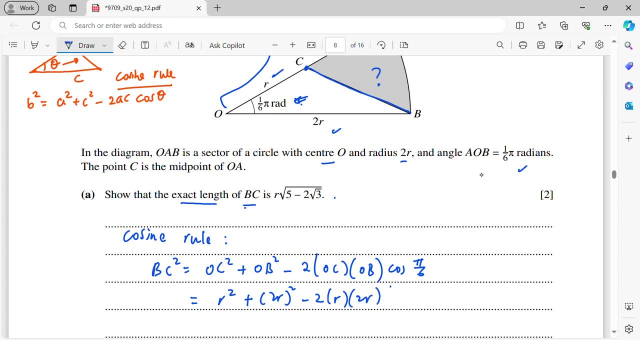 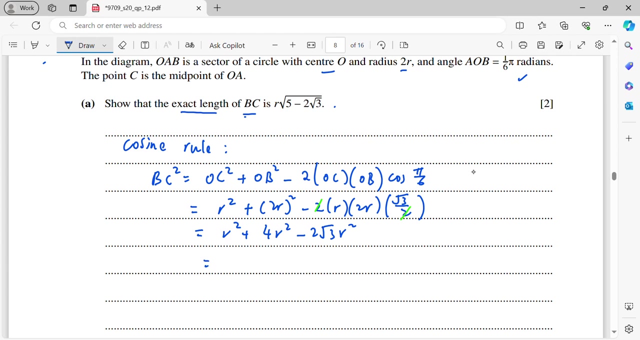 cos pi over 6 is basically square root, 3 over 2, so from here I can cancel off the two and half, right. so then here will be R square plus 4R square, then 2 square root, 3 R squared, and now R squared plus 4R squared is 5. 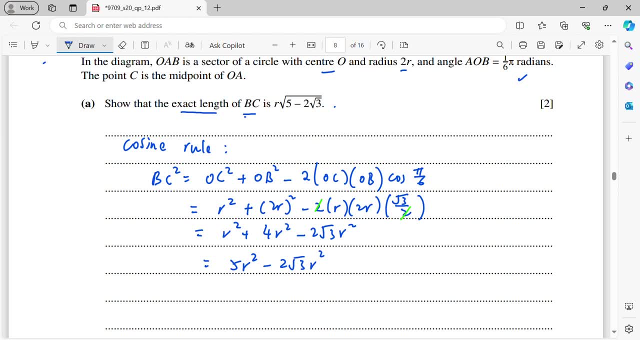 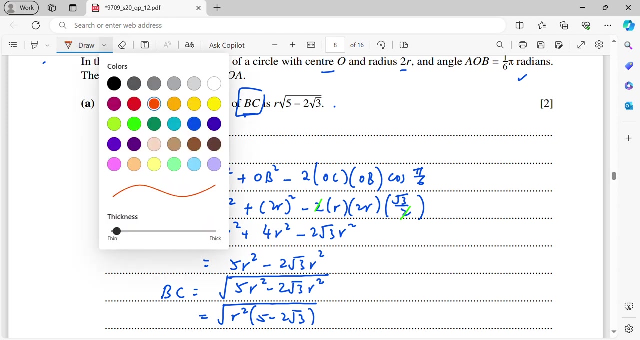 r squared minus 2 square root 3, r squared. and now to get the bc, we need to take square root and we know that r squared is in common, so you can factorize r squared. there will be 5 minus 2 square root 3. and now, for your information, square root of a times b. 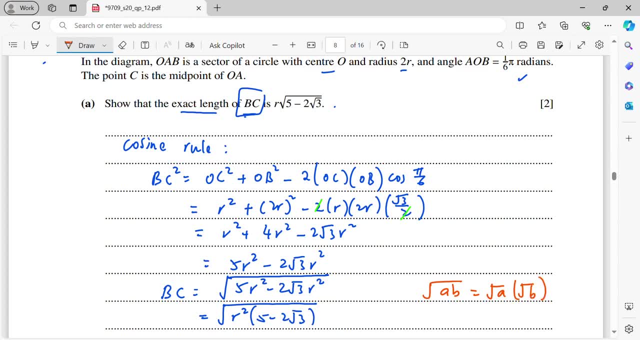 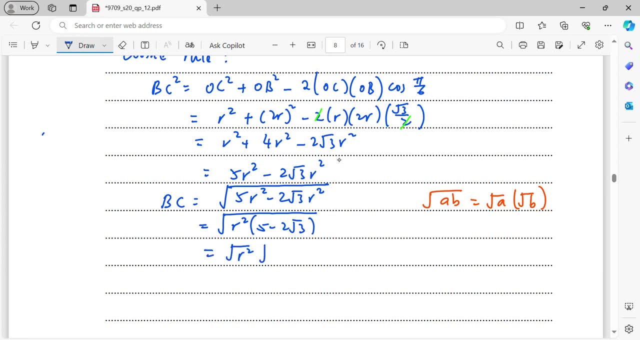 is basically square root a times square root b, so square root of r squared times the bracket. i can split it into: square root r square times square root 5 minus 2 square root 3, so square root r square is r, so r square root of 5 minus 2 square root 3. so this is the answer. 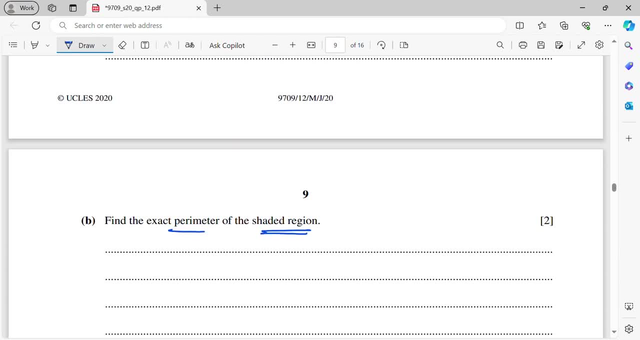 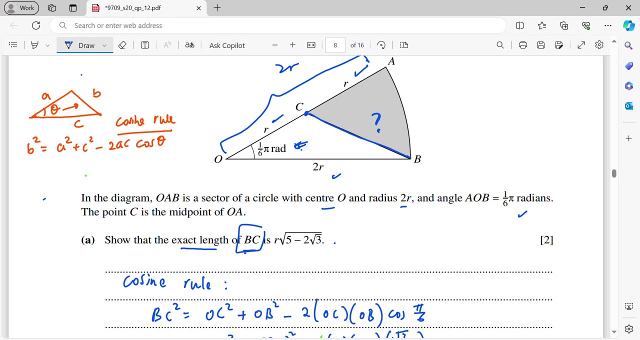 okay now b- find the exact parallel meter of the shaded region. okay, go back to the diagram. we have found this pc, and then the ca is given. so now i just need to find out what is my a b. so the a? b is actually the length of the sector. 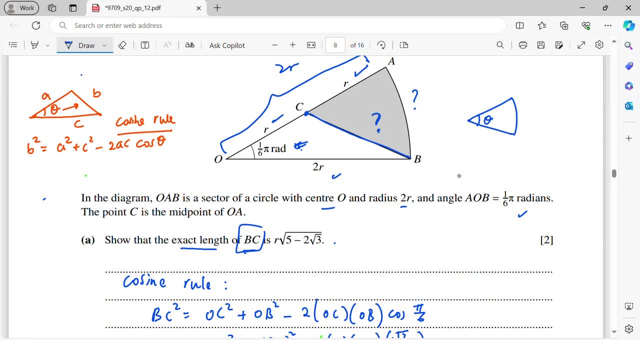 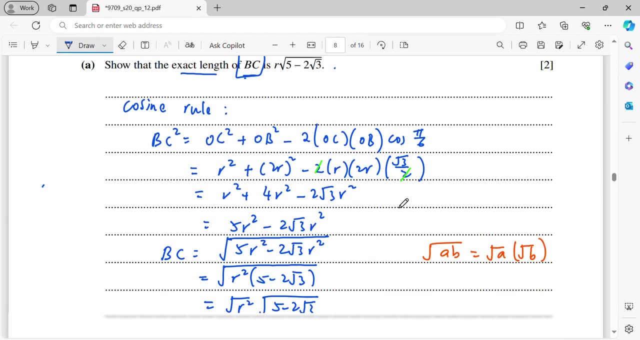 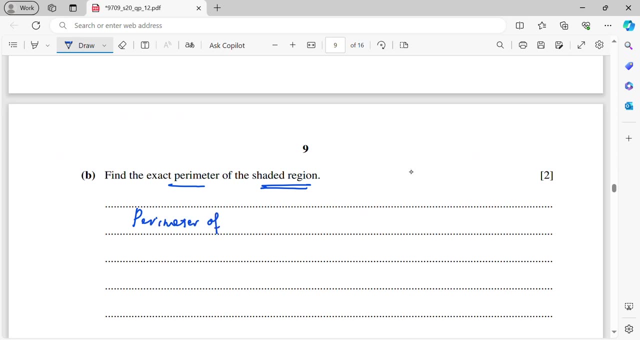 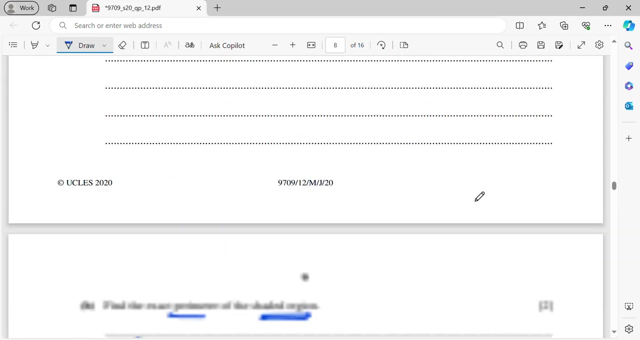 for your information, let's say this is theta, the radius is r, so the art length here, which is s, i will write s equals to theta r, okay? so from here i will just write: perimeter of the shaded region equals to c a plus c b plus art length of a b. so c a plus c b plus art length. 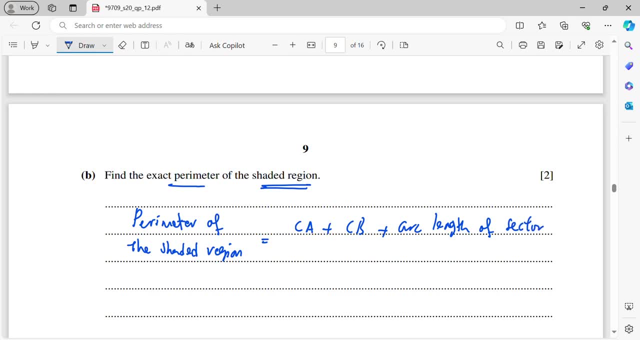 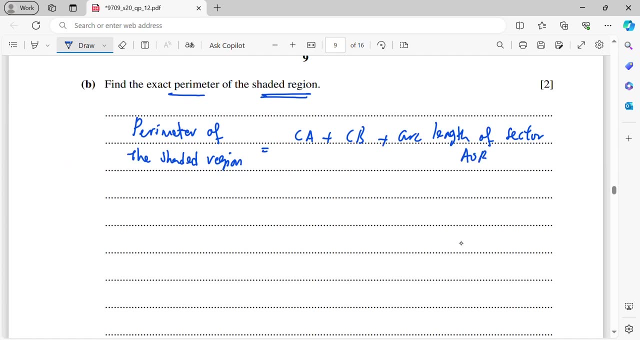 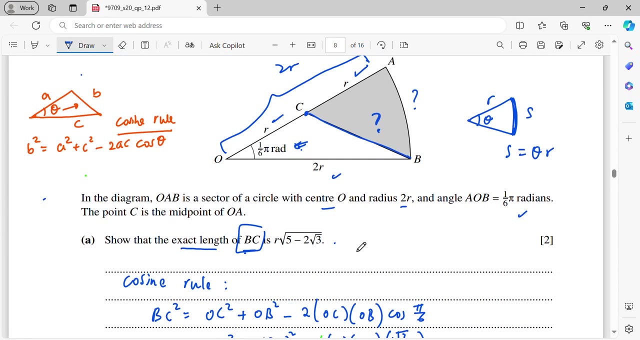 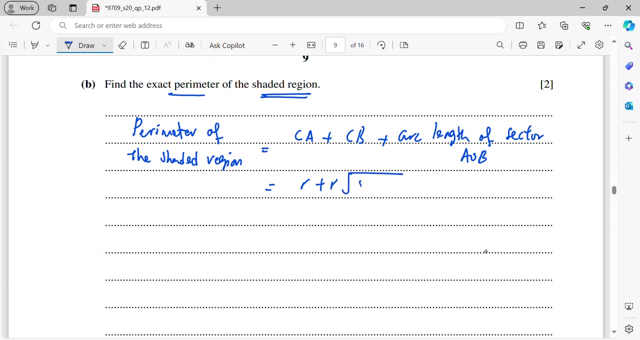 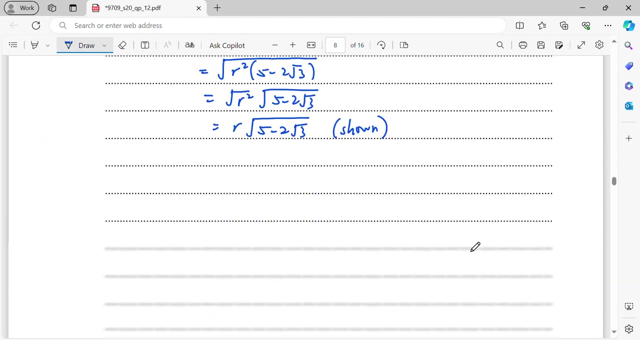 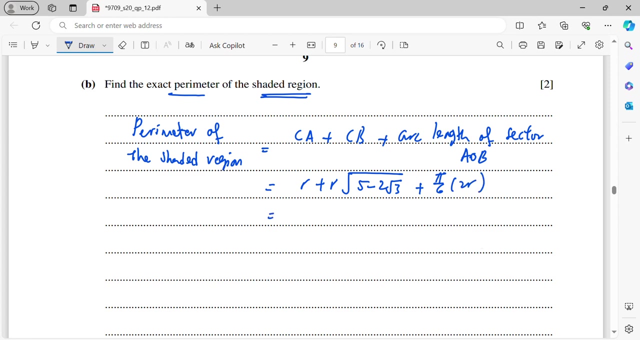 um of sector aob. so c a is given our cb. we have just shown. okay, just copy: all this is basically a theta r. so now your radius is 2r, theta is pi over 6, so pi over 6 times 2r. that means now here: 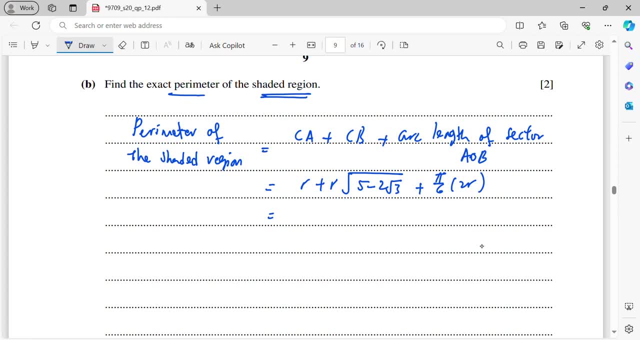 2 and 6 can be simplified into over 3, so here i will get r plus r, square root 5 minus 2. square root 3 plus pi over 3 r. so from here, if you want, you can just factorize r, which is in common. 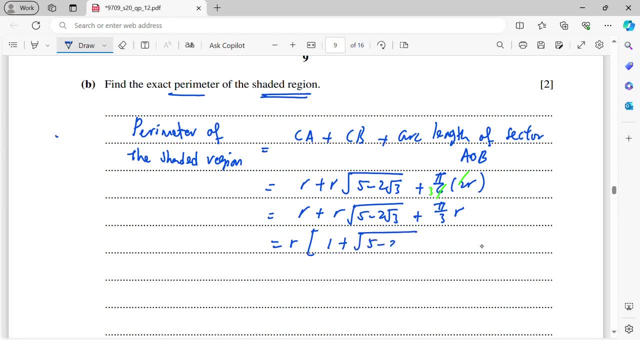 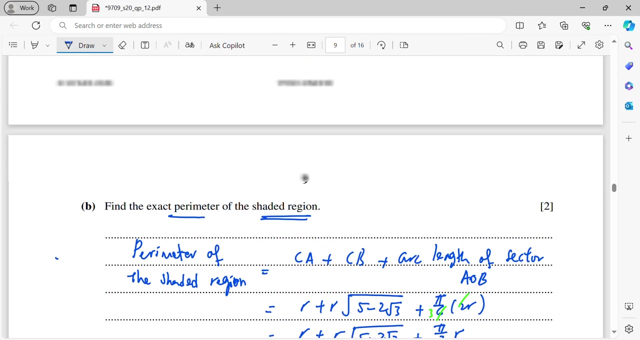 so 1 plus square root of 5, minus 2 square root, 3, then plus pi over 3, so that is the perimeter of the shaded region. see, find the exact area of the shaded region. so to get the area, okay, i will say that it is. 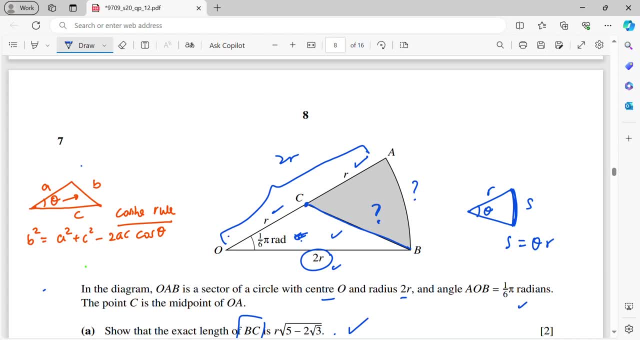 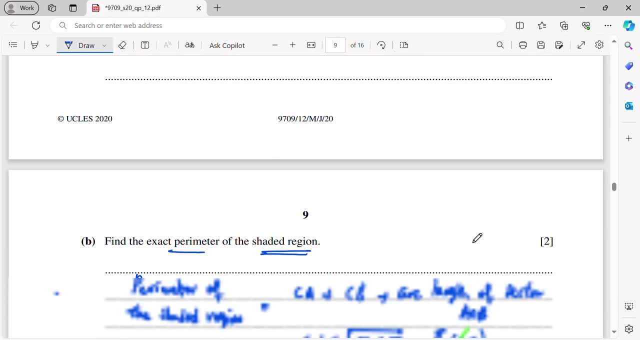 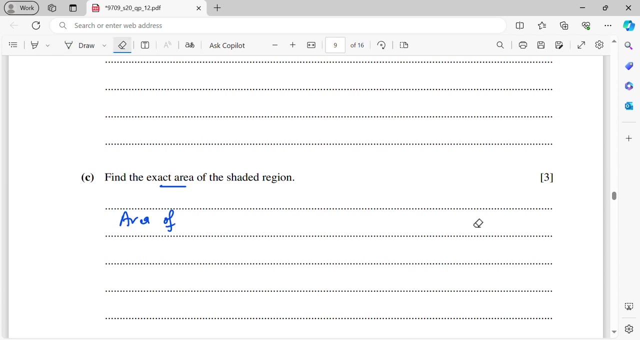 area of the sector a or b minus area of triangle ocb. okay, so i will say that it is area of the sector a or b minus area of triangle ocb, right? so area of sector formula is, or i will just write down here's first: area of the shaded region. 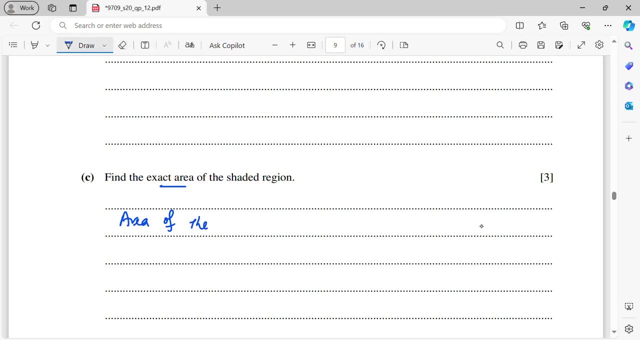 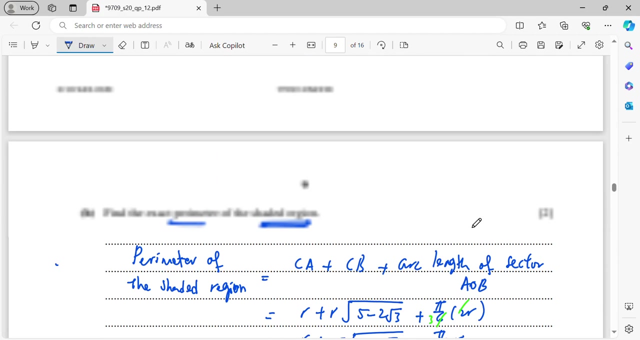 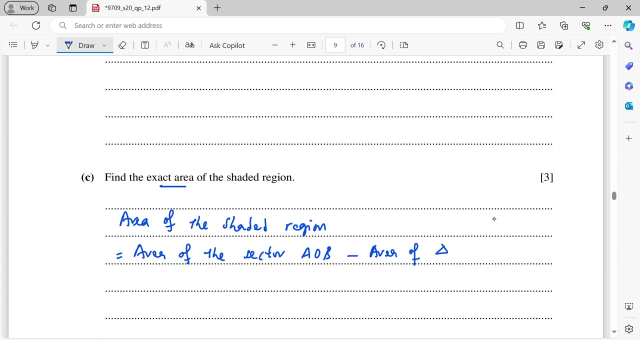 equals to area of the sector a or b minus area of triangle. okay, so this area, let's say here is the general form, so the area is basically half theta r squared. so now i will get half. my theta is pi over 6, my r is 2r, so you square it, okay, minus area of triangle. okay, let's say this is a triangle. 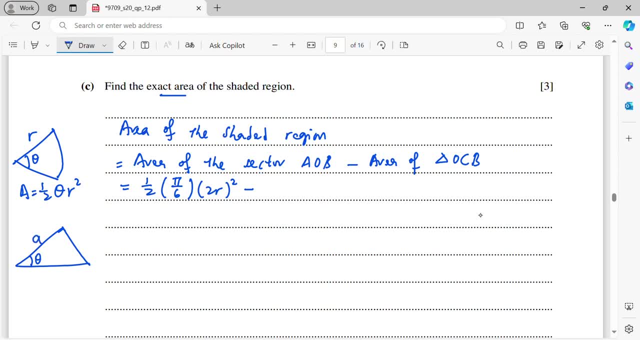 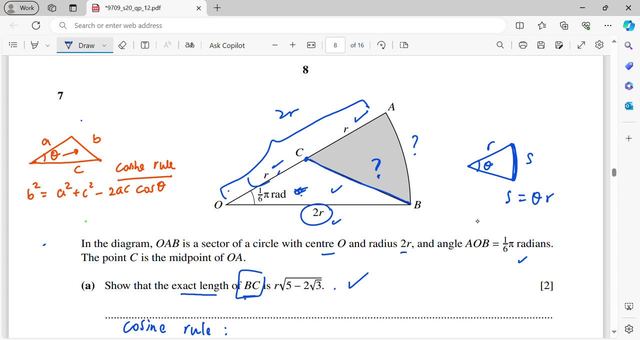 and now we know that here is the theta. so unless as long as you know these two sides, so the area is half a b sine theta. okay, therefore i will get half. now go back to the triangle. so half oc ob sine pi over six. so i will write half r times two r. 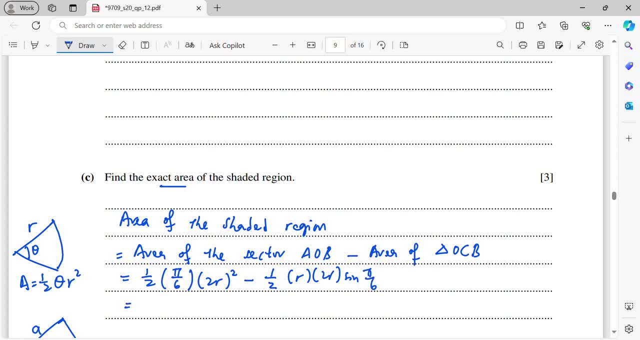 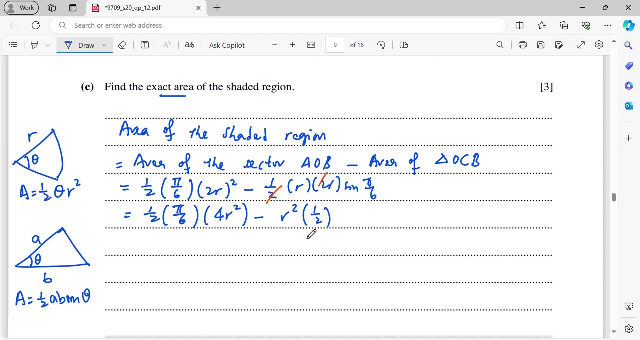 sine pi over six. okay, then for the first term you will get half pi over six. this is basically four r squared. then minus the half and two, cancel off, i'll get r squared sine pi over six. so sine pi over six is basically half. right then, now you can simplify. 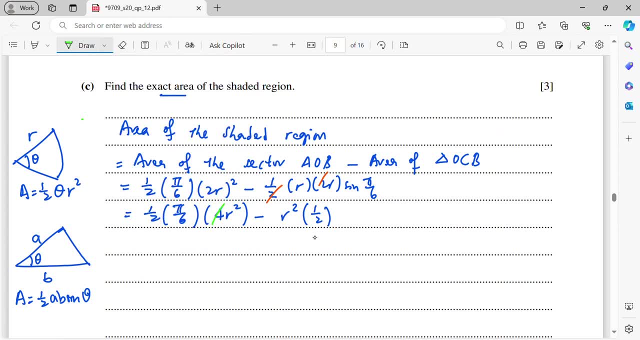 here is okay, this is two. cancel then these two. cancel with the over six, this is three. so that means you will be getting pi over three r squared minus half r squared. then from here the common term is over six, one over six r squared. so when i factorize 1 over 6 from 1 over 3, that is times another 2, so 2 pi, then same goes. 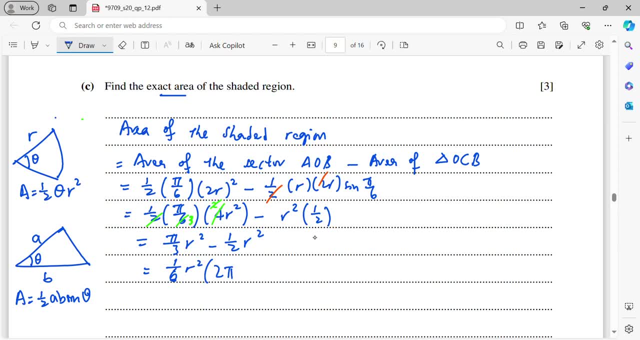 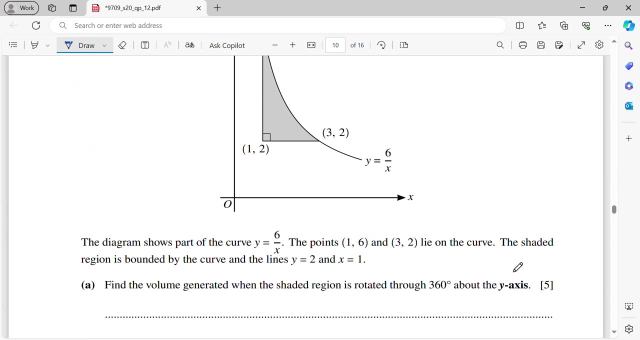 to the next term minus half. when you factorize 1 over 6 from half, that is 3, so that will be the exact area of the shaded region. okay, question number eight. the diagram shows the parts of the graph. the points one, six and three two lie on the curve. so, given here, oh, one six. one six is also. 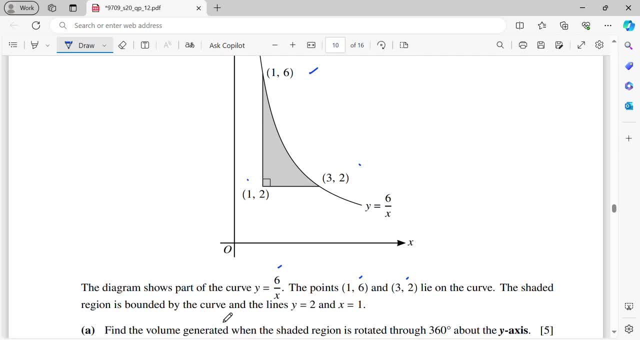 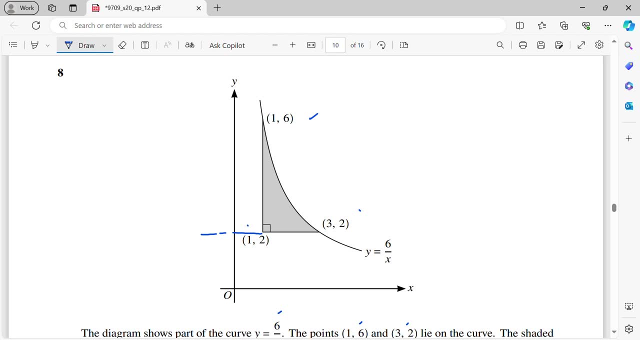 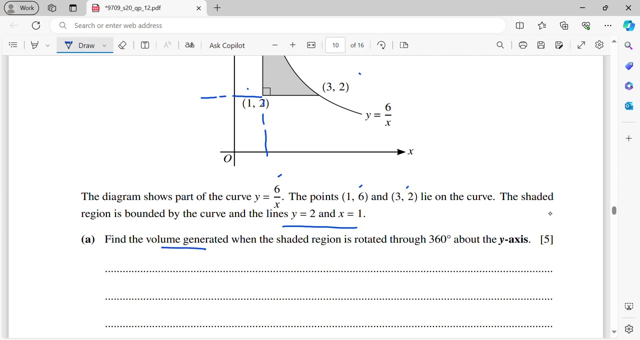 given right the shaded region is about is bounded by the curve and the lines y equals to two and x equals to one. so y equals to two. this is y equals to two, x equals to one. all right, find the volume generated when the shaded region is rotated through 360 degrees above the y axis. okay, so. 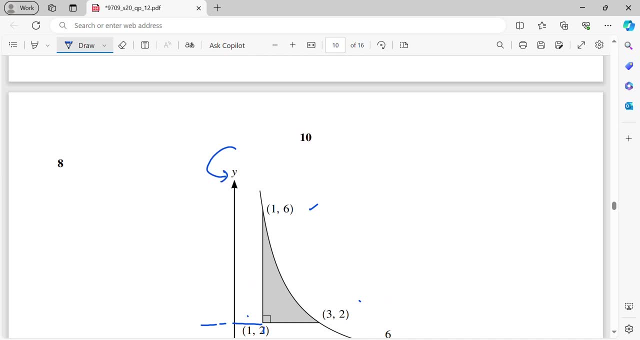 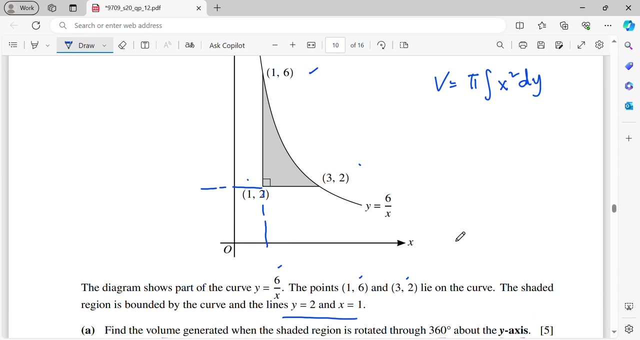 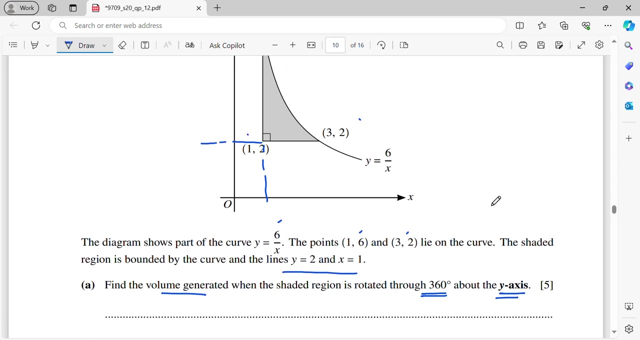 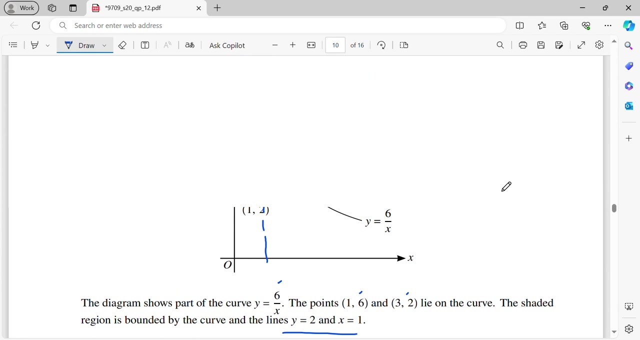 when it is about the y axis, our formula is: v equal to pi, x square d, y, right, okay. so from here about the y axis, i start with: y equals to 6 over x first, so now i must get x square. okay means that i need to get the x value. 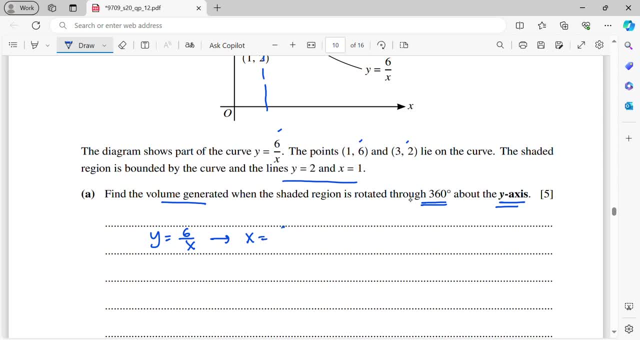 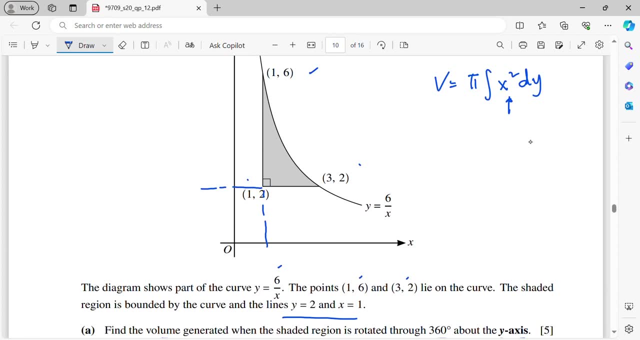 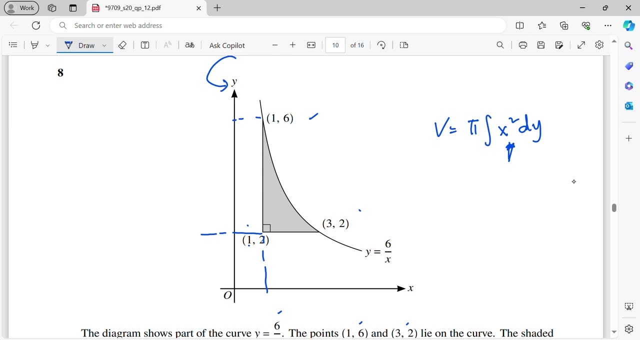 so my x just move up and move down the y, it will be 6 over y. okay, then when you just directly integrate this right, use this formula and then the y value obviously is from: this is x is one, y is two. so x is one, y is two, this is one, all right, so when you integrate 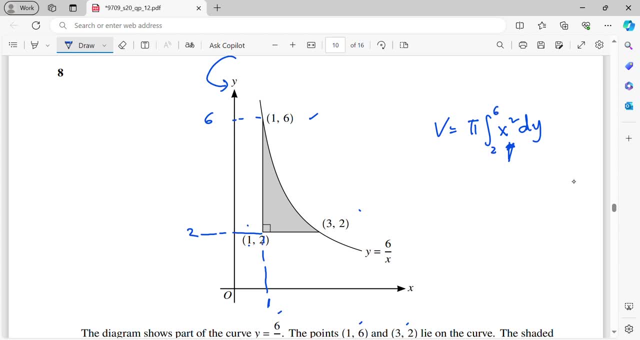 from 2 to 6, this part. that means you are finding the area towards the y axis, which is here. okay, which is not correct. okay, because our shaded region is just this part. so what to do now? here is- i have to refer to this line, this is my, let's say, this is my x1. that means here is my x1. 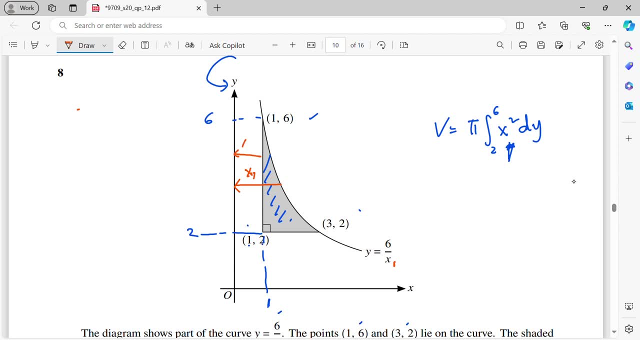 here, then i need to minus this line: this is my x2, so obviously my x2 is 1, okay, because of the coordinate. so i need to minus and then you square and minus. it's like you find the area. if the volume of this graph means everything right, which means like this: you find the 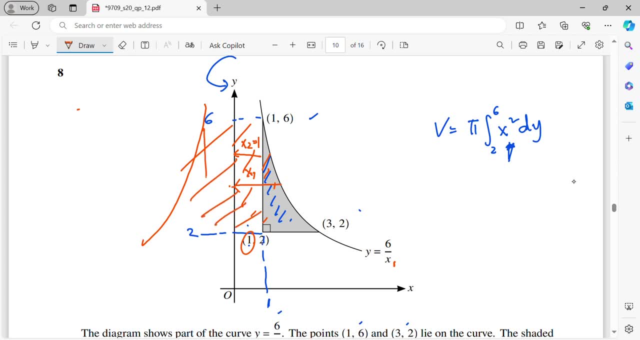 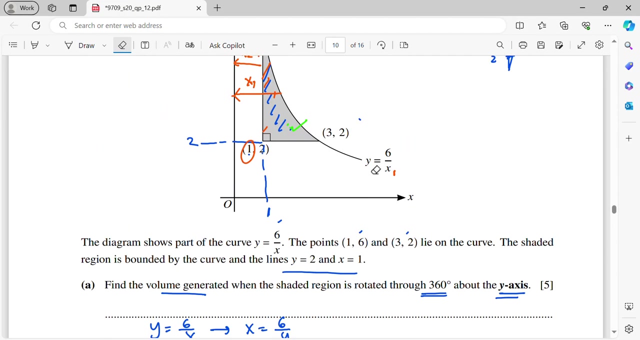 volume of everything. then you minus the middle value, the hollow, because the middle is hollow, right, you minus this. that will be the volume of this part, okay, so therefore, the idea is you use a longer y, a longer X minus a shorter X. okay, so my x1 is from the. 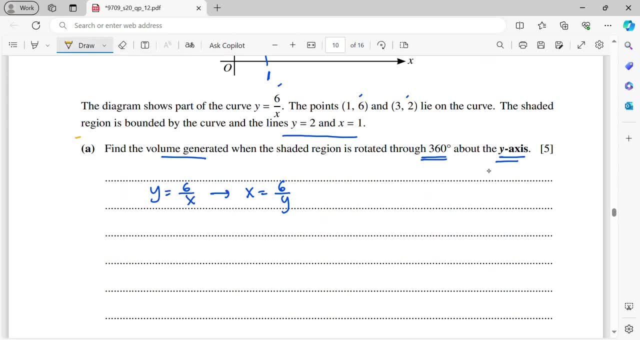 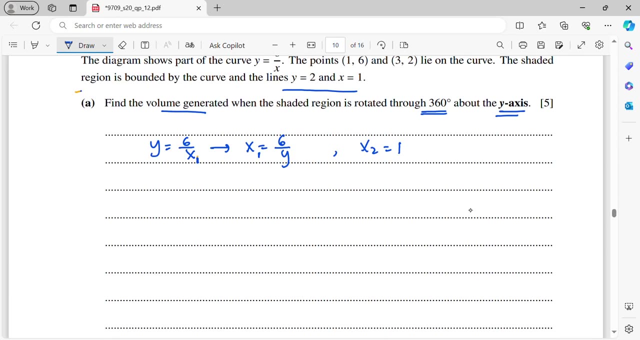 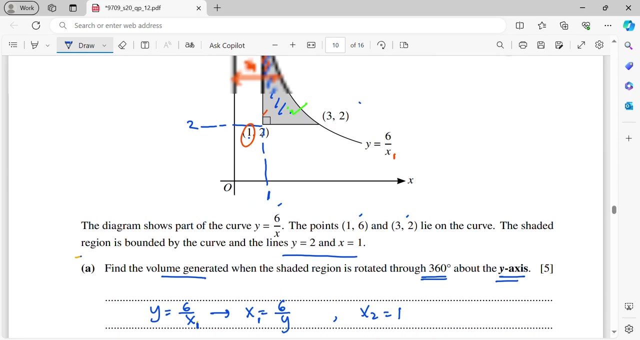 graph. so that means this is my x1, so my x2 it will be 1. okay, according to this to the explanation here. so now my volume equals to PI integrates from 2 to 6 due to the y coordinates. okay, 2 to 6 after that. 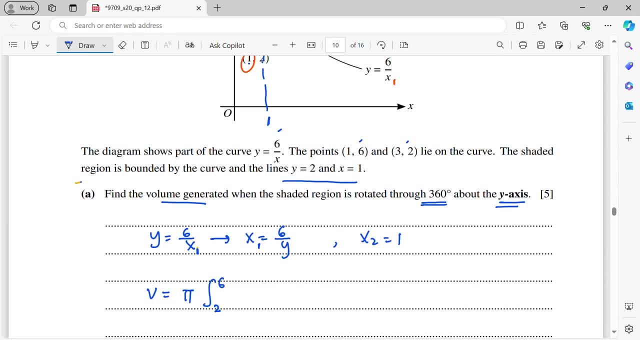 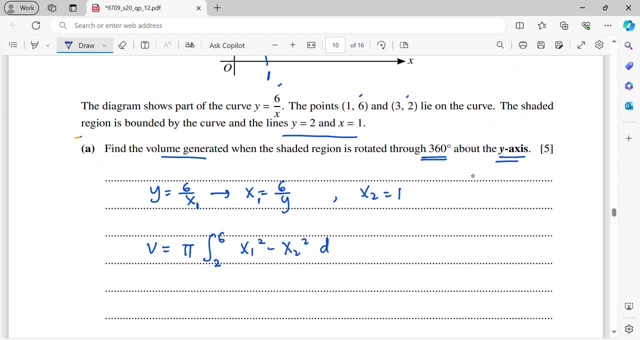 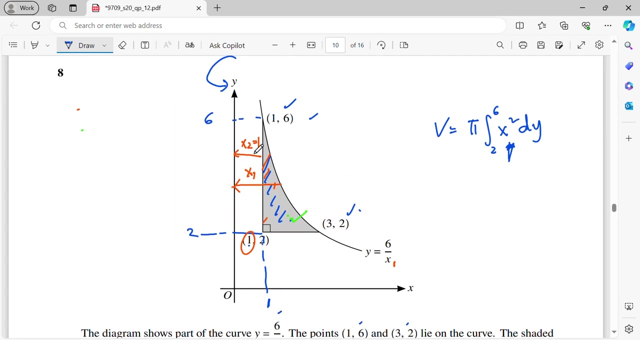 x1 squared because the x1 is longer. so x1 squared minus x2 squared, then dy. then from here I will write: pi: integrate 2 to 6, my x1 square is 6 over y squared. my x2 square. x2 square is basically 1. 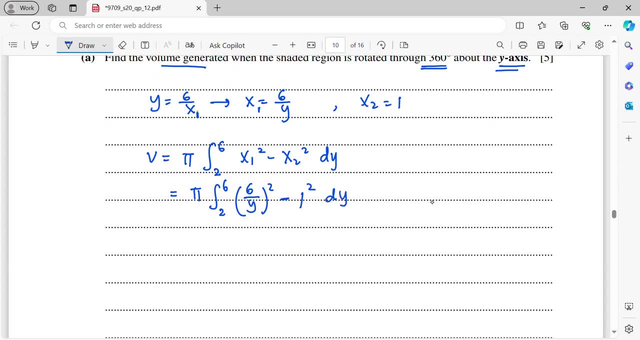 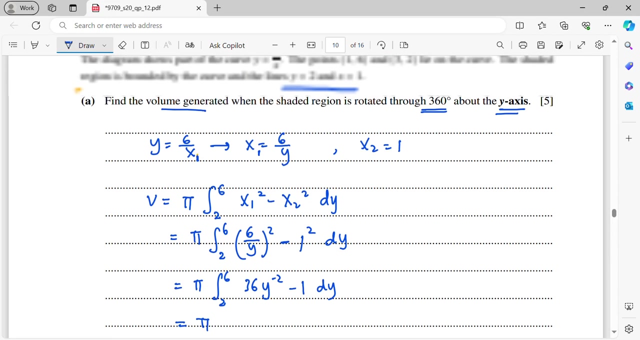 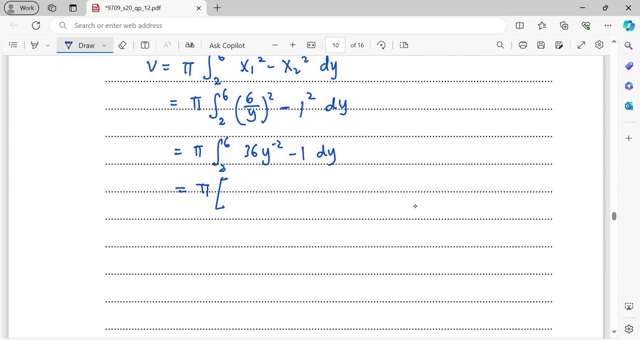 so 1 squared. then from here, before I integrate, okay, this square, I move in first and I move up the y, then you will be getting 36 y to the power of negative 2, then minus 1 dy, so that is going to be pi 36 when you integrate, okay, integrate x degree n dx, that is, x degree n plus 1 over n plus 1. then 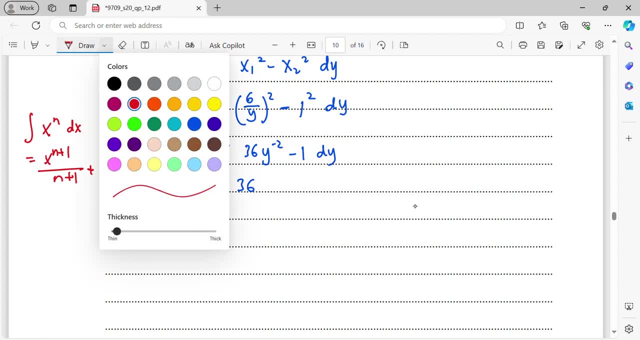 plus c. so now this formula is valid. when the n is not minus 1, then from here I will be getting y to the power. negative 2 plus 1 is negative 1 over negative 1. you integrate minus 1 is minus y, limits from 2 to 6. then now here I rearrange. 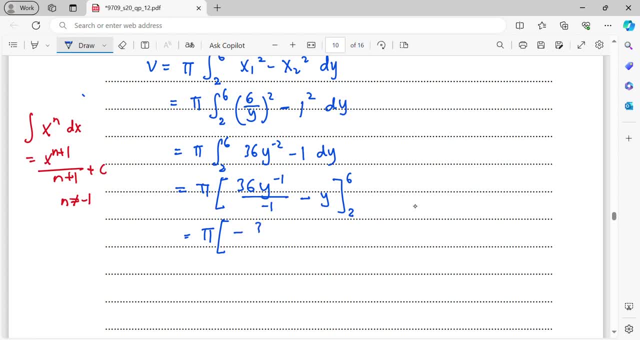 the first term it will be negative 36 over y, then followed by minus y from 2 to 6. and now here, when I replace the y by 6, I will get minus 36 over 6, then minus 6 and minus the lower limit, so minus. 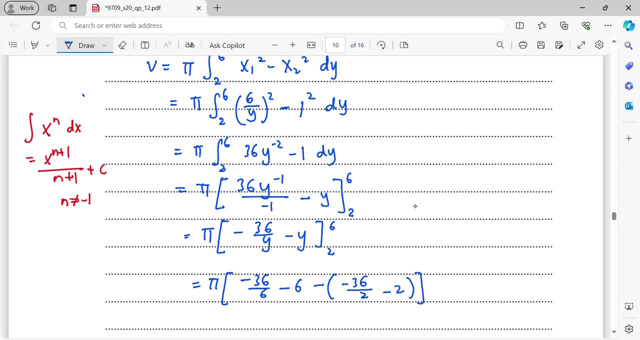 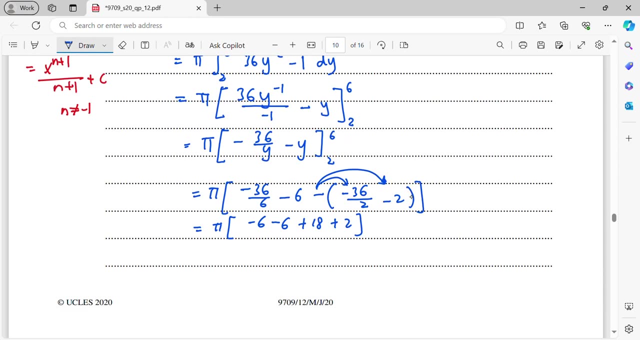 36 over 2 minus 2. okay, so you will get minus 6 minus 6, and then this minus minus is a plus, so plus 18, and minus minus is another plus, so plus 2. that means now here. okay, so when you look at this, this is 20, here is 12, so 20 minus 12, that is 8, so your. 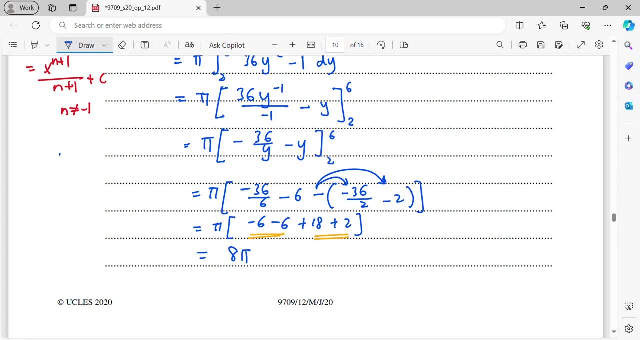 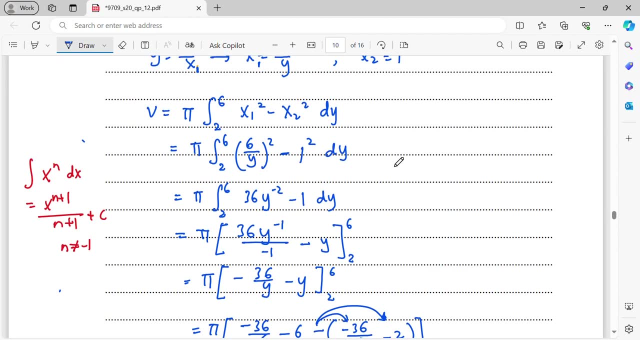 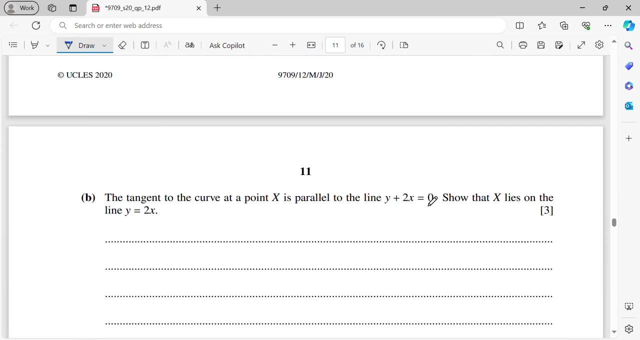 answer is 8 pi. okay, so be careful with this because it is hollow right. so you have the minus. x equals to 1. okay, done for this part b. the tangent to the curve at point x is parallel to the line show that x lies on the line. y equals to 2x. so 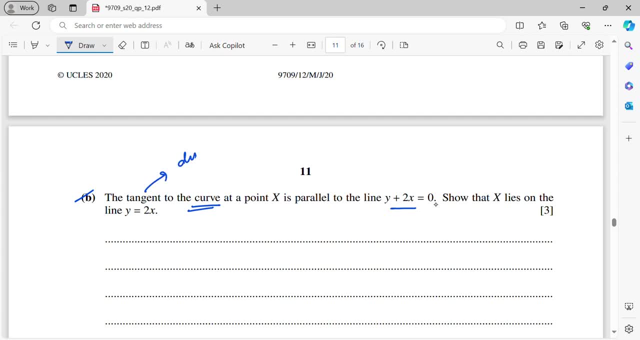 now the tangent to the curve. so whenever you see tangent means that dy over the x. so now my y is 6 over x. this is same as 6x to the power of negative 1. I find out what is my dy dx. first x, so now my d y dx. when you differentiate, keep the x, keep the 6 x power negative 1, you get negative x. 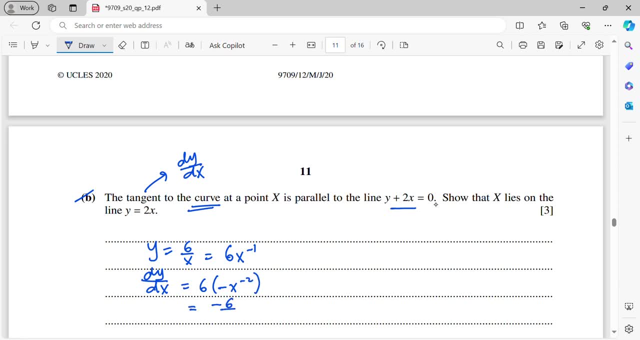 negative 2. that means this is going to be negative 6 over X squared. okay, and now it's mentioned that the tangent, this gradient, this dy dx is actually the gradient of the tangent- is parallel to y plus 2x. so where y plus 2x equals 0, I need to get the gradient from this line, which means y equals to negative 2. 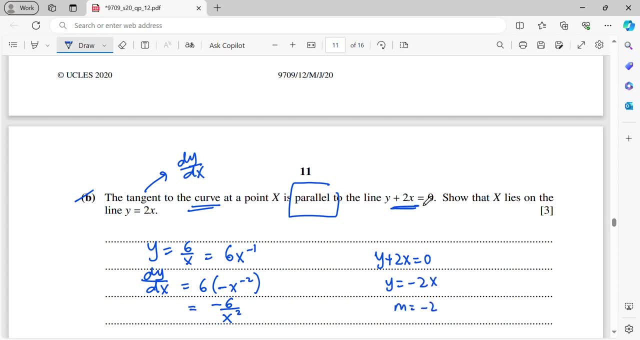 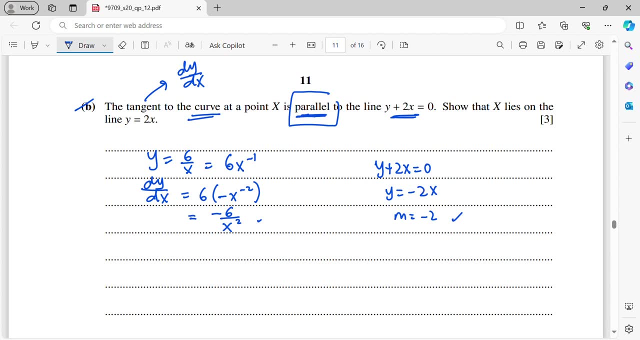 so the M equals to negative 2, which means okay. so this dy dx will have the gradients of negative 2 because of the parallel. parallel means that they will have same gradient. so now I will write: negative 6 over x squared equals to negative 2. I expect I'm expected to get the X from here. so what to do is the 2. 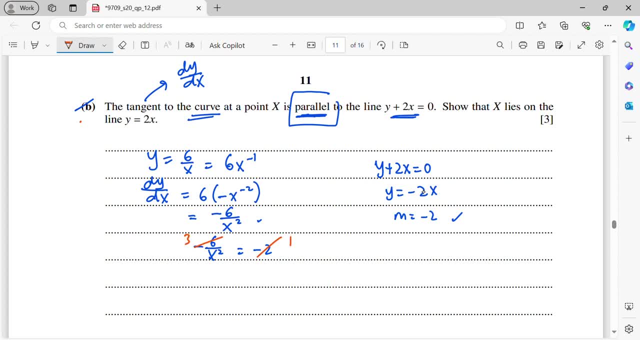 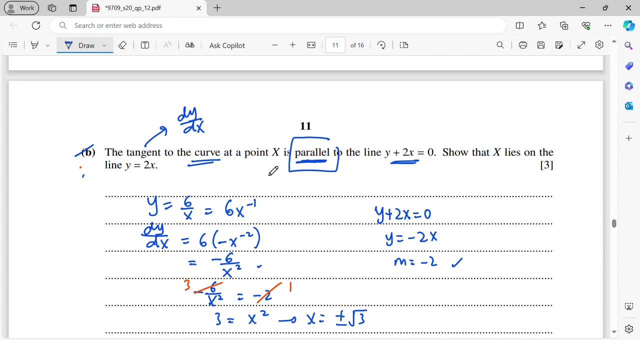 and minus 6. cancel off becomes 3. here is 1. you divide the whole equation by minus 2, so here I'll get 3 equals to the x squared. move up. therefore, my X will be plus minus square root 3. okay, so now show that the point X lies on this. 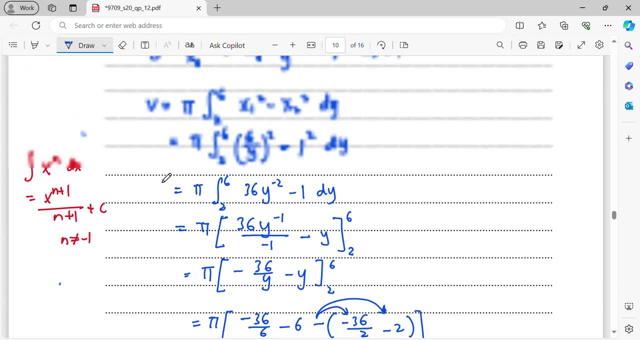 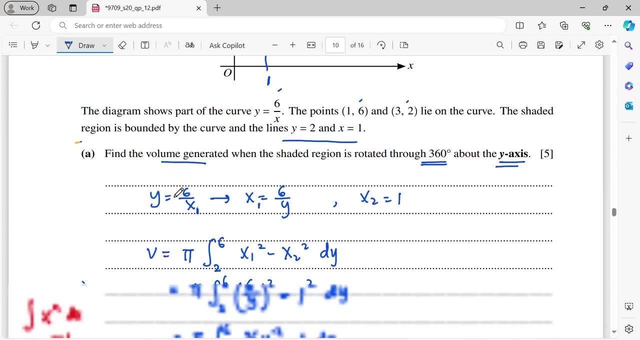 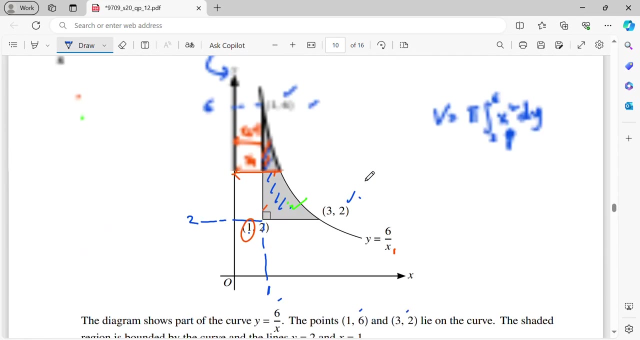 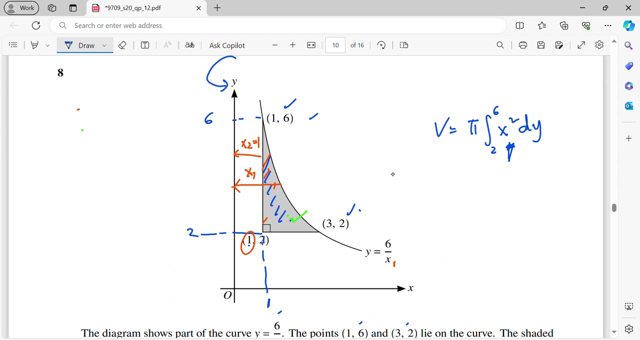 line. okay, so let's check your X from the graph. okay, from the graph, the line is: y equals to 2 negative 2x. so at X. so now from here. okay, from the graph you are showing, you are given that the graph. okay, this graph, the. it is on the. 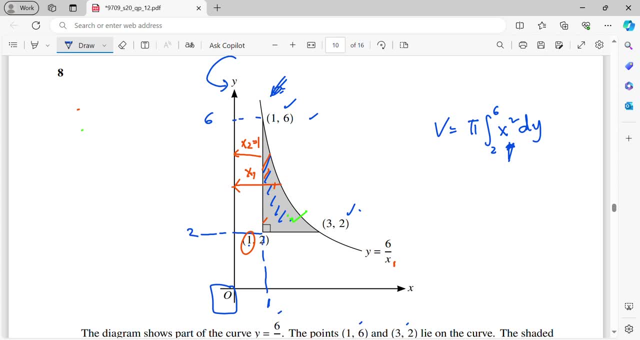 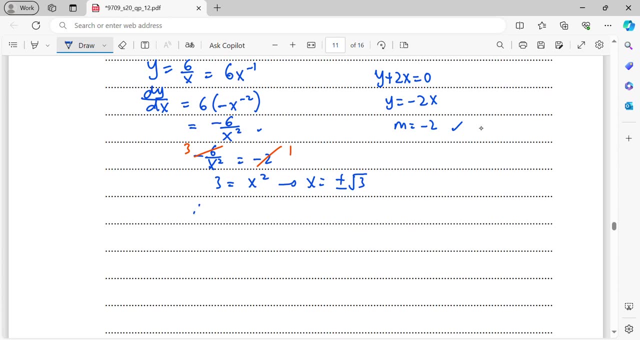 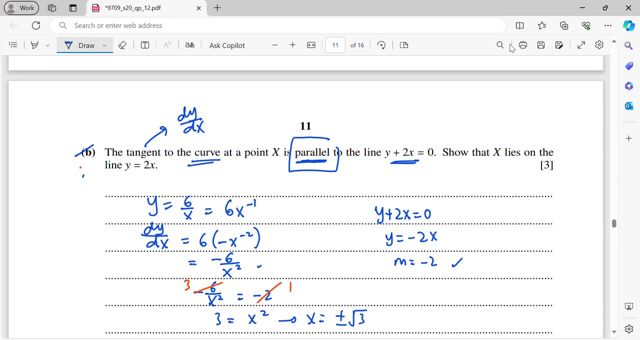 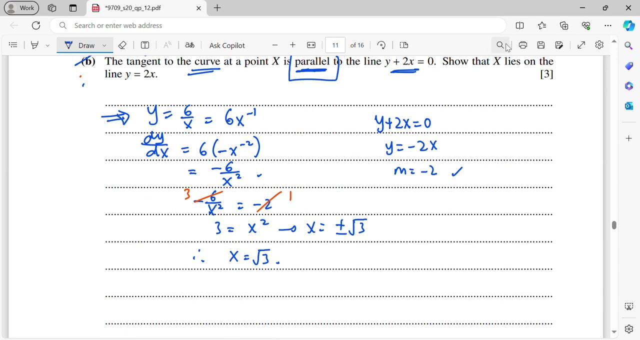 right side of the 0. okay, that means we will just take the positive X. okay, so therefore your X is square root 3. now I need to find out what is my Y first. so this substitute back into the curve equation, right? so when X equals to square root 3, my Y is 6. 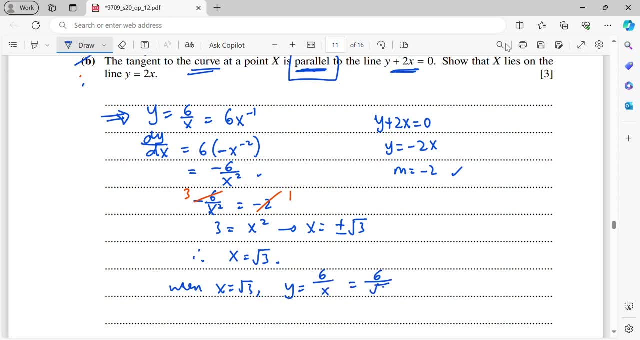 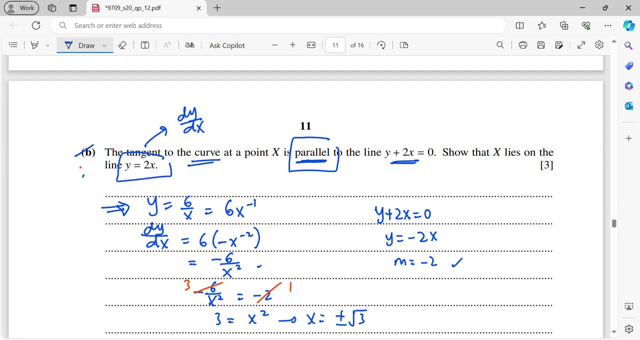 over X. that means it's 6 over square root 3, the 6 over square root 3. this 6 is basically square root 6 times square root. 6, then over square root 3, and now I need to show that it is in this: Y equals to 2x, so which means the square. 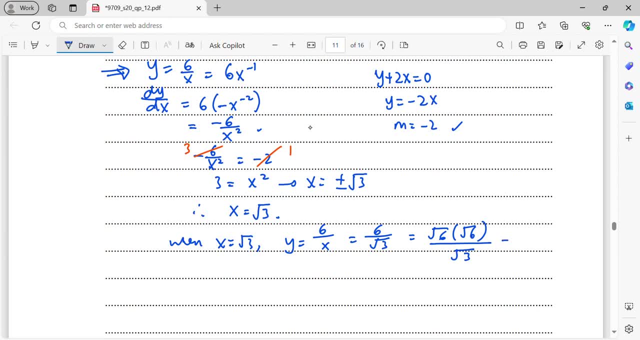 root 6. I need to simplify, okay. so square root 6 is basically square root 3 times square root 2. there another square root 6. you can probably just square it, okay, or if not, you can just write: square root 3, square root 2. so all these are multiplication. 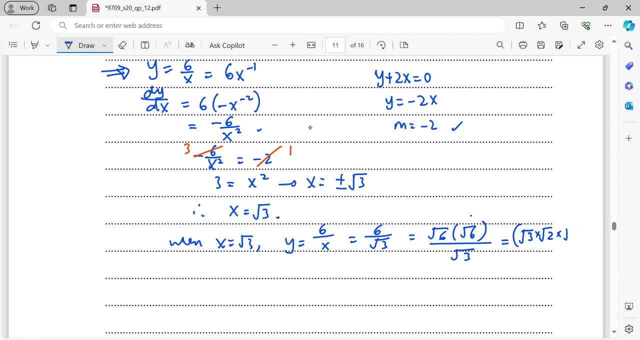 of y is 2x squared 3. so for x, square root 3 you are. you should be really careful of this here. okay for y, then from here I will cancel off the square root 3. okay, then here I will be getting equals to square root 2 times square root. 2 is 2, square root 3: right. so that means from here, when x is square root 3, y is 2, 3, which is 2, square root 3, which means, when I write it in a real shape- Look at the bottom here, when y is 2, where the second algebra a is what moment you write, y is 2. let me let 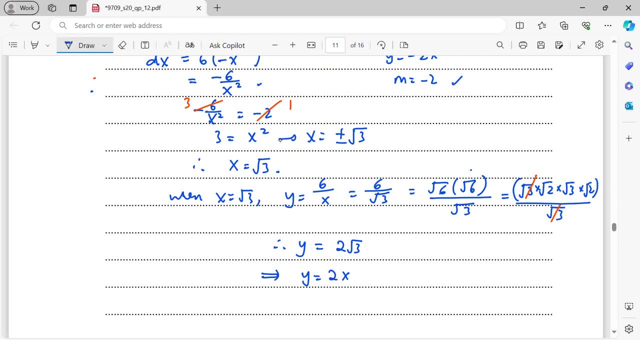 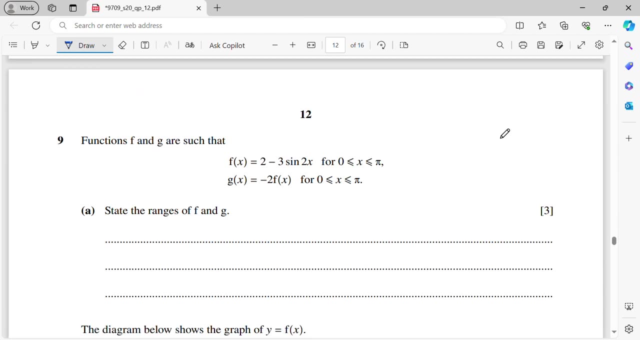 your y is 2x, so x lies on, y equals to 2x. so that is how i prove it. okay, next question, number nine: given fx and gx, so state the ranges of f and g. so now look at here: your fx is 2 minus 3. sine 2x x from 0 to 2 pi. so now i will write down here first when sine 2x. 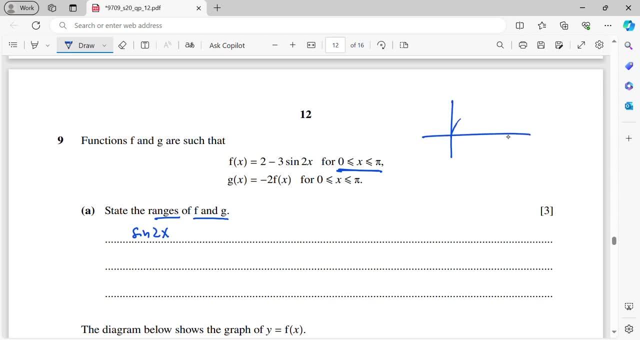 from 0 to pi. let's say you refer to the sine graph. this is sine 1x, sine 2x, from 0 to 2 pi. right, so here pi, this is my sine graph. but then when you look at the interval here, 0 to pi- 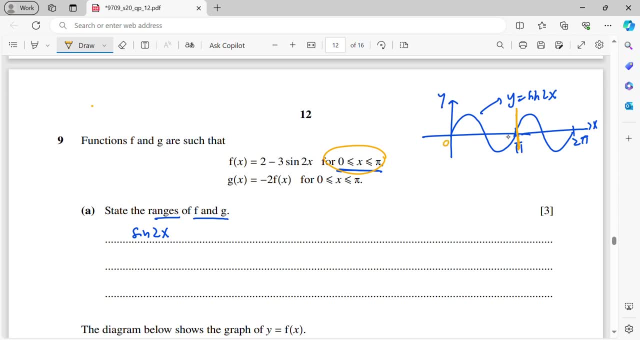 it means that we will just consider up to first part, so 0 to pi. so i know that maximum is 1, minimum is minus 1.. okay, so now i will write: sine 2x will be in between minus 1 and 1, so minus 3. sine 2x means your times minus. so you have to change the inequality sign. 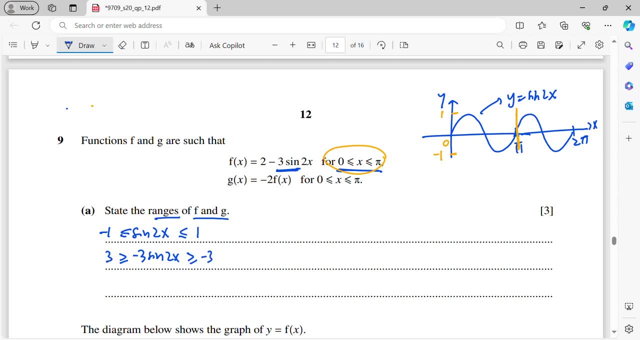 so all numbers times minus 3, so it will be 3 and minus 3 here. then after that this is basically same as three sine two, x plus two. so now i plus two. so when you plus two for the middle term, the other two terms must plus two. so means this is three plus two, here is minus three plus two, which means 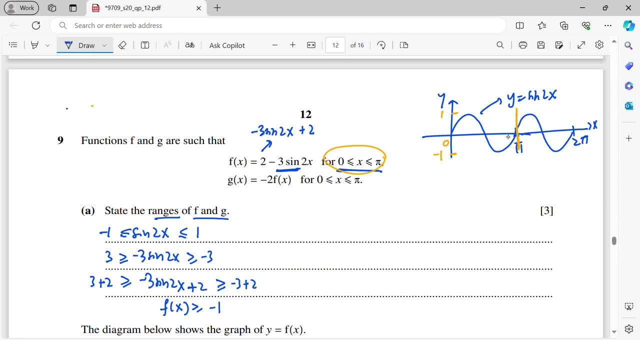 now this is fx is greater equal to minus one and less equals to five. so then from here i can say that my fx, so my fx, when you read from fx to the right side, it will be greater equals to minus one and less equals to five. when you read to the right side, left side- so from here i know that my range 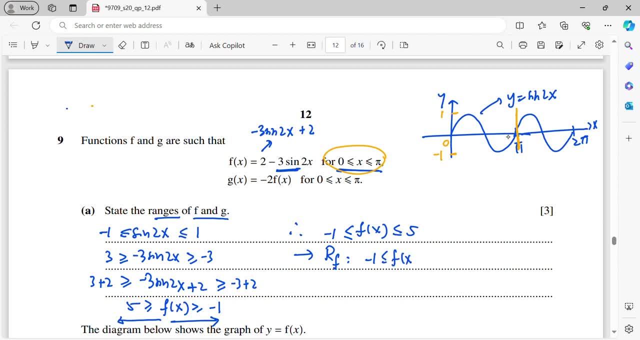 of f is basically between minus one and five inclusive. so for the gx equals to negative two, fx. right, so now you just have negative two. that means your gx. when you times negative two from here, all right, or probably, i just write negative two, x. so when times negative two to the inequality refer to this, you have to change the sign of. 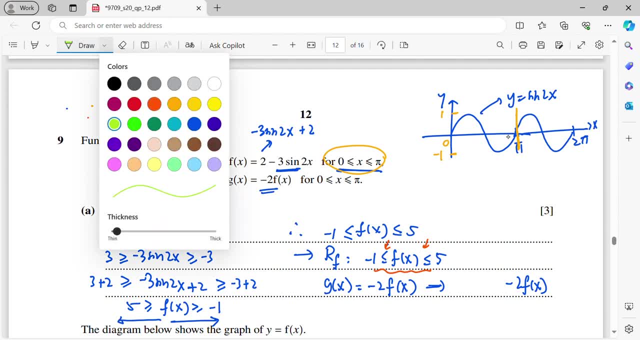 the inequality must remember that. so that means i will change it to critter equals two. okay, and here critter equals two. so minus one times minus two, minus one times minus two is two. then five times minus two it will be minus ten. so then i will change this back to gx. so gx. 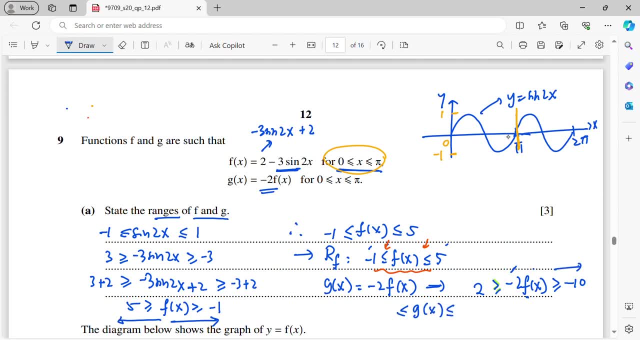 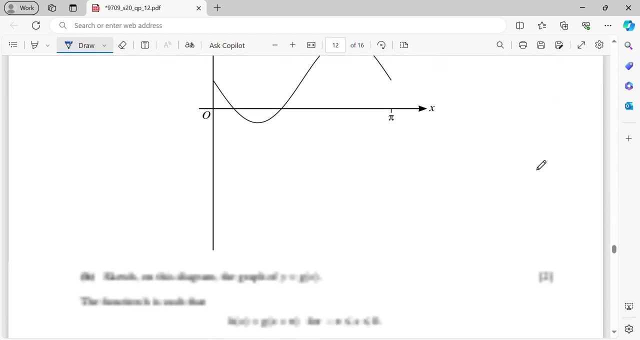 less equals two. okay, so when this is gx, you read like that: greater equals to minus ten, so greater equals to minus ten, and then this is two. that means this is your range for gx. so done for range for f and g. now the diagram below shows the graph of y equals fx. okay, this is graph sketch on this diagram, the. 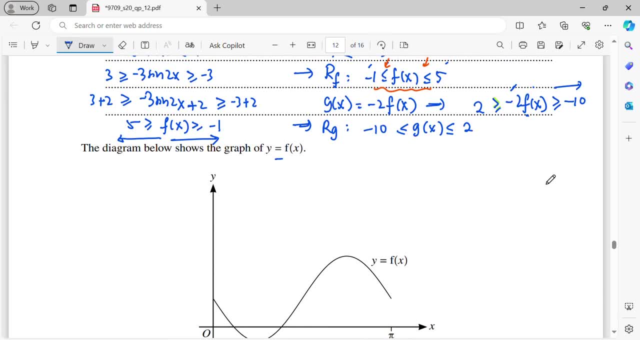 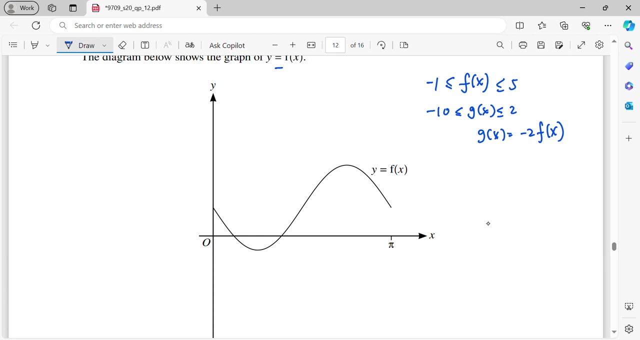 graph of y equals to gx. okay, so now we know that. okay, just now, your fx in between minus one and five. now the gx in between minus ten and two. okay, now your gx is negative two fx. okay, which means this is my minus one and this my. this is my five. that's why fx is in between minus. 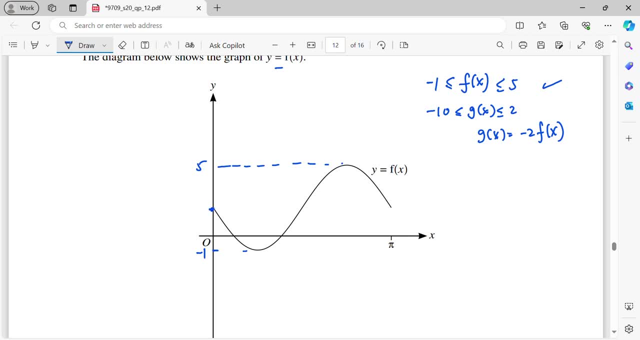 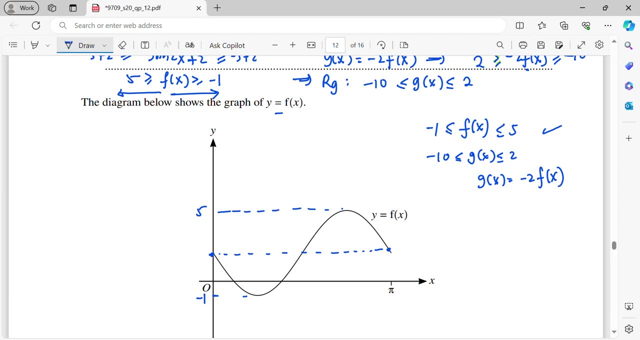 one and five. so i need to find out what is this value? okay, for your info, this value, when the x equals to zero and pi, the y will be the same. so now i will rewrite: my fx is two minus three sine two x. so when my x equals to zero, i'll get two minus three sine zero. sine zero is zero. 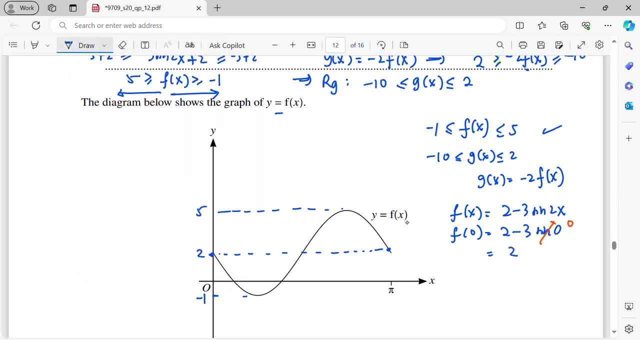 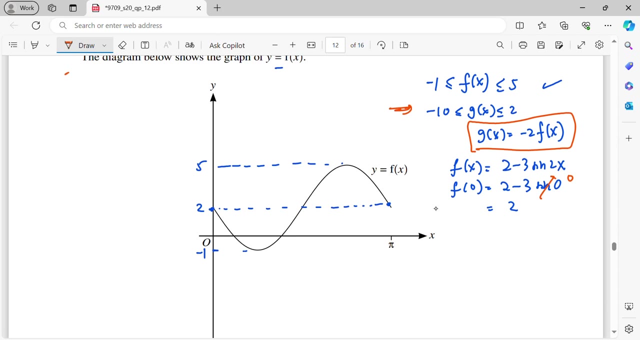 therefore, i will just get two. so i know that this is two. so now, when you multiply with minus two for this fx, right, for this function, you need to multiply minus 2 to the fx. now here, firstly this 2. okay, so i will mark probably: here is minus 2, here is minus 4.. 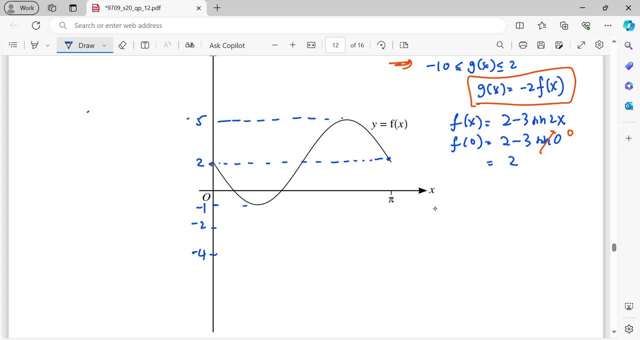 okay, then this 5 becomes minus 10.. that means here now i will be getting this from 2- change to minus 4.. this is minus 1.. so minus 1, you is minus 2, it becomes 2.. okay, this point is at 2, so it becomes minus 4.. 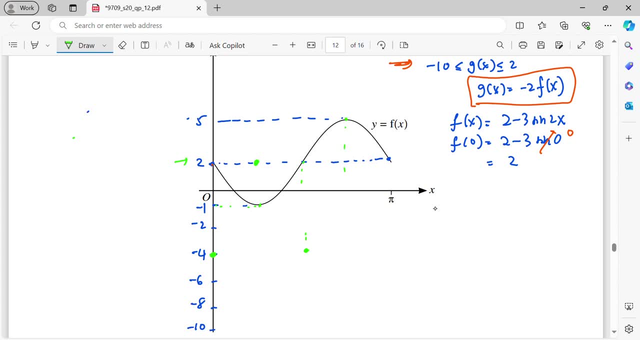 so maximum points: from 5, it will be negative 10.. so roughly here, right? it's just a reflection, basically. and then, uh, okay, this point at first, 2 now becomes negative 4.. so now you just join, right, so it will be touching same points. so the graph will be. 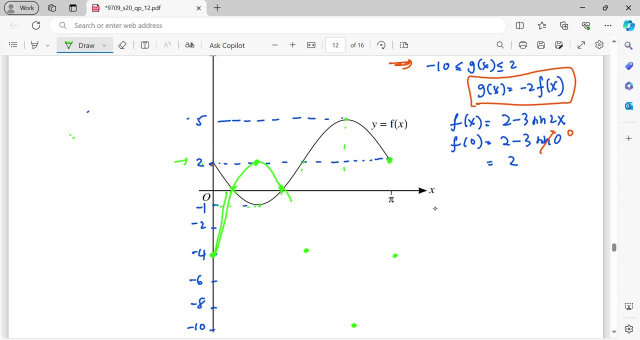 in this shape. so we'll get curve constant from diagonal to the base. so 4 minus 3 is the slider and 9 is the length. ok, this will be the graph. so this is the graph. graph, all right, so this is our y equals to g x. 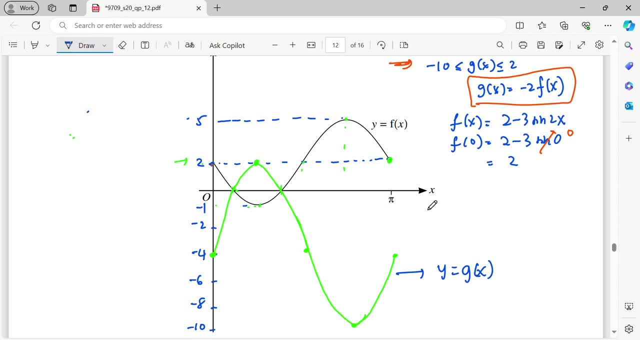 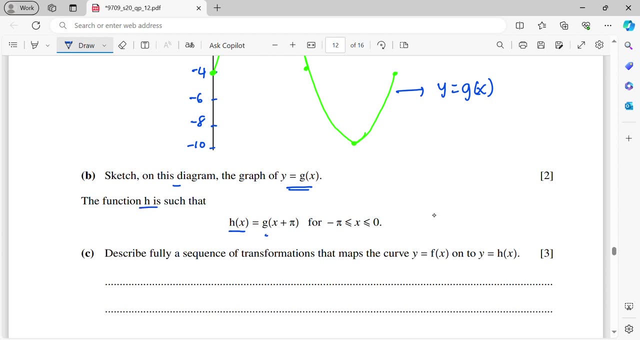 okay, now the function h is such that hx is g of x plus pi, where the x is between minus pi and zero. so now describe fully a sequence of transformations that maps fx onto hx. okay, so now your fx to gx is negative to fx. right, i will say: okay, um. 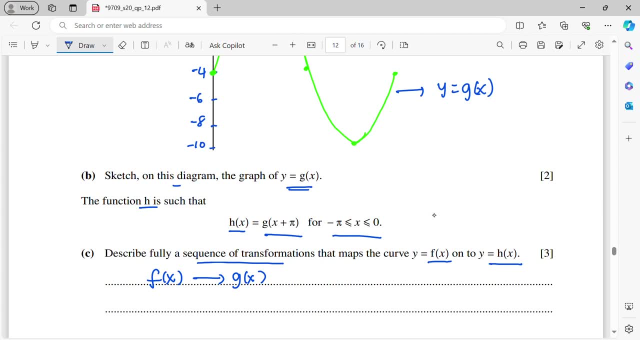 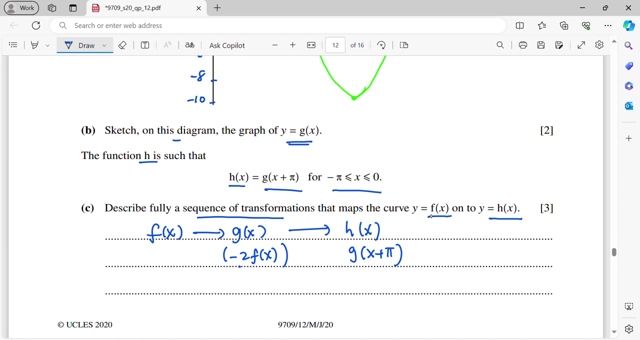 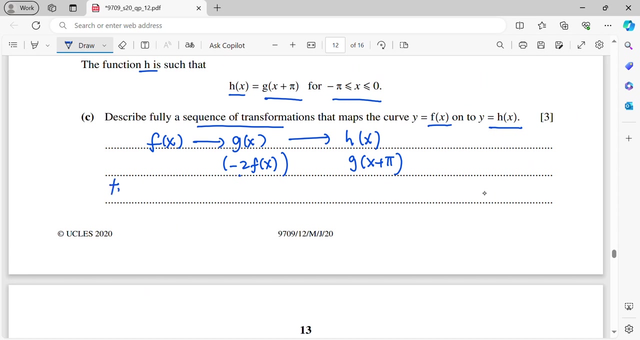 this is negative to fx. then from gx change to hx. so this is g of x plus pi. okay, which means now, firstly to get the gx. that is the reflection, because of minus two, minus two of fx, right, so just upside down, based on the graph, so that means the transformation. 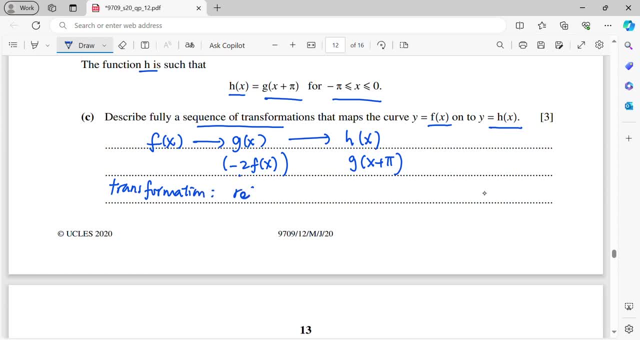 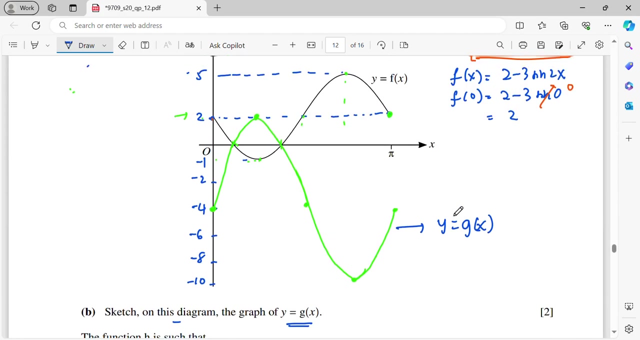 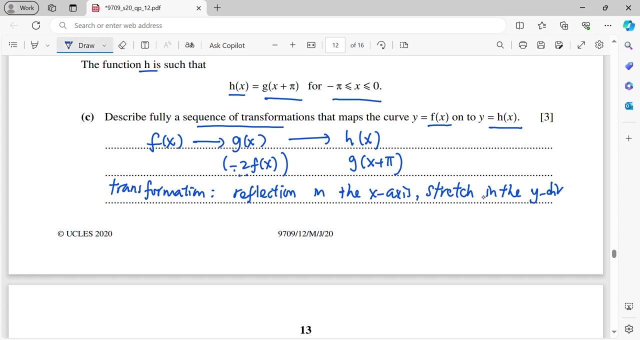 will be reflection in the x-axis. stretch because of the minus means reflection in the x-axis. okay, the two fx means stretch. so stretch in the y direction because the changes will be on the y values right, all the y values changes are changed. so in the y direction with scale factor. 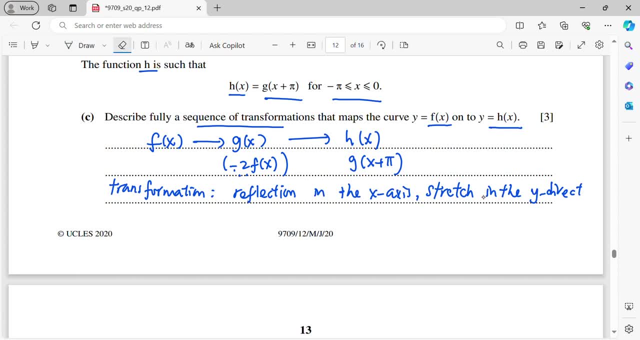 two. the dimension of the direction will be student. all the y values change or the y value on the y value starve change. so that means if student learnt add each or all, conv führt feito. two. the ga in one function or combination is cliche. the sum of values change so that the 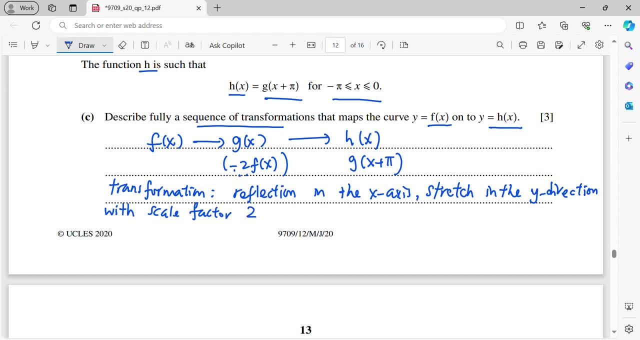 all Basket 것을, okay. so we found the gx here, and then followed by hx is gx plus pi. so when you let this x plus pi be zero, that means your x is minus pi. that means this is a translation okay of the x is minus pi unit. so here will be followed by translation: x is minus pi unit and then y: no change. 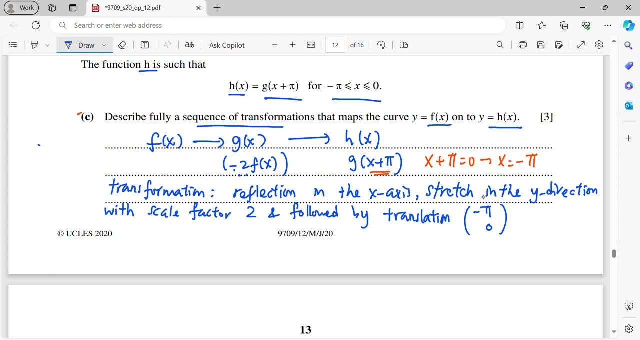 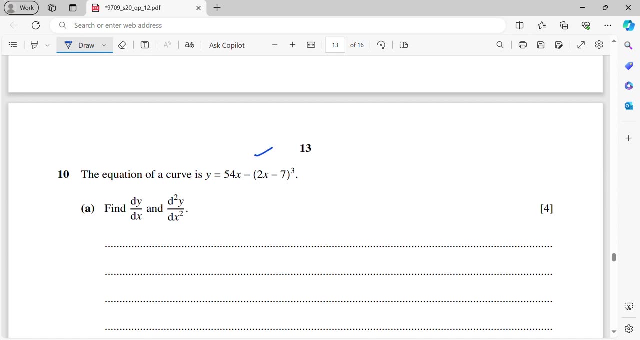 okay, so that's the transformation from fx to hx. okay, now for question number 10. given the curve equation, 5 dy dx and the second derivative, so your y is 54x minus 2x minus 7 cube, so my dy dx. okay, we have a formula over here. 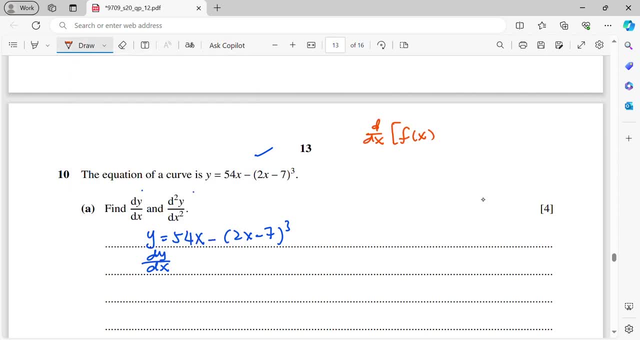 differentiate fx, degree n, that is n fx, to the power of n minus 1, and then differentiate fx is f prime x. so from here i will get 54. then bring down the 3, so 3. 2x minus 7, degree 2. so now when i differentiate 2x minus 7, it is 2. so this is going to be 54. okay, 3 times 2. 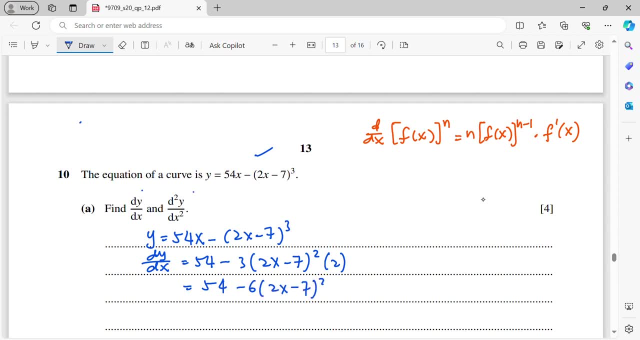 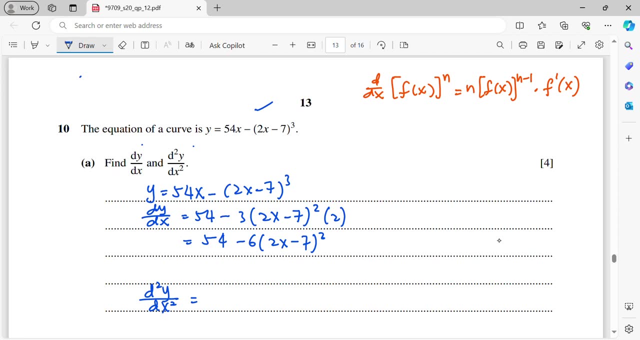 6. so minus 6 of 2x minus 7 squared, that is my dy dx. now for the d square y over dx squared differentiate for second time. so first term: there is no x. that means you get zero. so now just copy back the minus 6, the 2 will be moved down. rewrite 2x minus 7 degree becomes 1. 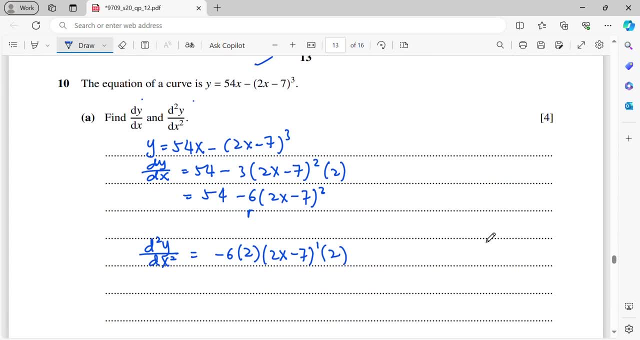 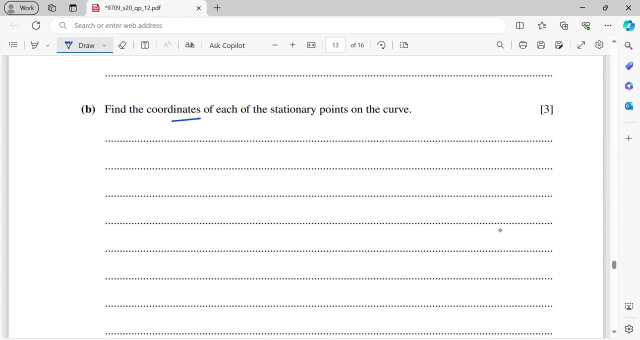 and differentiate 2x minus 7, that is 2. then you will be getting minus 24 of 2x minus 7. so that is the solution of part a. now b: find the coordinates of each of the stationary points on the curve means that: 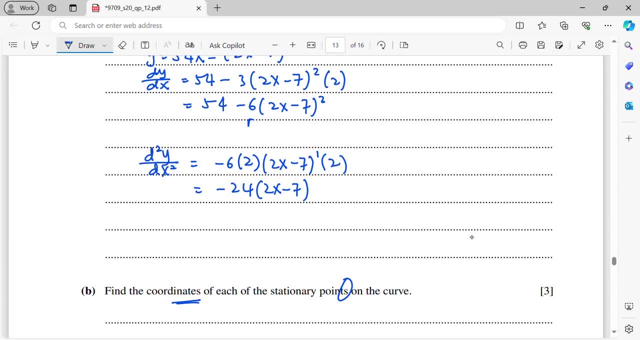 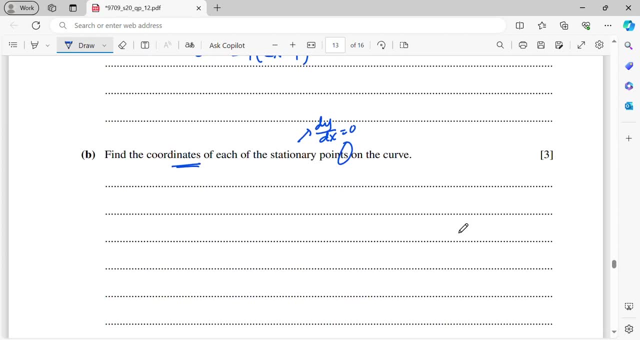 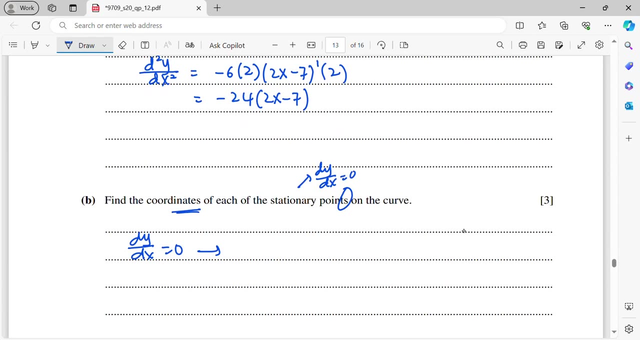 you will be getting more than one point. so the stationary points happens when dy dx equals to zero, right, so i will let this be zero. the solution of part a is 2 square root of x square. how much distance betweenieli and x square? here, mà you don't change the Sahara, andetztamən. 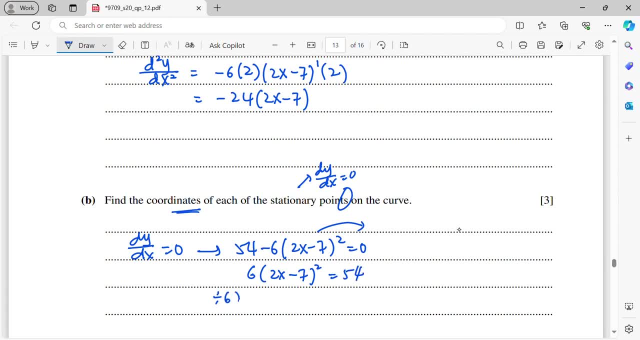 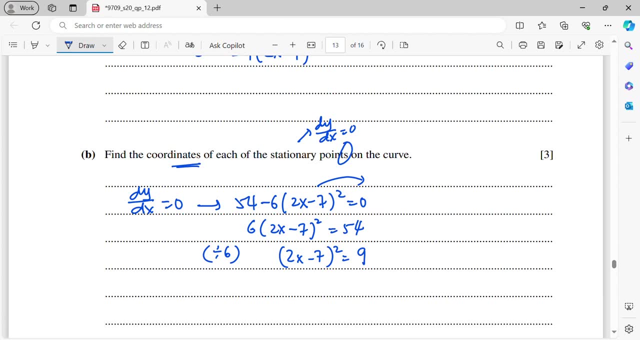 f, 2 andí. you are all right. then now to simplify this, i will just move this term to the other side and divide the whole equation by 6. i don't want to do expansion, so i'll get 2x minus 7 squared equals to 9. then now to eliminate the squared, it would be plus minus square root of y equals the times we do an evening. then divide the whole equation by six. I do want to do expansion, so i'll get 2x minus 7 square equals to nine. then now to eliminate the square, it will be plus minus school root. then you will get 2x minus 7. square equals to 9, it would be plus minus square root of the곳 of y equals to part A of the Mason system. numerically, returning here protected the answer from e-Nufile, you'll get 6x. that is to return crimes. 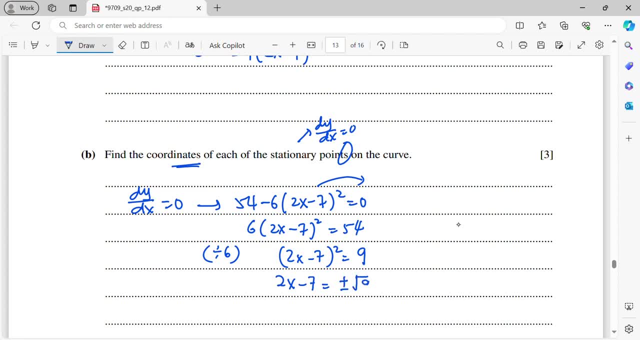 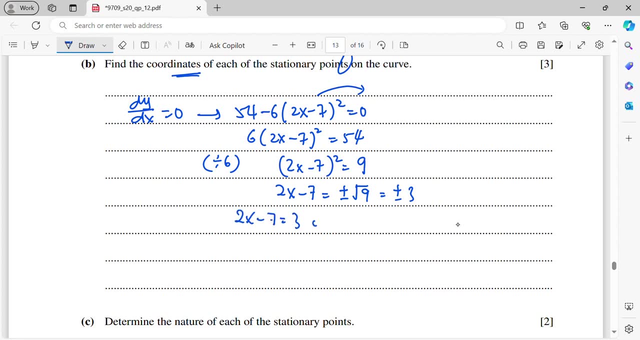 9. this is plus minus 3, so here i will get 2x. so now 2x minus 7 equals to 3, or 2x minus 7 equals to minus 3.. so now my 2x equals to 10, hence my x is 5 and the other one, 2x, equals to 4. 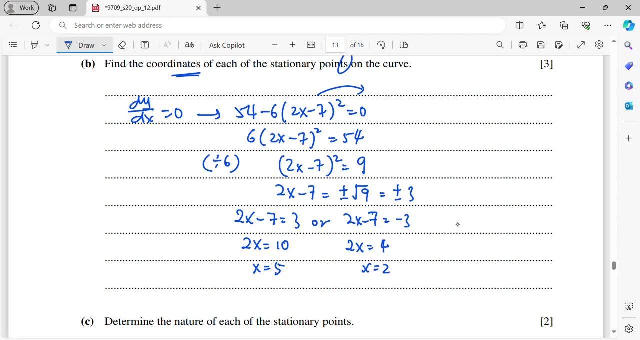 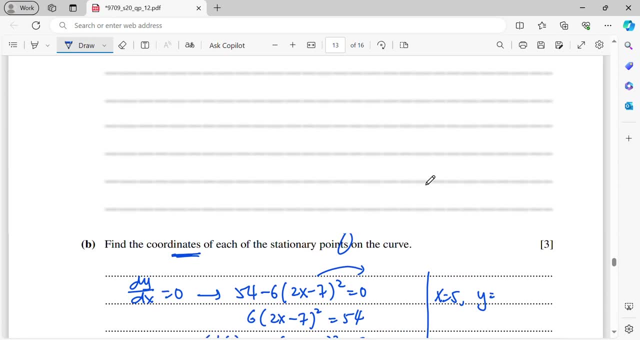 my x equals to 2, i get 2x. but then now question: asking for coordinates means when x equals to 5 i need to substitute back into my y to get the y coordinate. so my y is 54x minus 2x minus 7 cube. 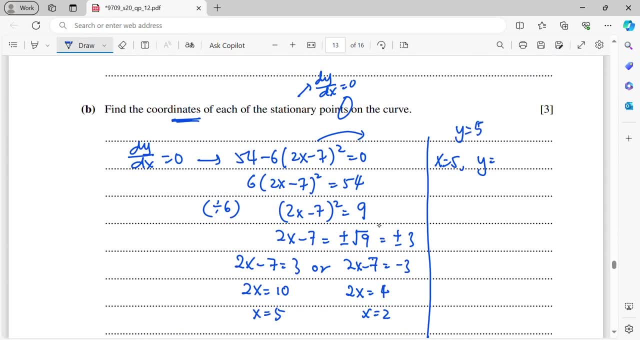 so y equals to 54x minus 2x minus 7 cube. so now just replace 54 times 5 minus 2 times 5 minus 7 cube. that is going to be 2 4 3. so when x equals to 2, my y is 54 times 2 minus 2 times 2 minus 7. 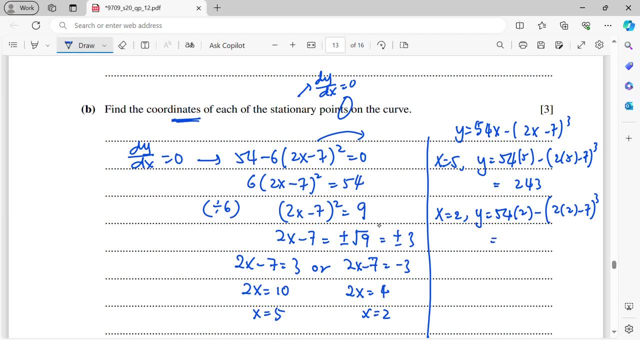 then you cube it and the answer is going to be 1, 3, 5. therefore i get 2 points, so stationary points, with coordinates 5, 2, 4, 3, and the other one is 2, 1, 3, 5. so that's all for the part b. 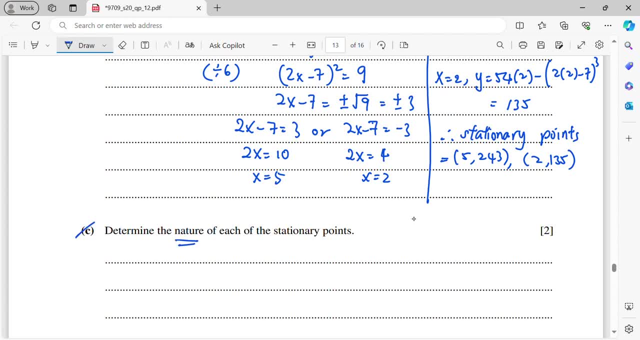 and now part c determine the nature of each of the stationary points. nature means maximum or minimum. so if the second derivative is greater than zero, that is minimum. but if let's say d square, y over dx squared is less than zero after you replace the x, that is maximum point. 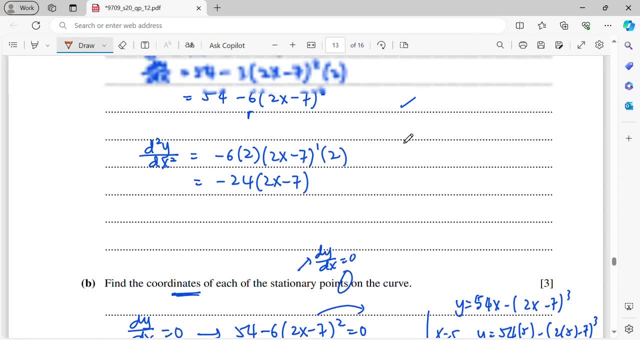 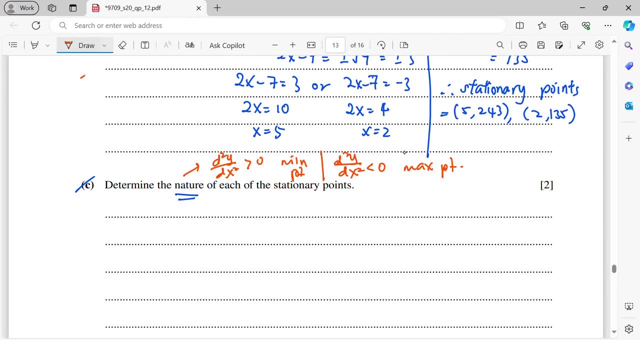 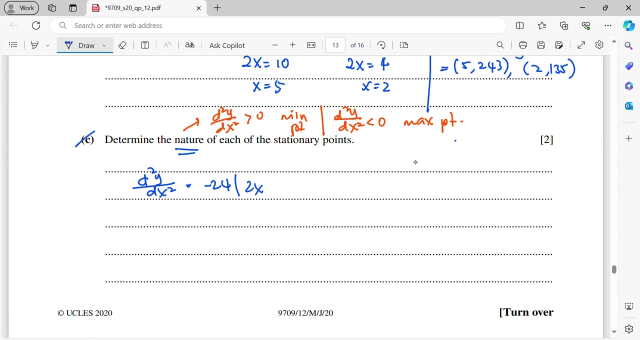 okay, then now i refer to my second derivative expression: minus 24 times 2x minus 7. so from here you will get d square y over dx squared is minus 24 times 2x minus 7, so at x equals to 5 according to the point c. 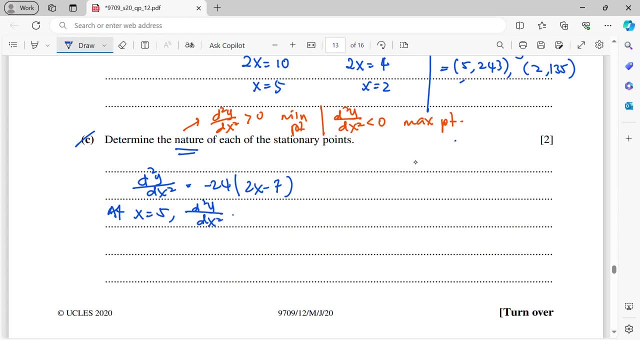 your d square y over dx squared is 24 multiplied with 2 times 5 minus 7. so this is negative: 72 less than 0, then at x equals to 2. the other point, your second derivative, is negative 24 times 2 times 2 minus 7. 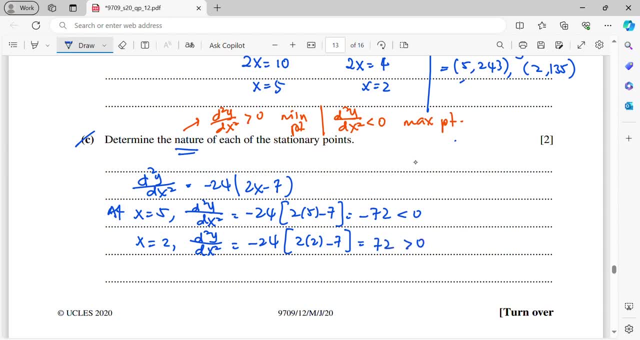 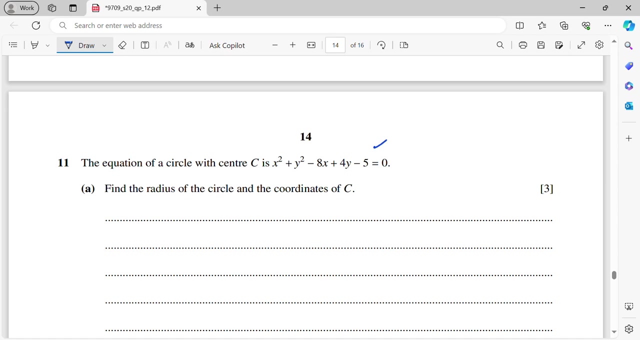 then this is going to be 72 greater than 0, so which means 5, 2 for three. this is maximum, this is minimum. it's a maximum point, okay, and the other point is a minimum point. all right, so done for this question, okay. question 11: the equation of the circle is given for the radius of the circle and the 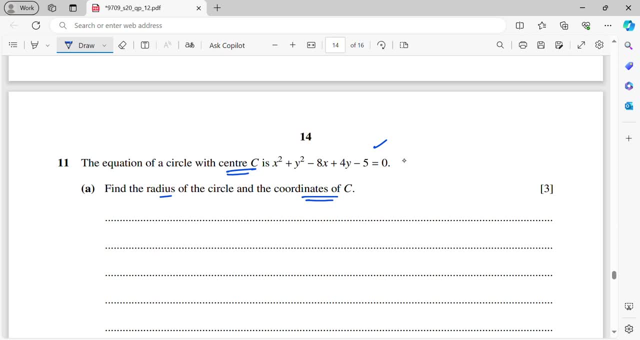 coordinates of c, c is the center. so now here i need to group the term with the x and the term with the y, because our formula for circle is basically x minus a square plus y minus b square equals to r squared. so the a and b is the center coordinates. right, then the r is the radius. 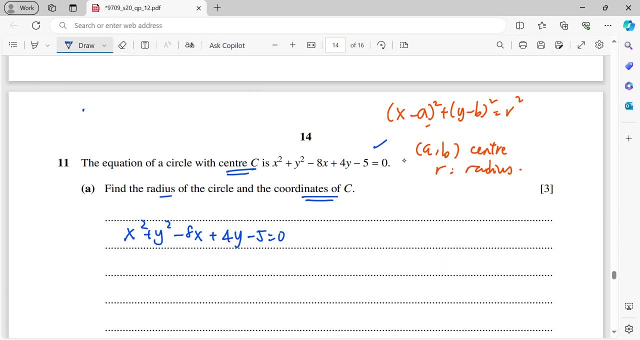 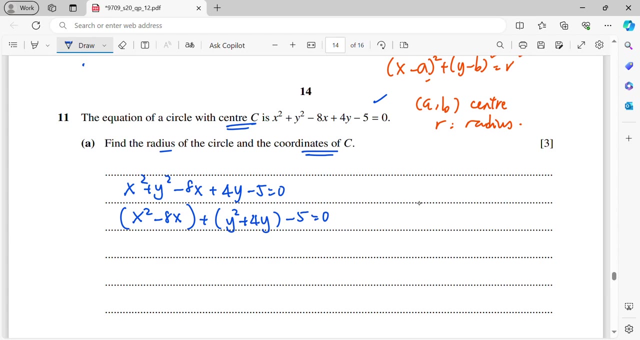 so to get this form you have to perform completing the square method. so, which means now i rearrange first, then the minus 5. i will just keep it on the left side, or you can move to right side, up to you. so, from completing the square, make sure the coefficient for x squared is positive one. and 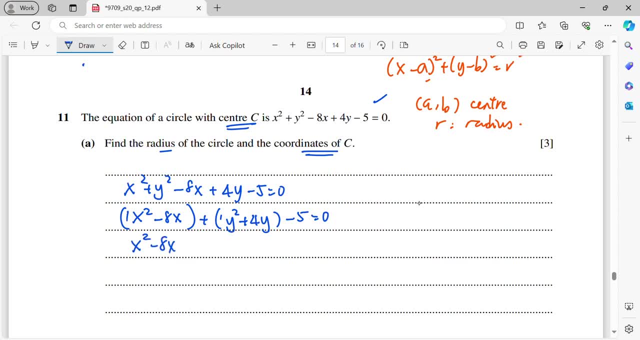 the y square is positive one. so now i will rewrite and then add two more terms. this is for x, so for the y, still the same. rewrite both terms and then plus bracket square, minus bracket squared and then minus five equals to zero. so the term inside the bracket, it should be half of the coefficients of x and also. 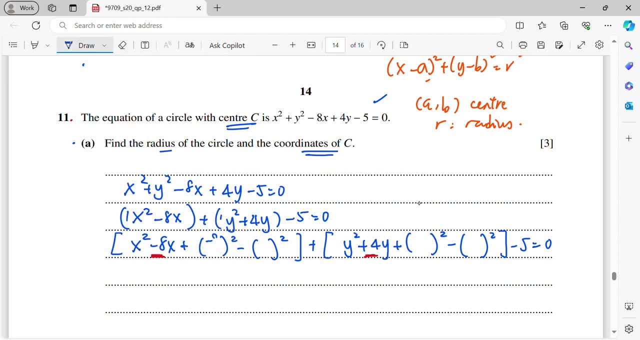 y. that means that is going to be minus 8 over 2 for the first term. for the y will be plus 4 over 2. so that means that is going to be minus 8 over 2 for the first term and for the y it will be plus 4 over 2. for the y it will be plus 4 over 2. so for the y it will be plus 4 over 2. so for the y it will be plus 4 over 2. sub Focus two gives you that shortcut because you say the term is negative for the y. this is so. i take over to the y, even a plus 4. we give you that circle minus 5 into 4 using the line- and we did require an extension to me for the super sırita to measure that. 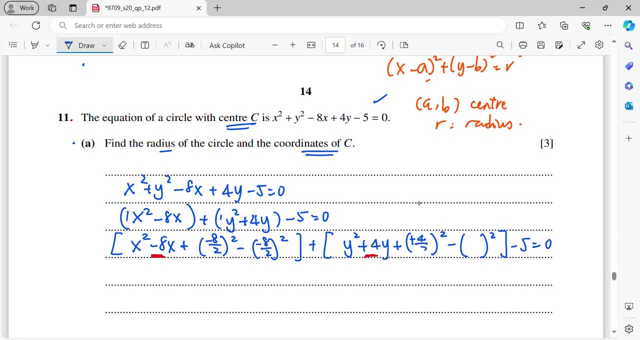 the first term and for the y it will be plus 4 over 2. okay, so for the first bracket i will group the first and third term. okay, here i also group the first and third term. so when i group i will get x now from the second tick in the first bracket. 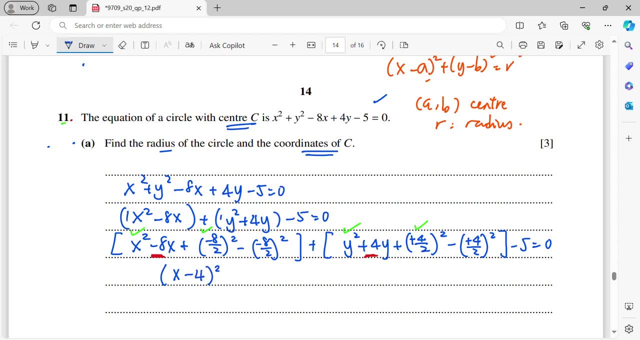 it will be minus 8 over 2, that is minus 4. okay then, minus minus 4 squared, and plus in the second bracket, y square, and plus 4 over 2 will be combined. it will be y plus 2, because 4 over 2 is. 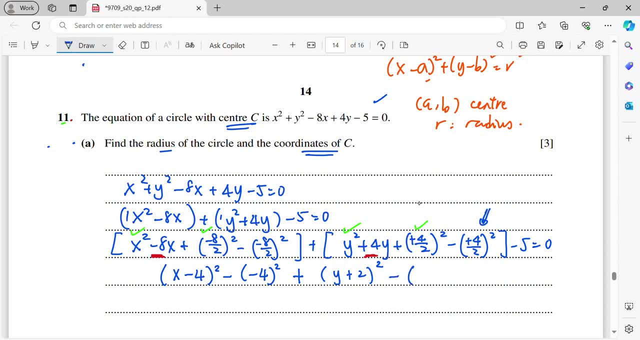 2 squared, then minus the. this term is basically 2 squared, then minus 5 equals to 0. so now combine the first and third term. okay, just rewrite these two terms. then now this is basically minus 16. okay, so i will just write here: minus 16, and then followed by: 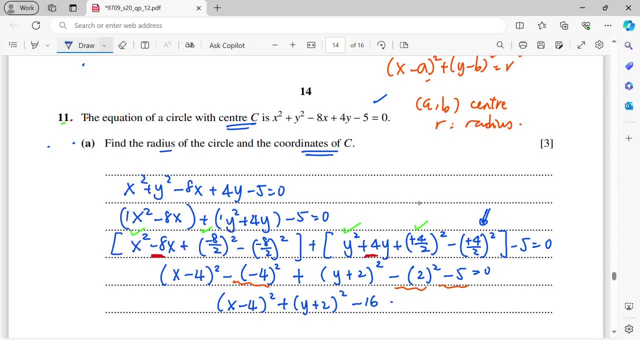 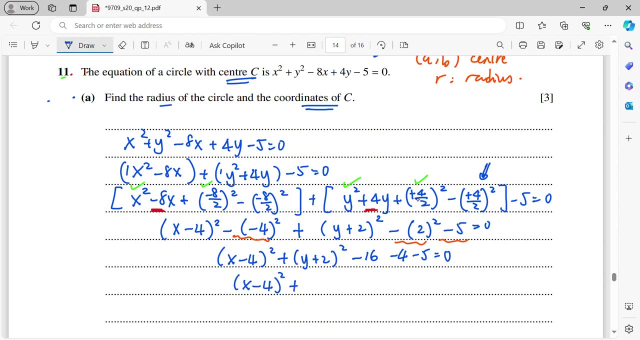 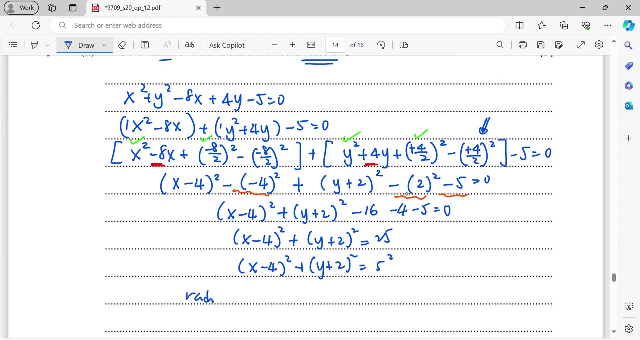 minus 4 and minus 9 minus 5. therefore, i will get x minus 4 squared plus y minus 2 squared equals to 25. this 25, it will be same as 5 squared. therefore, radius is 5. center is with coordinates of 4 negative 2, because the general form this will be y minus. 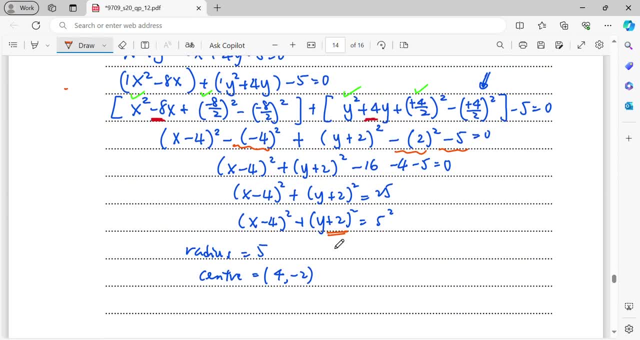 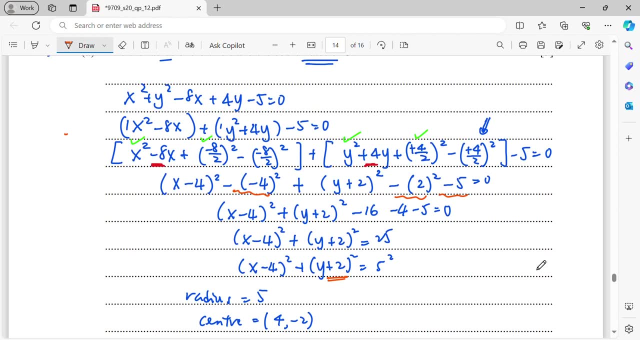 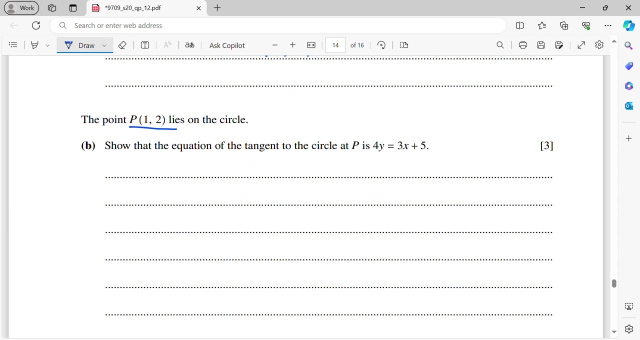 b. okay, so y minus b. that's why now you are getting y plus 2, so the coordinate is basically minus 2. okay, now p lies on the circle, so that the equation of the tangent to the circle as p is this right. let's say, for example: we know that the circle is, with center 4, negative 2. 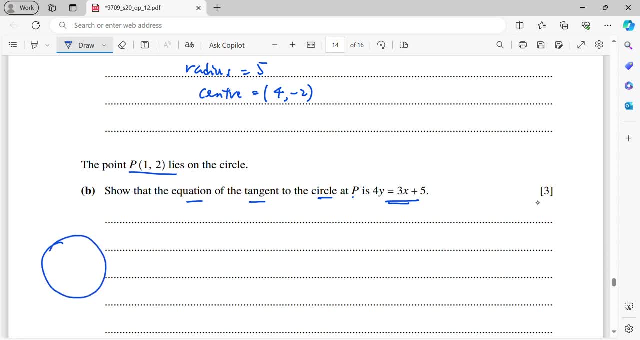 so let's say here 4 negative 2. okay, i simply sketch the circle. this is 4 negative 2, because the radius is 5. so you go up 5 units, okay. or I will say I go up 5 units from the x or from the minus 2, it will be. 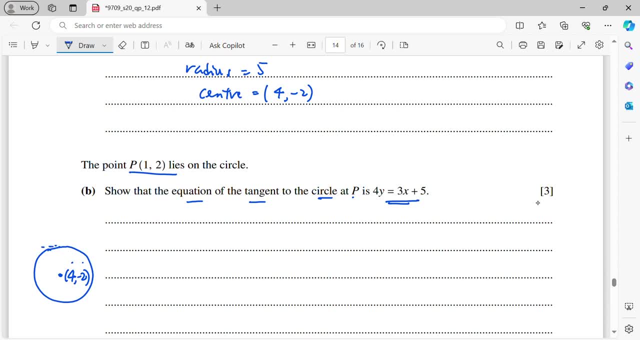 5 minus 2, which is 3. that means here I know that that is 3. okay, and then my 5 units to the left side. this is 3: my 5 units to the left side. that means it will be minus 1 here. supposed to be minus 1 for the x, all right, so which means where? 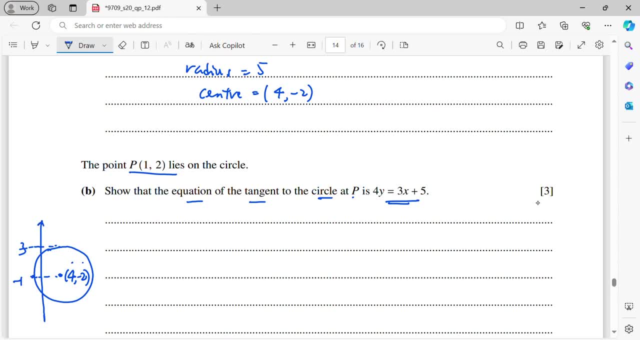 sketch is roughly like that. so this is minus 1, here is 3, this is y, and then my x value. since this is x, this is y, my y, x assist. so this is minus 2. means that, roughly, here this my x. okay, so here is my 0. now the show that the equation of 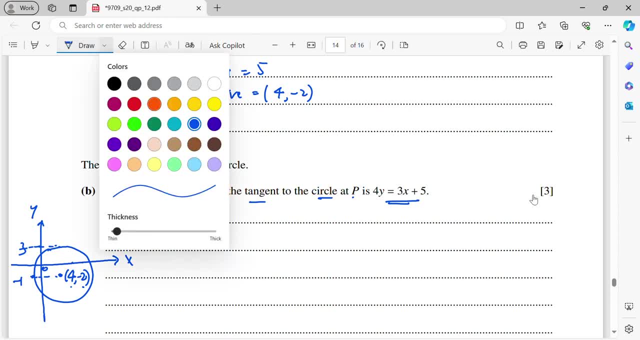 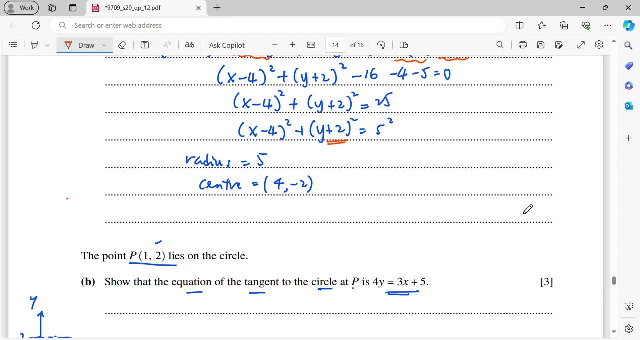 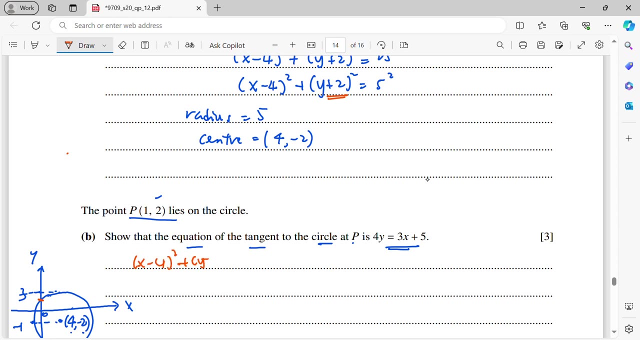 tangent. okay, P 1, 2. so my 1: 2, let's say, here is now let's check at the circle for my x minus 4. right here, x minus 4 square plus y plus 2 squared equals to 5 squared. so I need to find out when, at the x assist, what is the x, what is the y value? 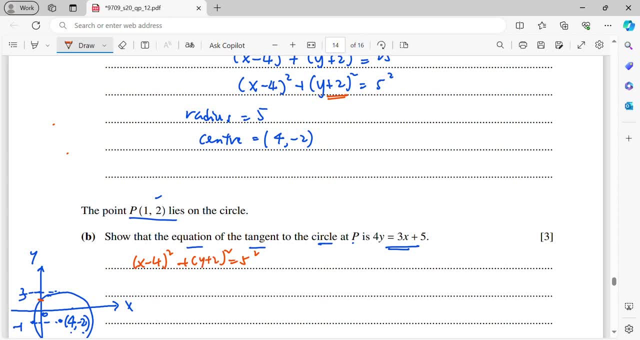 so at this point- because I need to find out where is my 1- 2. so at this point the x is 0, that means I will get. I will get 16 plus y plus 2 square equals to 25. so at this point the x is 0, that means I will get. I will get 16 plus y plus 2 square equals to 25. 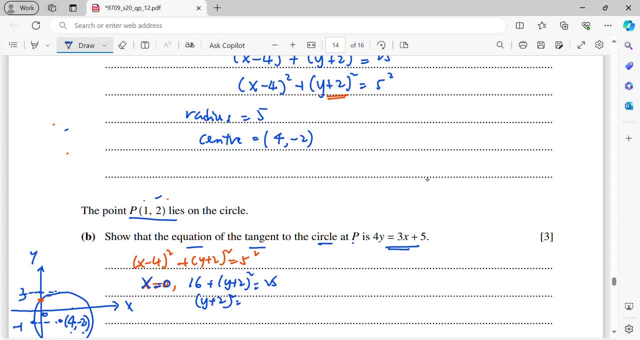 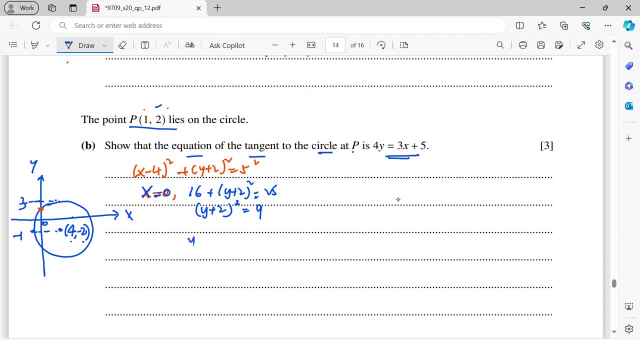 therefore, y plus 2 squared 25 minus 16 is 9. therefore, y plus 2 squared 25 minus 16 is 9. therefore, y plus 2 squared 25 minus 16 is 9. okay, so my y plus 2 equals to 3 or minus 3. 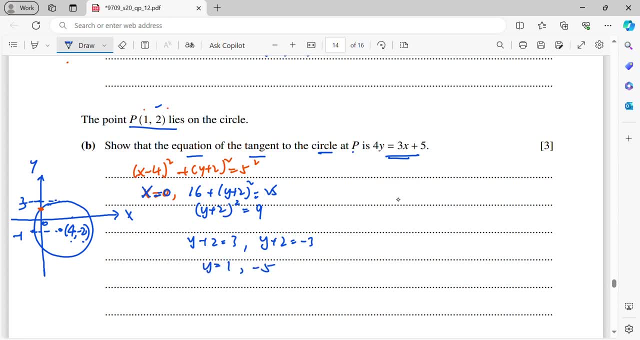 okay, so my y plus 2 equals to 3 or minus 3. okay, so my y plus 2 equals to 3 or minus 3. so my y equals to 1 or minus 5. that, so my y equals to 1 or minus 5. that. 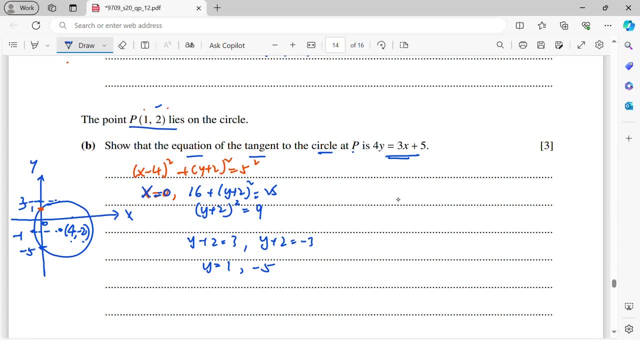 so my y equals to 1 or minus 5. that means: here minus 5, this is 1. okay. so now means here minus 5, this is 1. okay. so now means here minus 5, this is 1. okay. so now I know that my points P is 1, 2, that. 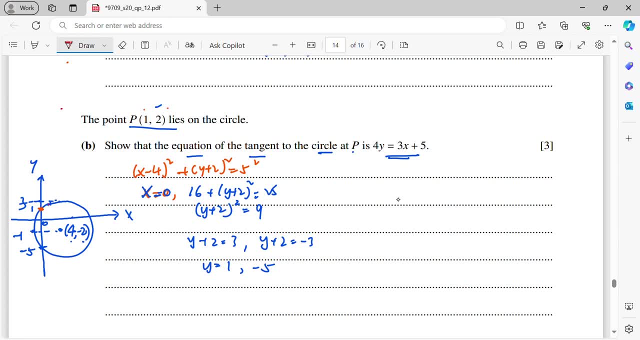 I know that my points P is 1- 2, that I know that my points P is 1- 2. that means it's somewhere here, means it's somewhere here. this is my point p. right then now show that the equation of the tangent to the circle. 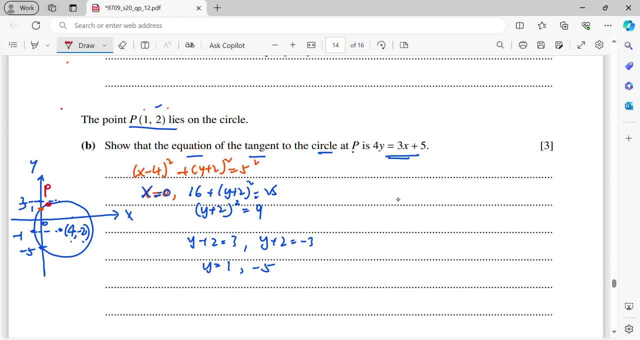 at p is this so equation of the tangent to the circle? that means now you need to show this. all right, this is the line. so from here, what i need to do is: this is a c, here is a c. since this is equation of tangents, means that here must be 90 degrees. okay, so now i need to find out what is my. 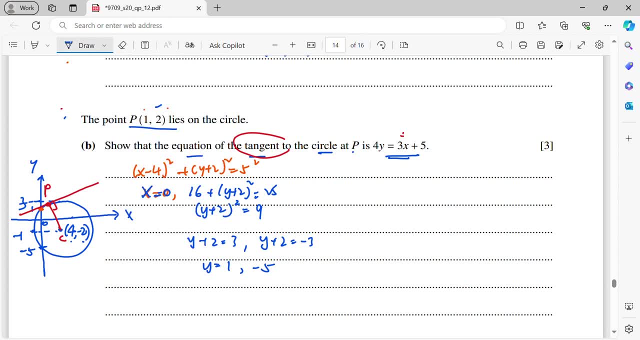 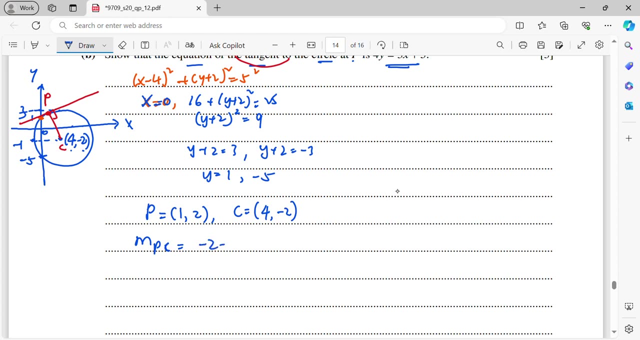 gradient of pc first. so npc: my p is 1, 2, my c is 4 negative 2. so now my npc gradient equals to change in the y. so minus 2 minus 2 over 4, minus 1, that is, minus 4 over 3. so 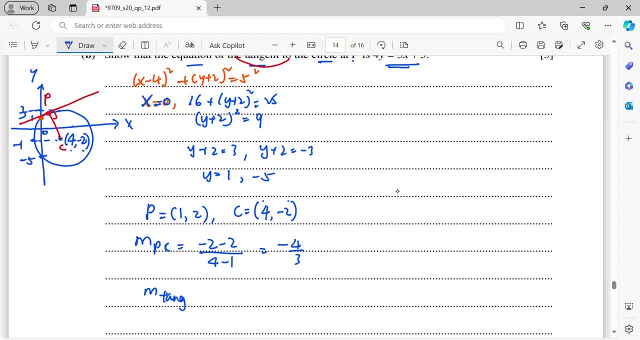 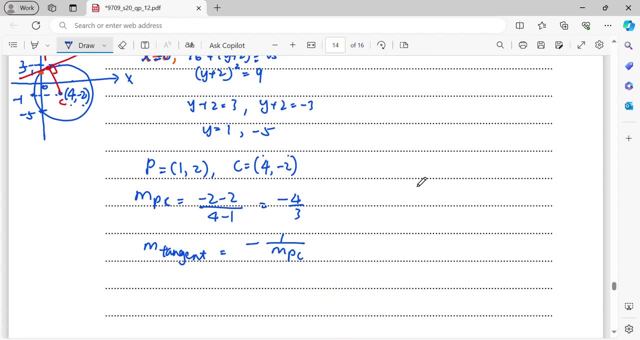 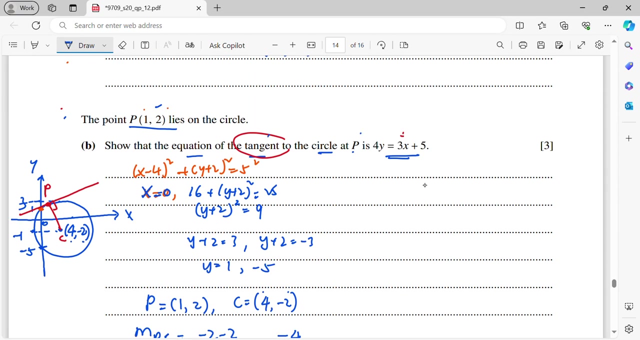 that m tangent, it will be negative 1 over mpc. based on the graph. okay, based on the diagram, that means that is going to be negative 1 over negative, 4 over 3. this is 3 over 4, and now i need to find out the equation of the tangent at points p. so since the points 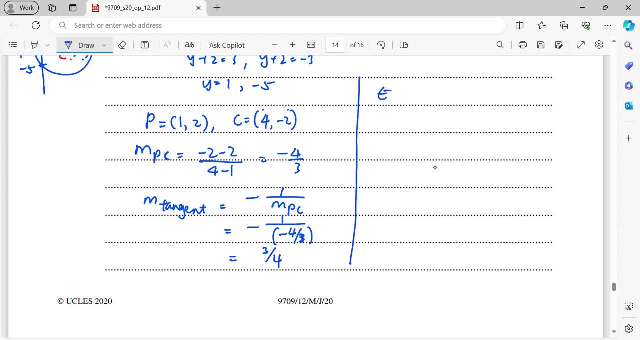 p is given, the gradient is also given. so the equation of the tangent at p, that is, y minus y1, equals to m bracket, x minus x1. so here is going to be y minus the y1 is 2, the m is 3 over 4, the x minus x1 is 1. okay, and now you need to get your. 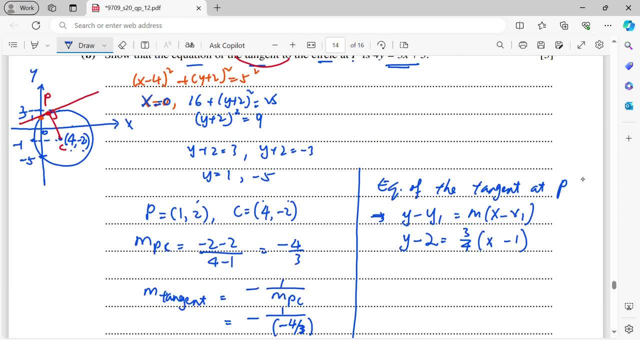 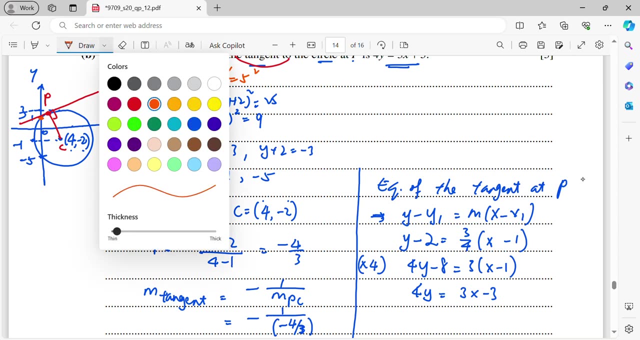 answer in this form: 4y equals to 3x plus 5.. so now times 4 to the whole equation. first, 4y minus 8 equals to 3 of x minus 1. therefore 4y equals to 3x minus 3. when you do expansion, okay, and then at the same time the minus 8 move to. 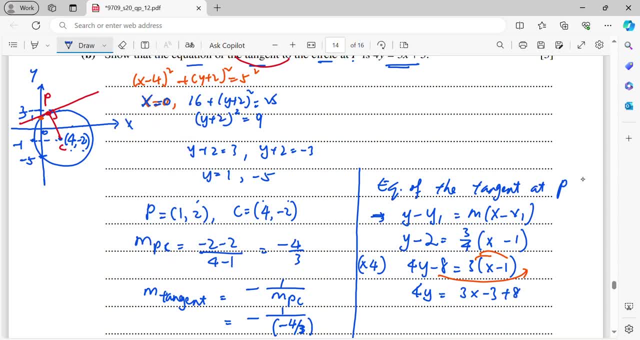 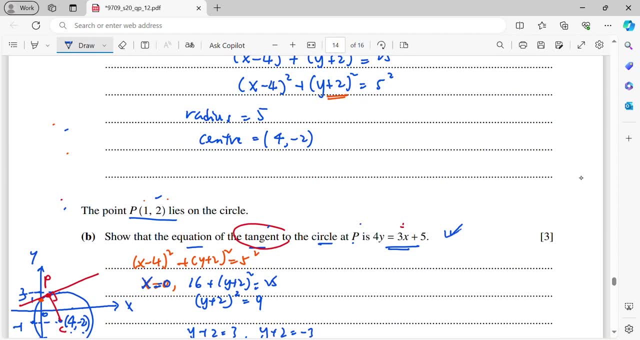 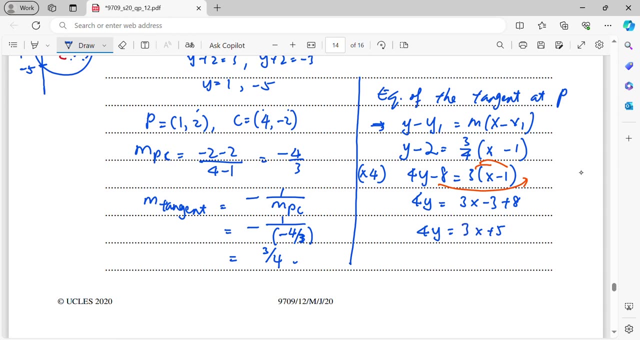 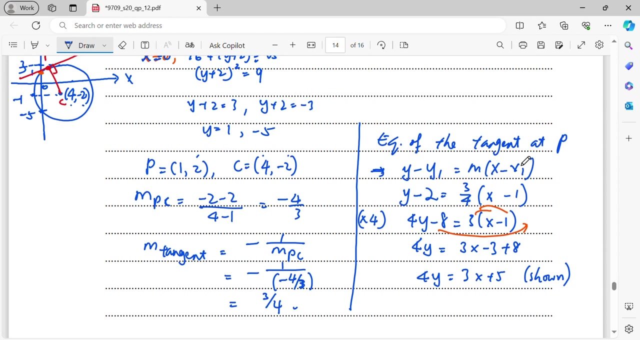 the other side. so here becomes plus 8.. so i will get 4y equals to 3x plus 5. okay, that is the given answer. so here i will change to 3x plus 5. right, so shown. okay, this is my working. 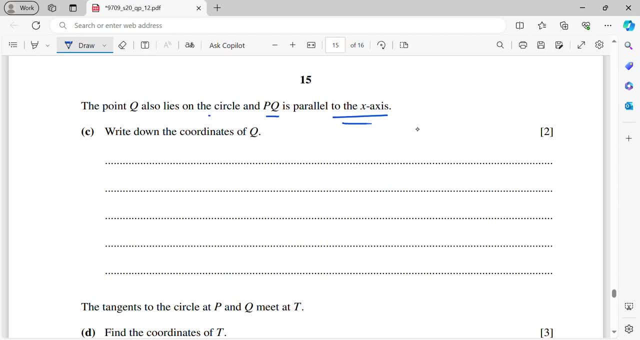 now the point skew also lies on the circle and pq is parallel to x axis. so pq is parallel to x axis means that my q is on the same level. this is my q, so that it is parallel to x axis. so pq is parallel to x axis means that my q is on the same level. this is my q, so that it is parallel to x axis. so pq is parallel to x axis means that my q is on the same level. this is my q, so that it is parallel to x axis. so pq is parallel to x axis means that my q is on the same level. this is my q, so that it is parallel to x axis. 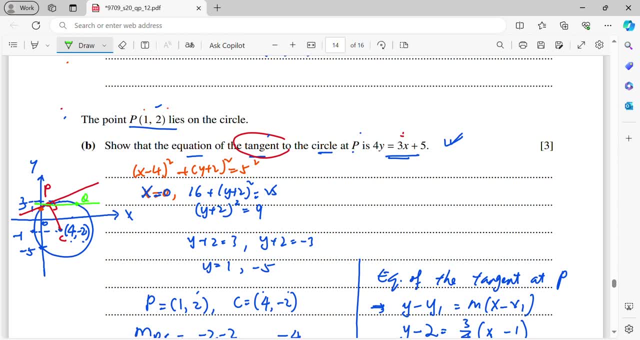 so pq is parallel to x axis means that my q is on the same level. this is my q, so that it is parallel to x axis. my q, so that it is parallel to x axis, so which means my y value will be the same. so y value is: 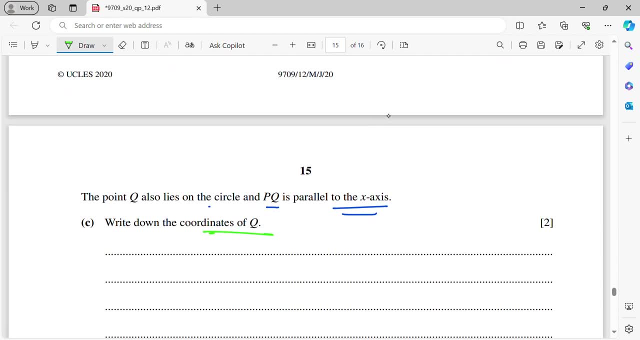 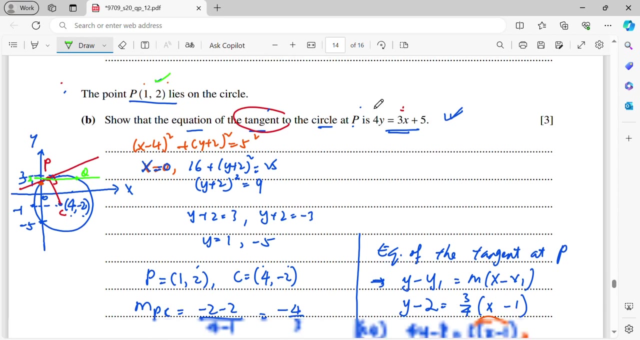 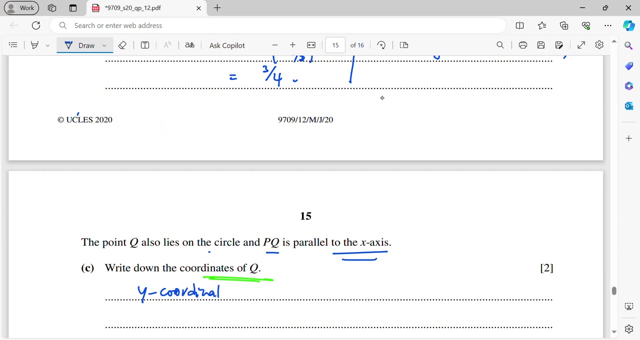 2. okay, so now write down the coordinates of q, all right. so from here i will say: my y coordinates of q is 2, that is what i'm confirmed because the p is 2, right? so the y coordinates of q, y coordinate of q is 2. so now i will substitute y equals to 2 into the circle equation. so i will copy my. 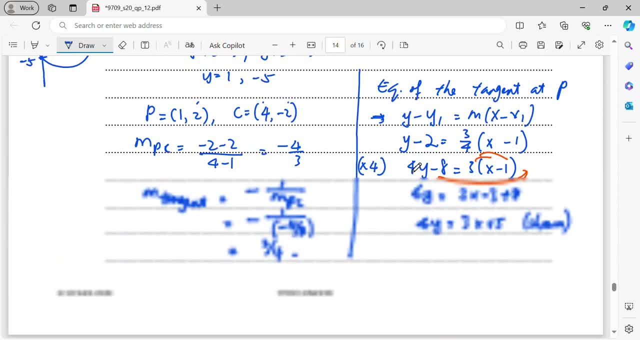 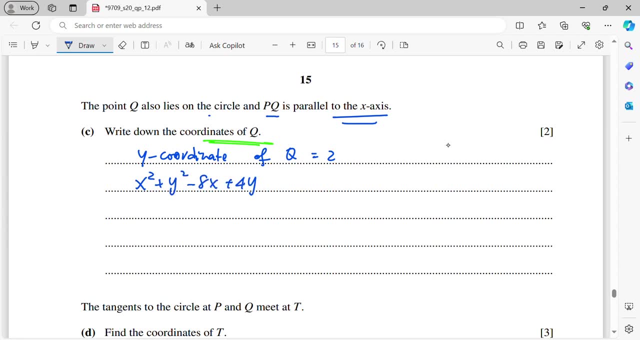 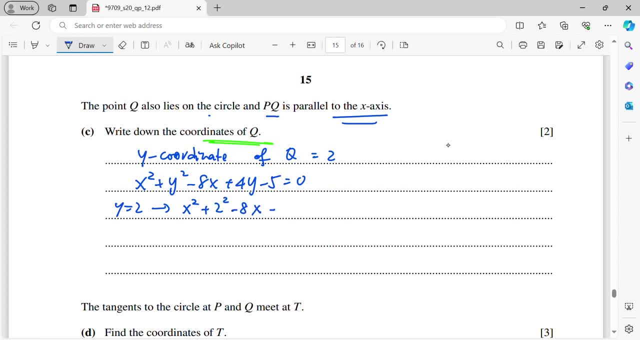 square plus 2, squared minus 8x plus 4 times 2 minus 5 equals to 0. so then x square plus 4 minus 8x plus 8 minus 5 equals to 0. hence you will get x square minus 8x. 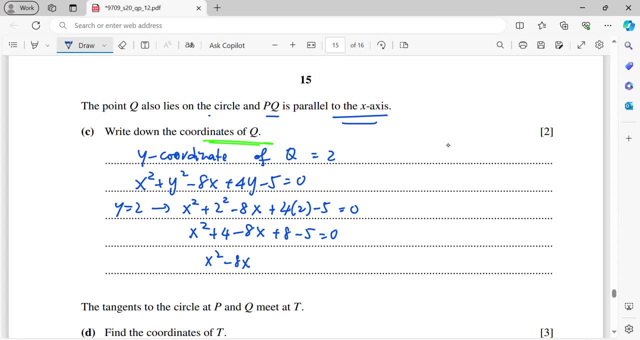 plus 12 minus 7 is basically plus 7. sorry, plus 12 minus 5 is plus 7. then from here this quadratic equation can be factorized. this is going to be x minus 7 and then x minus 1. so here i will get. 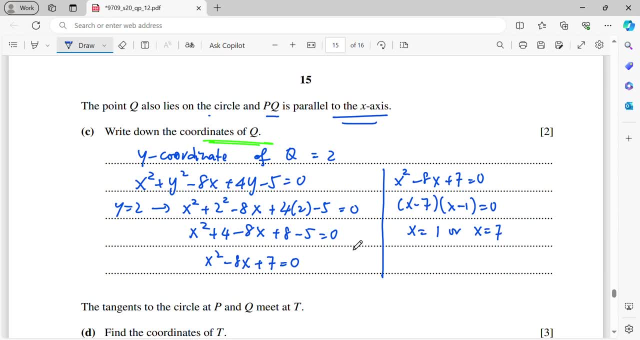 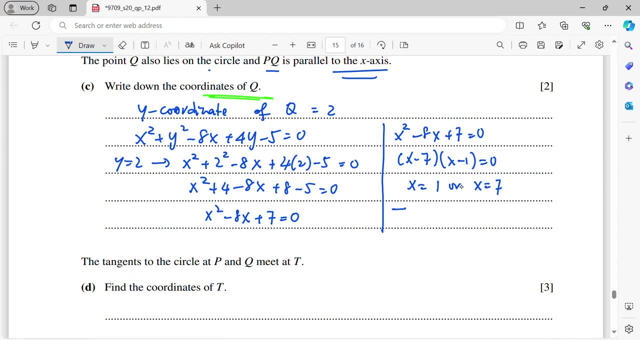 x equals to 1 or x equals to 7. now, when p, x equals to 1, when the x equals to 1, that is basically the points p. so now i know that, okay, at q the x must be 7. therefore my q is, with coordinates, 7: 2. 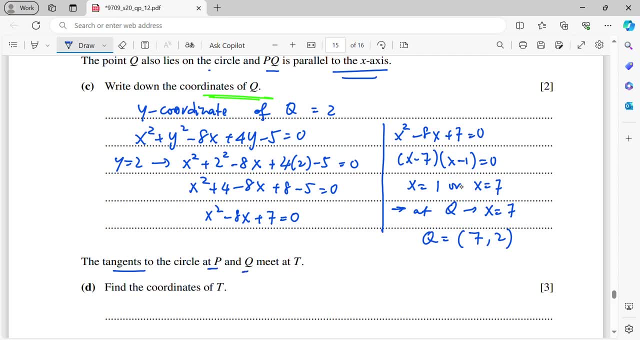 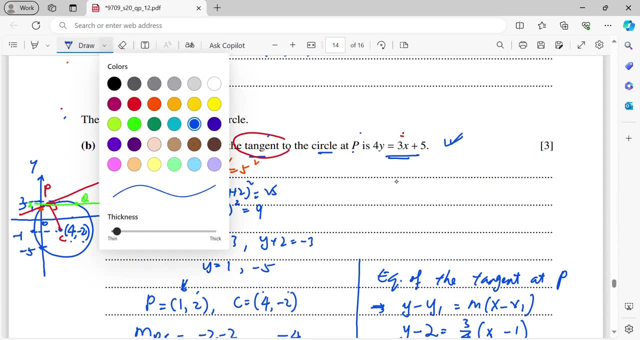 now the tangents to the circle as p and q meet at t. find the coordinates of t. okay, let's say, here i have another tangent, here is the tangent right, this is the t. so now i need to find out what is my gradient. and again, here is 90 degrees, okay. so i need to find out the gradient of qc, then find. 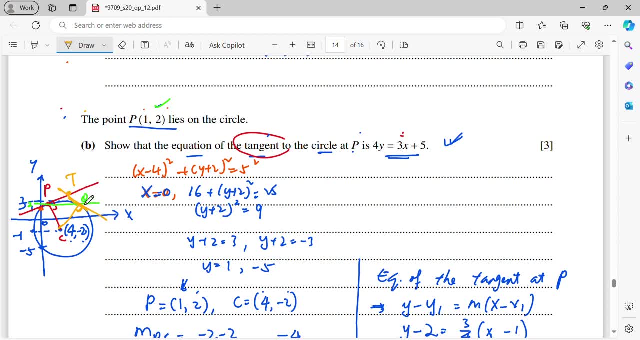 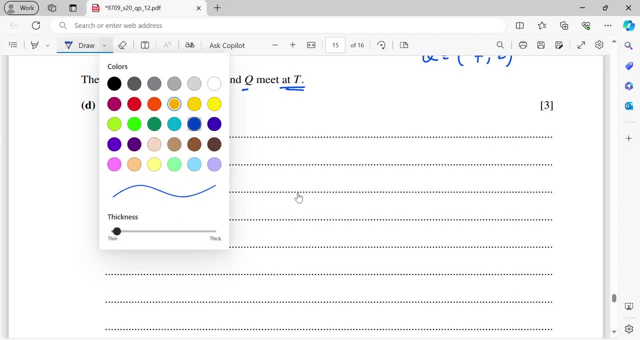 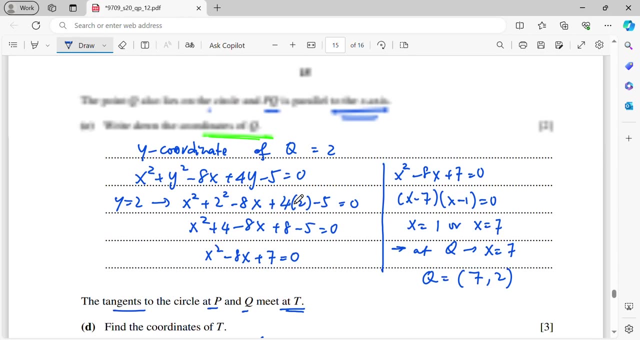 the gradients of the tangent. after that form the tangent line at the q and get the intersection. so now i will write mqc. so my q is 7, 2 and then my c is, with coordinates, 4 negative 2. okay, based on here: 4 negative 2. 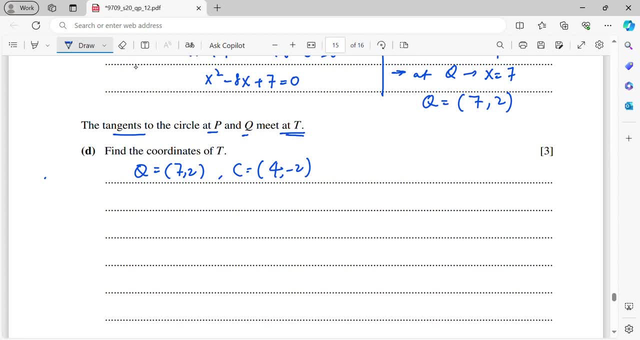 so 4 negative 2. so the gradient of qc is basically change in the x, oh sorry, change in the y. so i will write minus 2 minus 2- i use this first- over 4 minus 7, that is, minus 4 over 3. 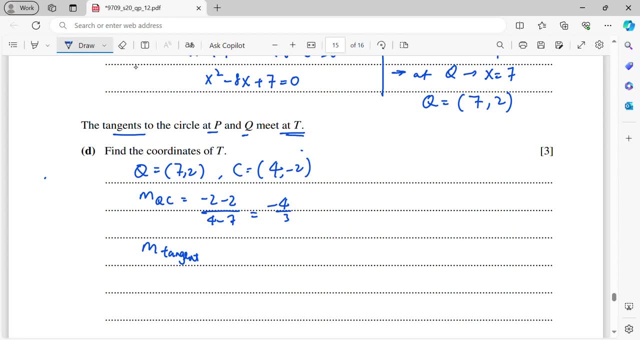 so now m grade, m tangent, it will be negative 1 over mqc because they are perpendicular to each other. so negative 1 over negative, 4 over 3, this is going to be 3 over 4. okay, wait, minus 2 times minus 2, minus 2, minus 4, 4 minus 7 is minus 3. therefore, this is 4 over 3 is a. 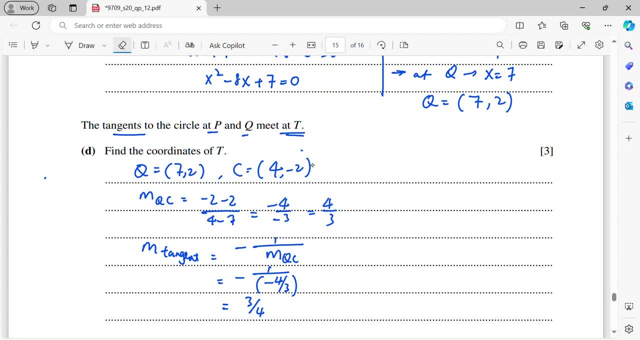 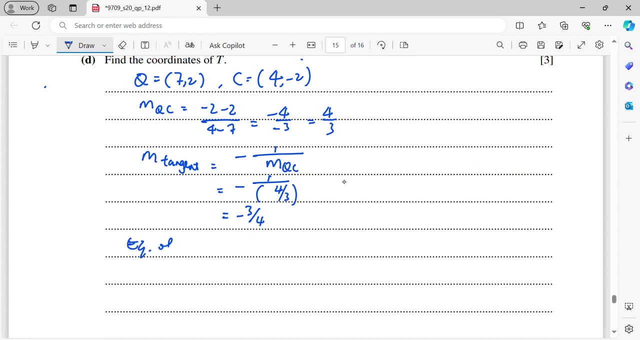 positive. okay mistake, so here is positive. therefore your gradient of tangent is negative. now equation of tangent at q. so that is going to be: y minus y, 1 equals to m, x minus x, 1.. so again now, y minus the q is 7, 2. so 2 equals to the. m is negative, 3 over 4. 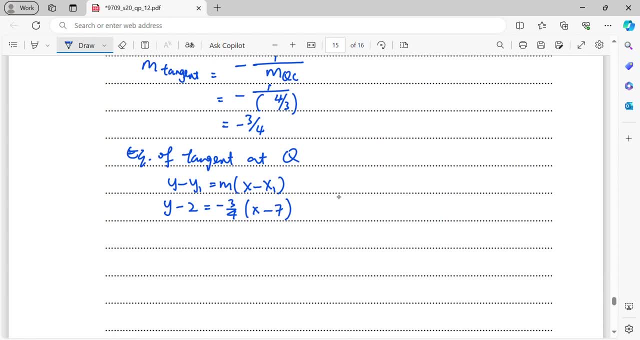 x minus 7. then from here i will get the equation: this is a times four. so when i times four it will be four times one minus two equals to negative three times x minus seven. then here, when i do expansion, four y minus eight, y equals to negative 3x plus 21. at last, my 4y equals to minus 3x plus 21 plus 8.. that is negative 3 plus y minus 7.3.. 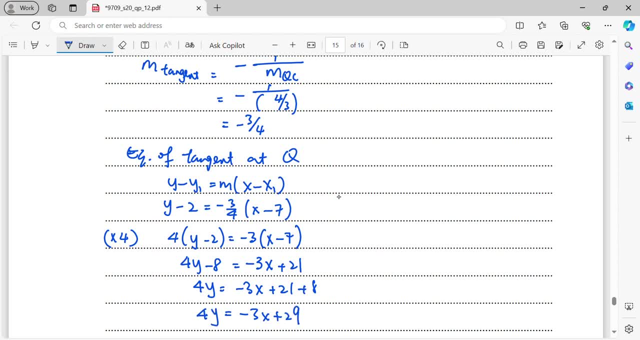 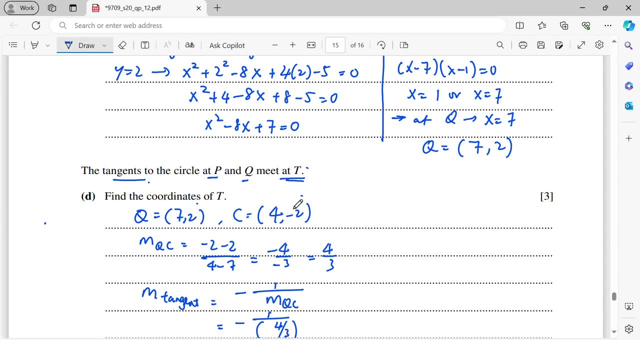 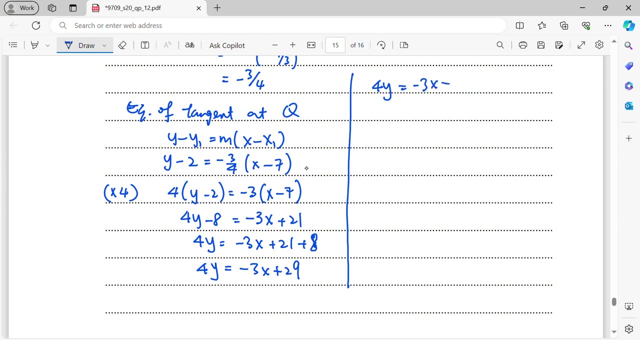 3x plus 29, that is my 4y. so this is the equation of tangent as q. okay then, now it's mentioned that both tangents meet at t, so now I have to solve the simultaneous equations, so I will let 4y equals to minus 3x plus 29 as the first equation. this is the equation of the tangent as q. 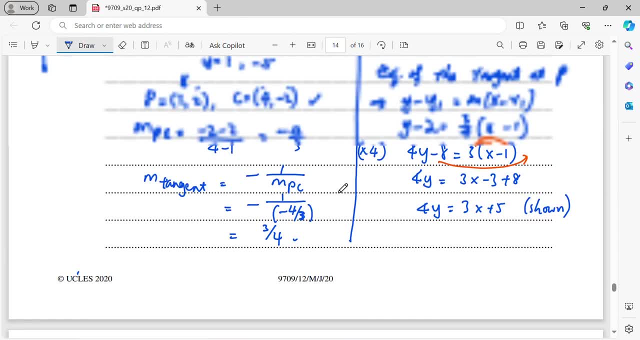 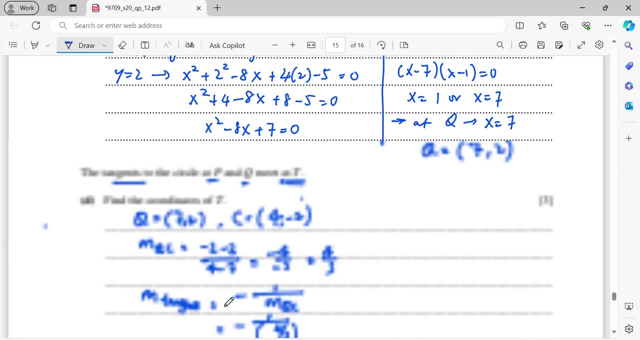 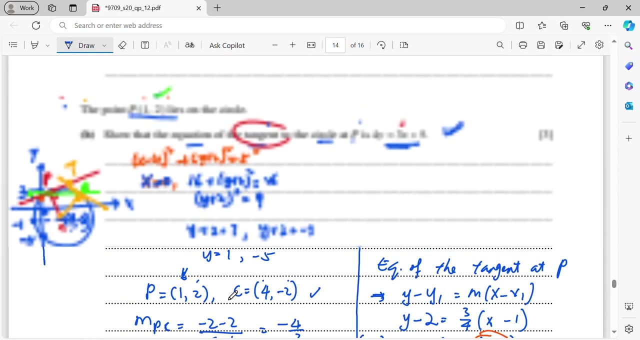 and then the equation of the tangent as p. we get it from the previous part, which is: 4y equals to 3x plus 5. okay, so here I will write: 4y equals to negative. sorry, 4y equals to 3x plus 5. okay, 3x plus. 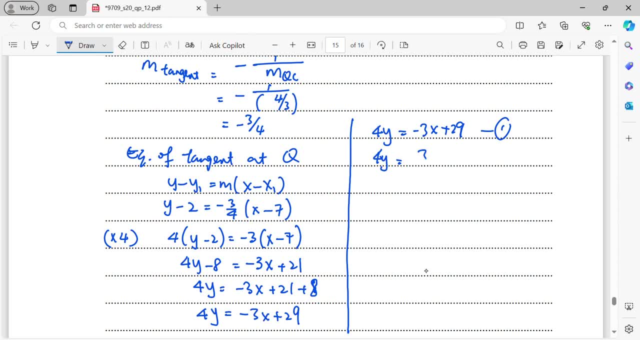 5. this is my second equation, so now to find the intersection points. I will solve these two simultaneous equations, since both also 4y, so I will just use second equation minus first equation. so left side is 0, right hand side 3x. minus minus 3x it will be 6x. sorry, positive 6x.